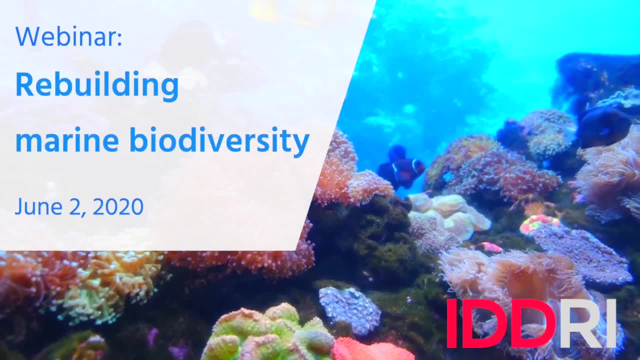 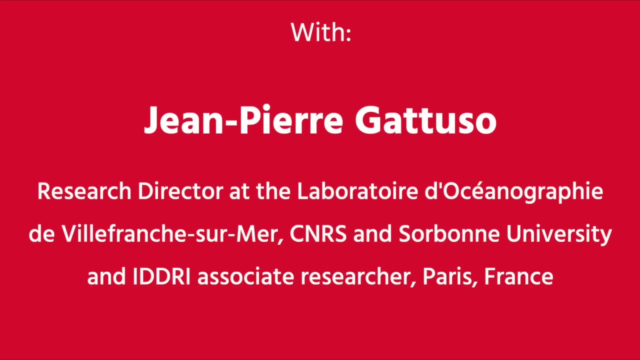 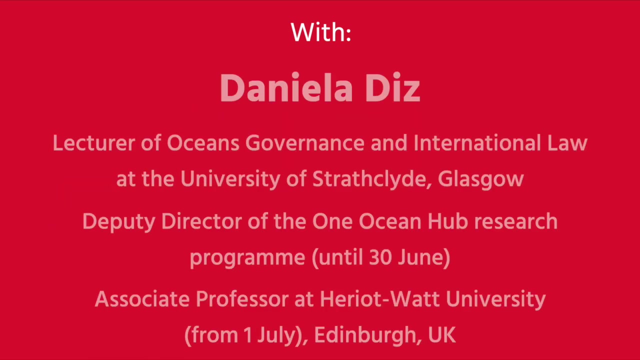 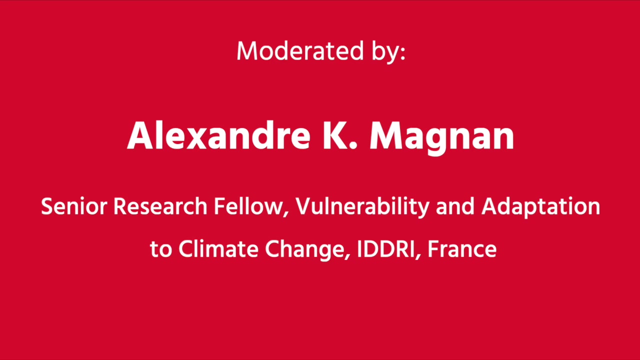 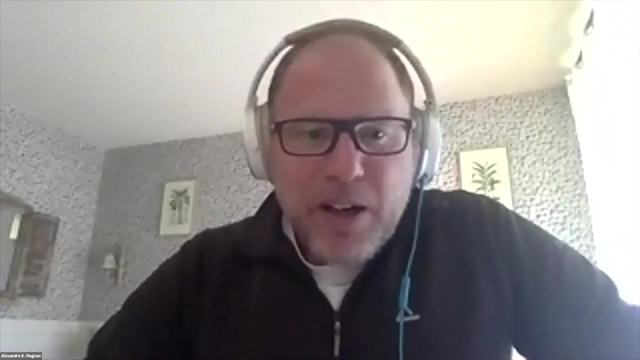 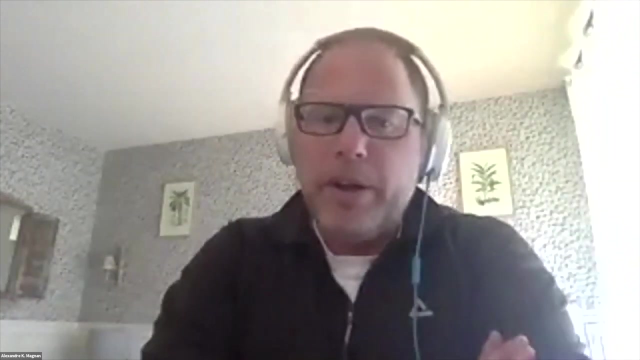 Learn French through audiobasics at Léves-Françoiscom. Learn French through audiobasics at Léves-Françoiscom. So welcome everybody to this IDRI webinar. We are together for about one hour and a half to discuss some interesting perspectives. 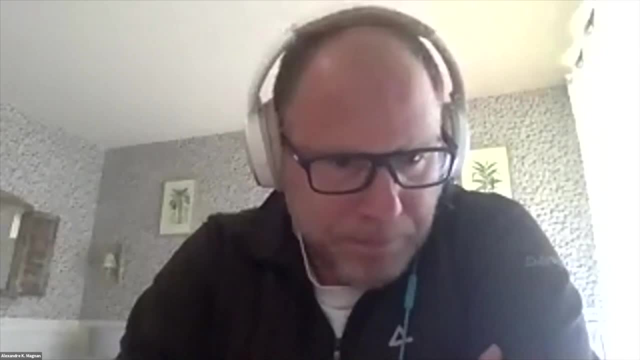 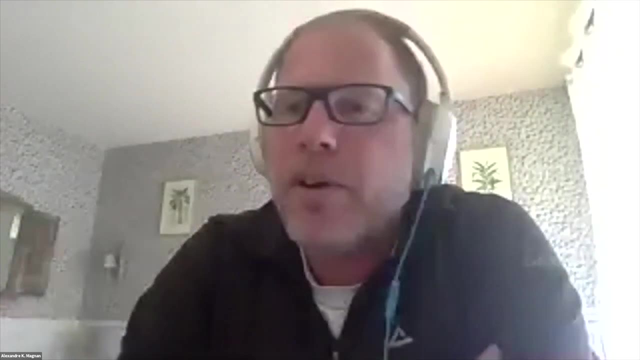 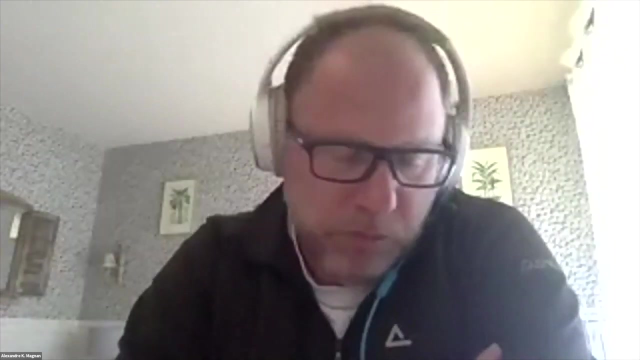 on rebuilding marine life. So, as you all know, talking about the threats to marine life is wider than asking ourselves how to save just fishes or coral reefs or other species. It's more profound. It's really about understanding the risks. It's more profound. 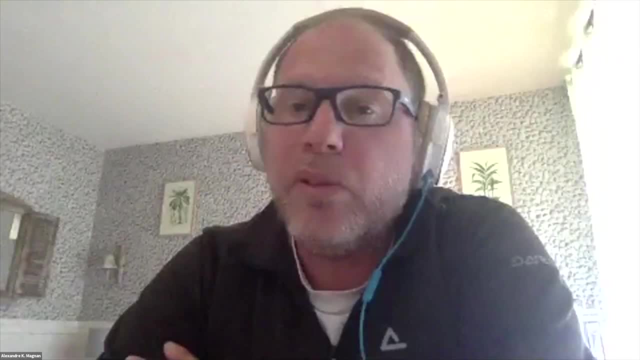 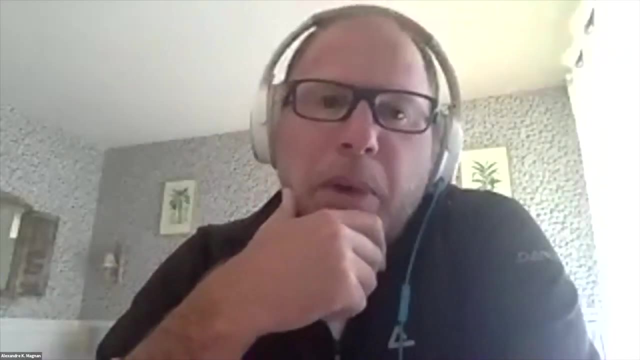 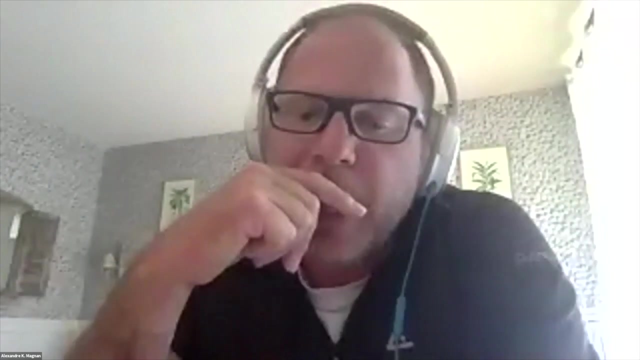 It's really about understanding the risks. It's really about understanding the risks posed to the good functioning of the whole ocean system And, if we go a step further, it's about understanding first an important piece of the climate system puzzle- the ocean- and as well about understanding the risks to ecosystem services that are for 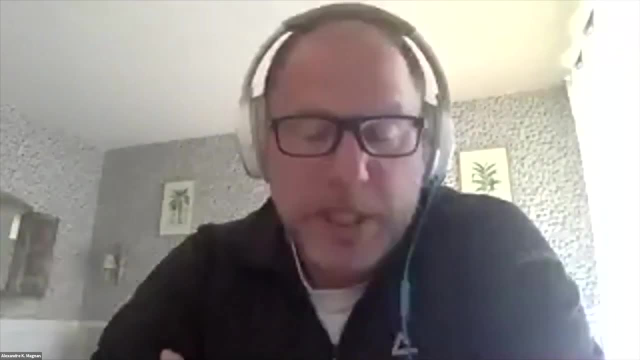 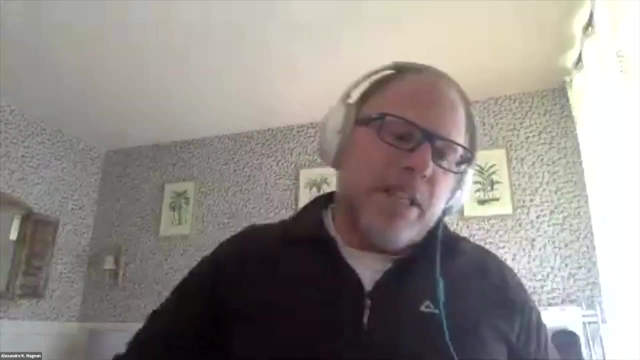 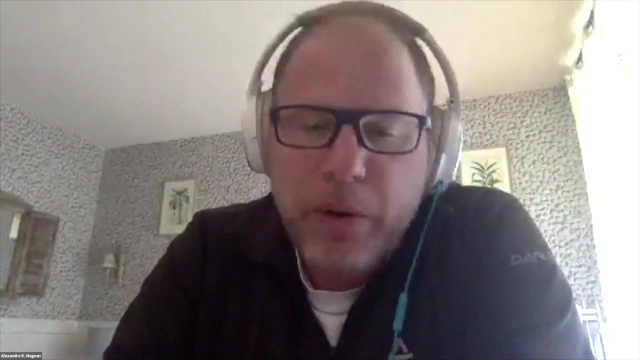 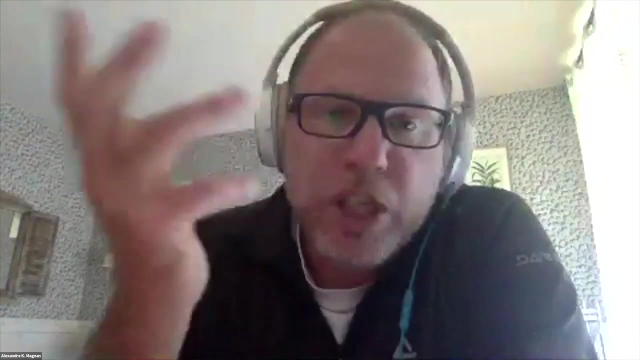 many people around the world absolutely critical, if you think about food security Or coastal protection, for example. And what science shows is that many drivers of depletion often risk to marine life- are converging since the second half of the 21st century through fishing and habitat destruction. 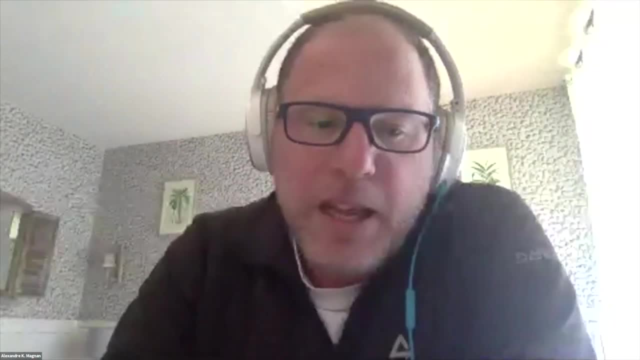 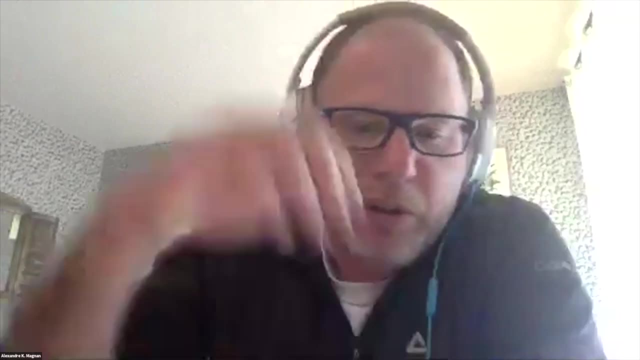 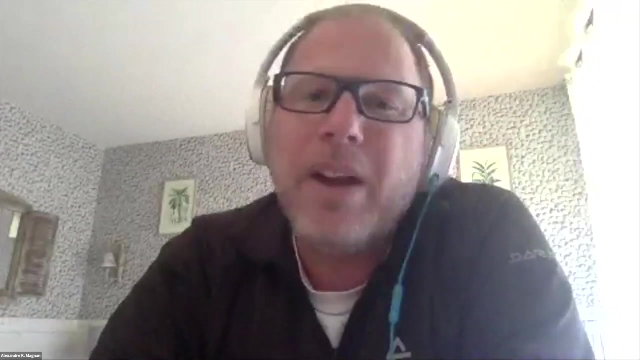 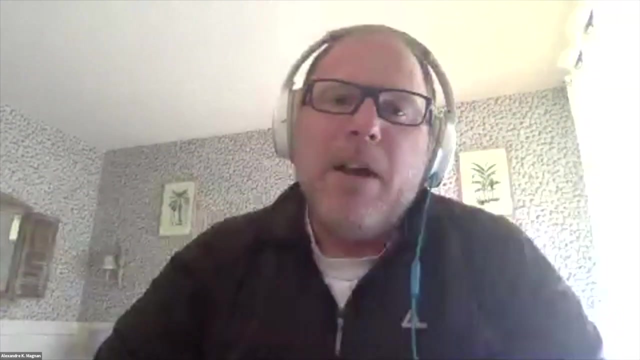 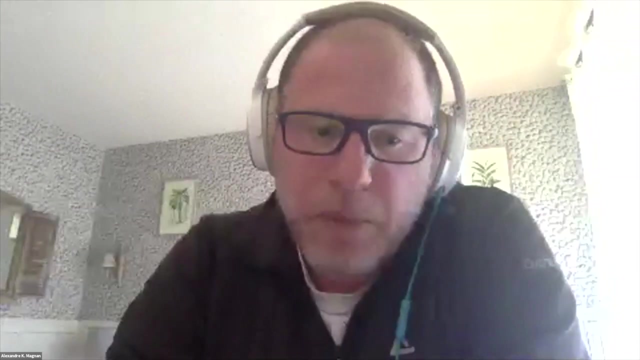 for example, and now including climate change And the recent IPCC special reports on 1.5 degree on land and on ocean and climate. but to the friend of conveying the Waase, наш lange, science is clearly highlighting that climate impacts on the ocean and coast are already. 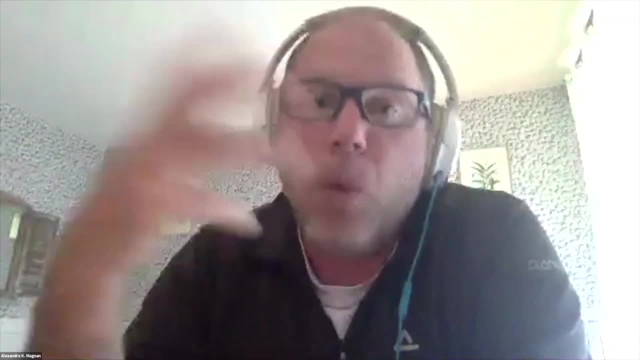 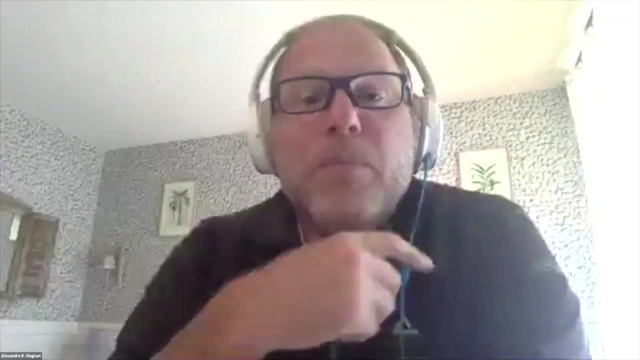 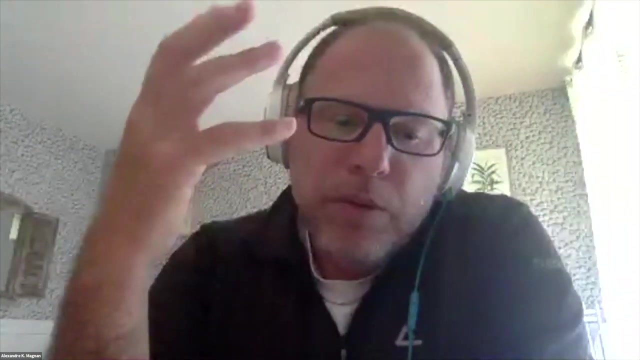 detectable and at all latitudes and at all depth, And these impacts will likely become more severe in the decades to come. So the problem is serious. okay, The future risk will not only depend on climate change, for example, or external drivers. 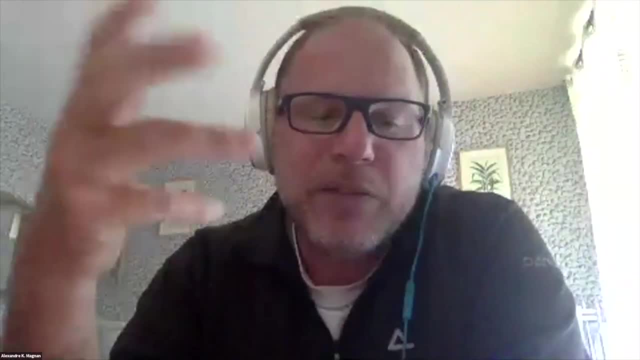 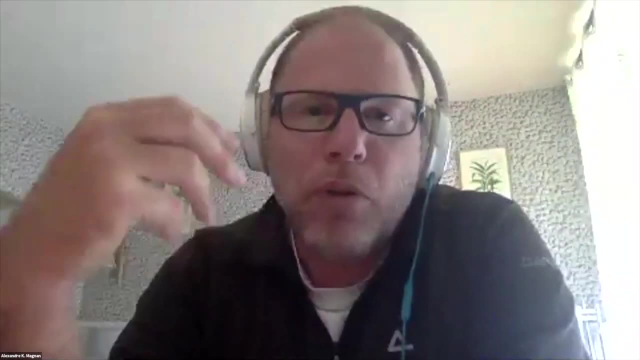 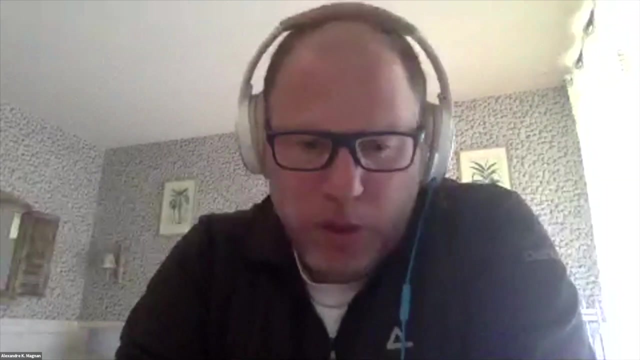 The risk will also partly depend on how effective what we will globally and locally put in place now, how much it will be effective on the long run, And this is a critical question, And a recent paper published in last April in Nature brings some encouraging and insightful messages. 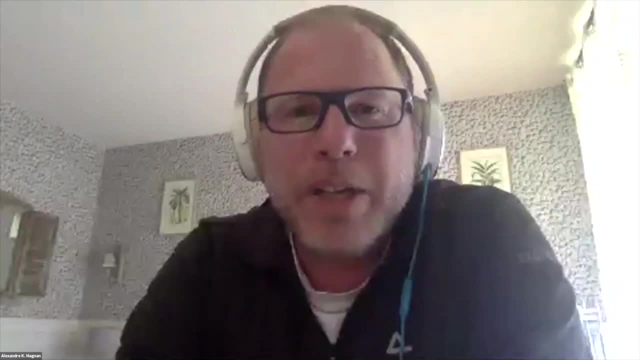 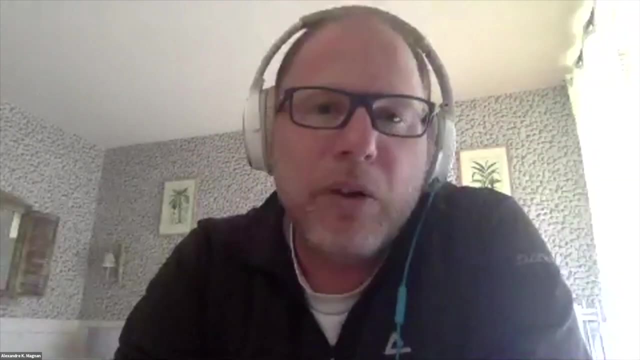 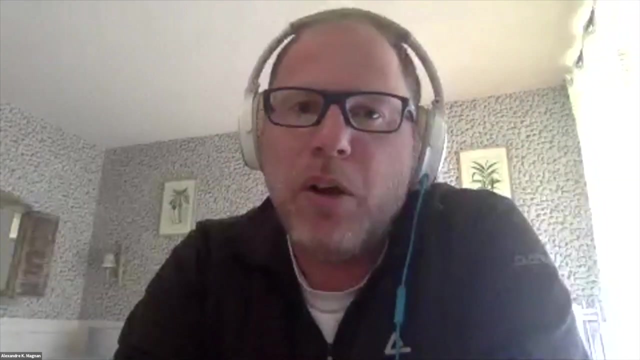 And that's good, in this period of troubles, to hear about some positive messages. This paper basically shows that, depending on various conditions, scaling up human-driven conservation efforts could help substantial recovery of marine life within a generation, that is, by the mid-century. 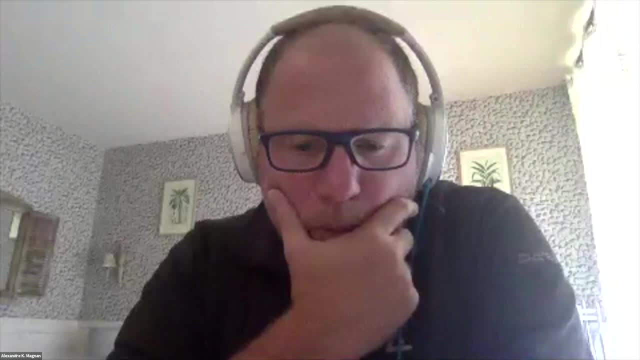 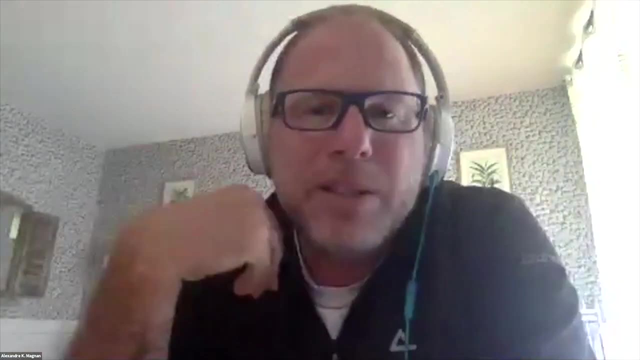 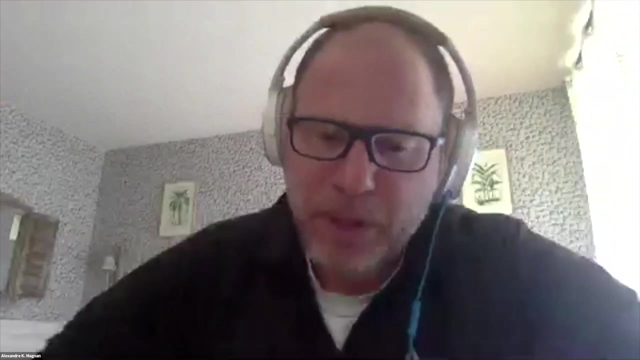 And that's an important message for many species, for the ocean as a whole, but for the planetary system as a whole and for humankind at large. To discuss this, Idri welcomes three speakers today: Jean-Pierre Guettier, who is research director at the. 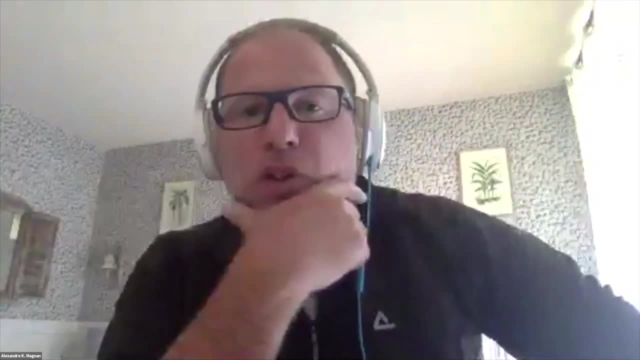 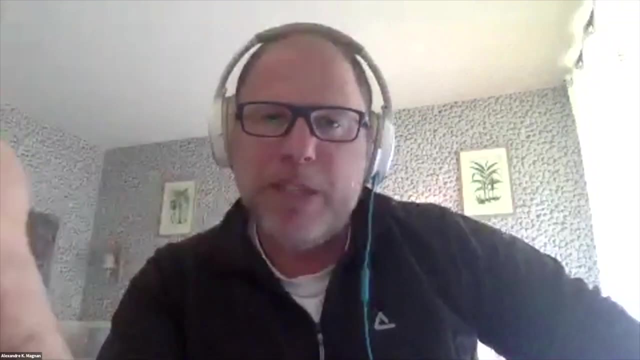 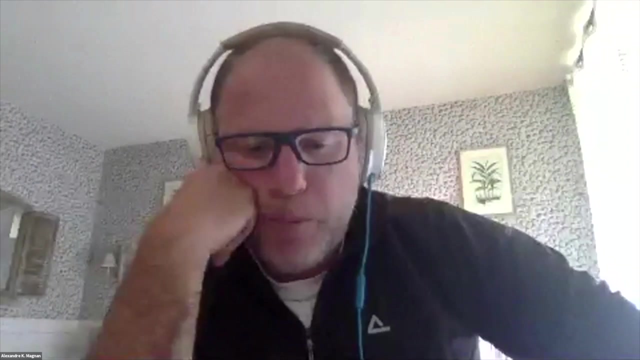 Laboratoire d'Océanographie de Villefranche-sur-Mer. It is a laboratory of the CNRS and Sorbonne University in France, so based in France, And he is also Idri's associate researcher. He co-authored the Nature publication. 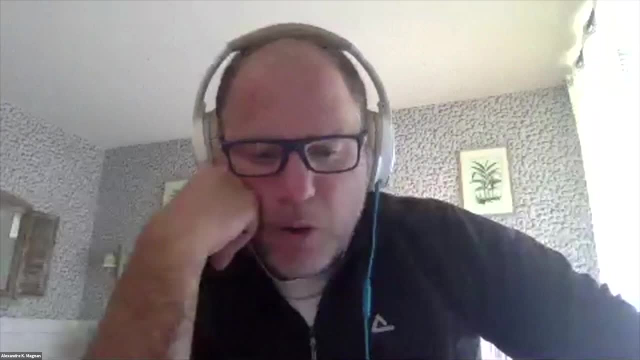 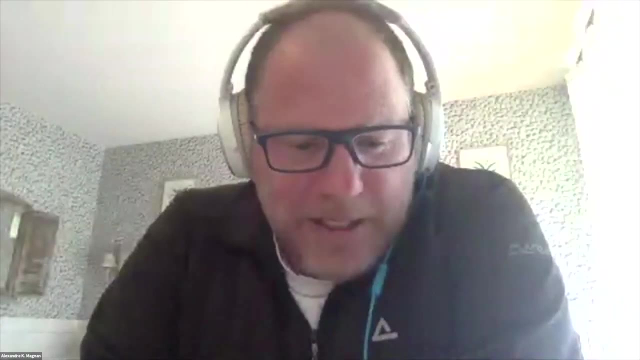 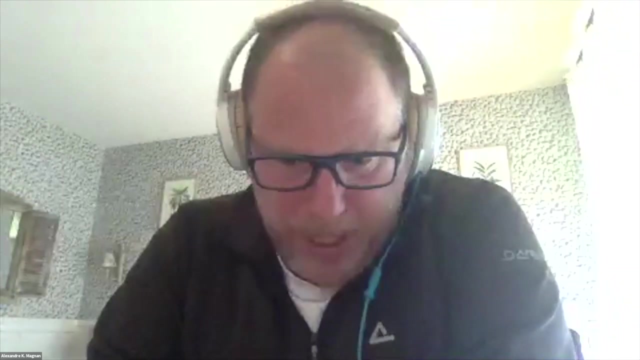 Second, we also have Nancy Nancy Nolton. She also co-authored the Nature publication. She is a coral reef biologist And is the Smithsonian Institute's SENT chair for marine science, And she's based this morning in the US- this morning for her. 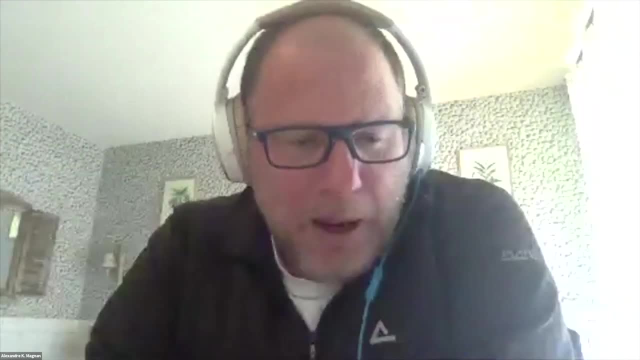 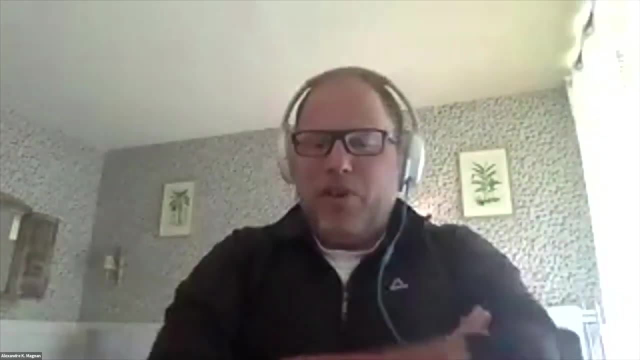 I've done it for Europe. And last but not least, of course, Daniela Gies. She is joining from UK. She is lecturer of oceans, covenants and international law at the University of Strathclyde in Glasgow. 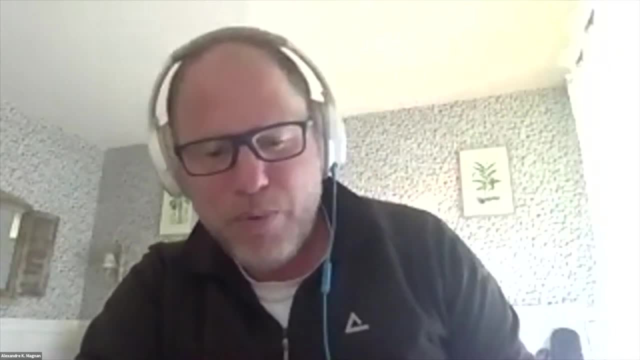 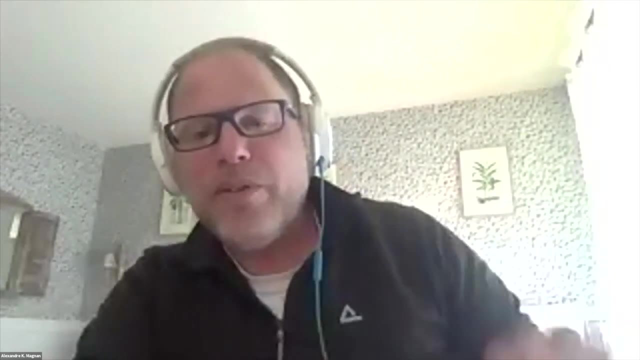 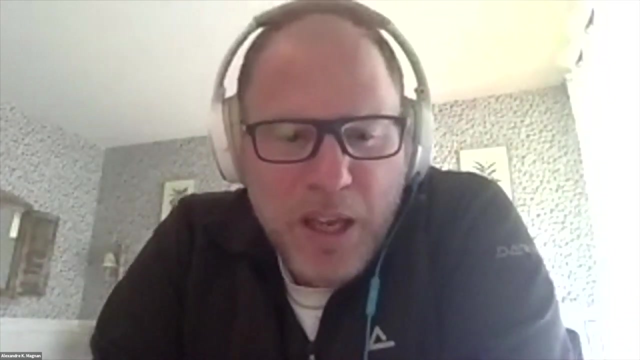 She is also director of the Deputy Director of the One Ocean Hub Research Programme And in a few weeks from now she will join the Eriot-Watt University in Edinburgh, still in UK. Briefly, Jean-Pierre will present the main conclusions. 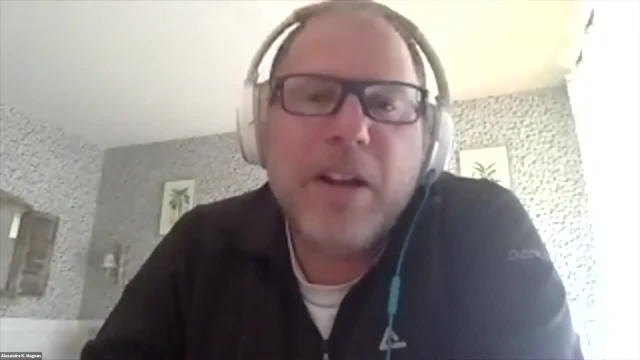 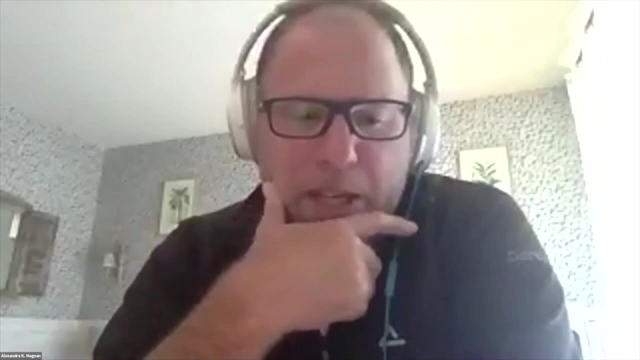 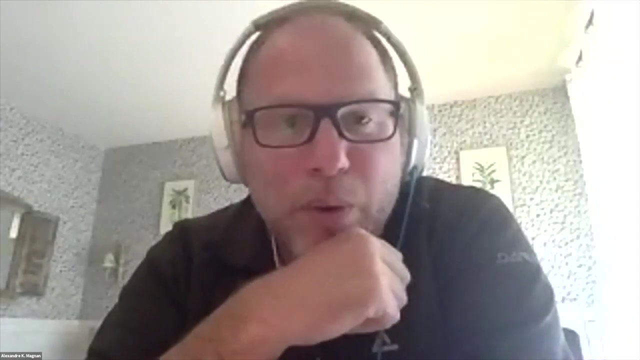 of the Nature paper, as well as some insights on the panel of ocean-based solutions that can help support rebuilding marine life and, more broadly, to help address climate change. And it's it, And Nancy will take us for visits of the world of coral reefs for more specific insights. 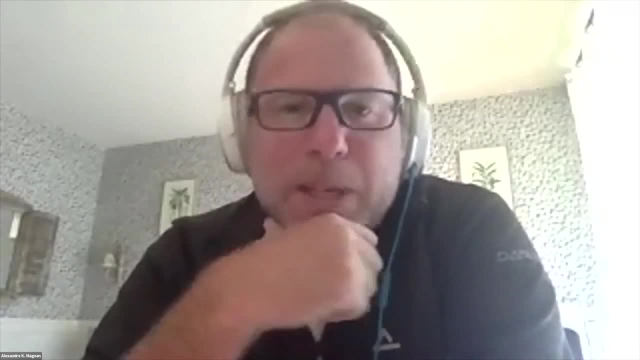 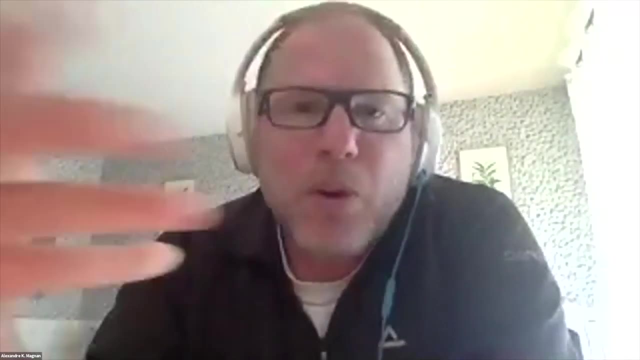 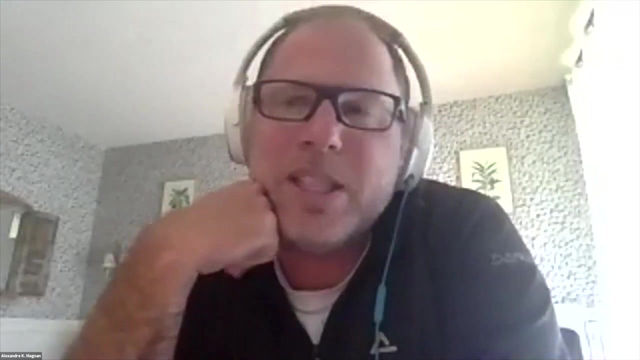 and interesting things. because we know coral reefs are the frontline of climate- climate change, sorry. And so the question is: what can we do for them? Because if we can do something for coral reefs and if the benefits to be expected are interesting, 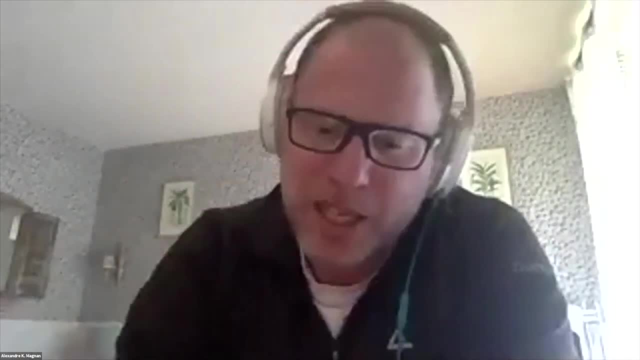 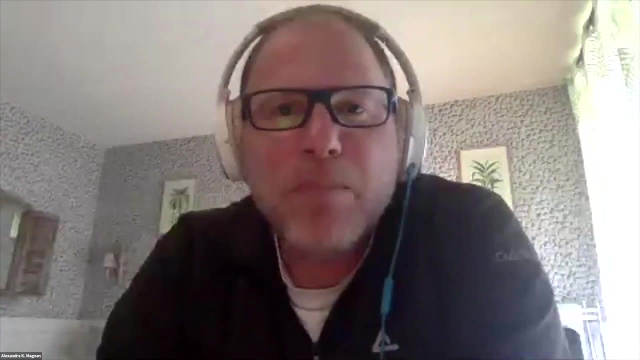 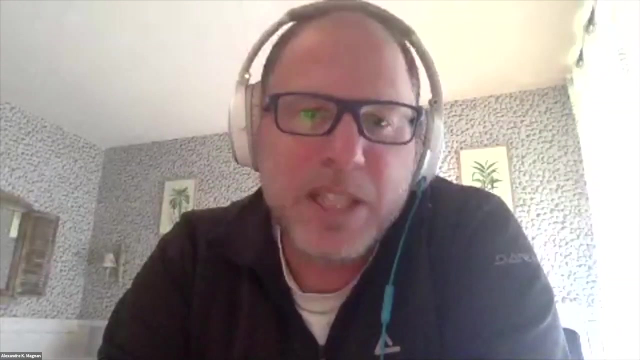 then this is a positive signal for other species In the ocean, but maybe not only in the ocean. And then Daniela will help us understand how to move from scientific solutions to policy action. And the question is what kind of governance frames can help rebuilding marine life and what challenge they face. 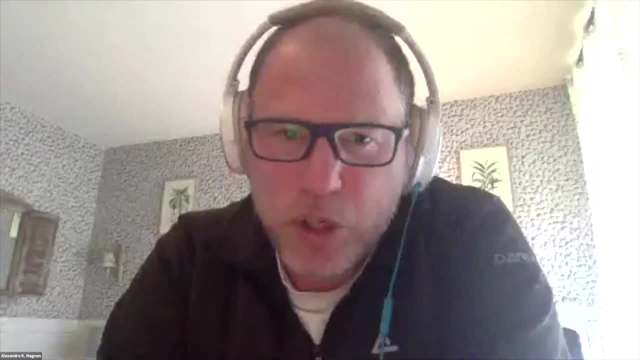 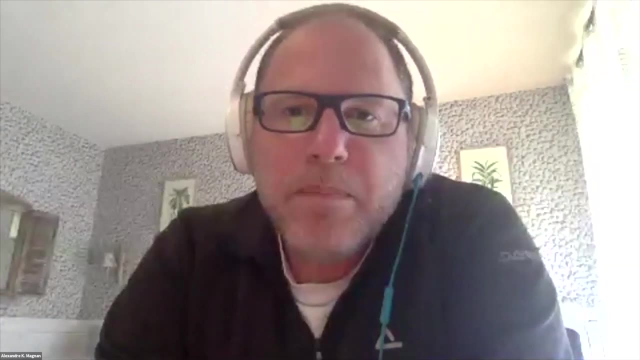 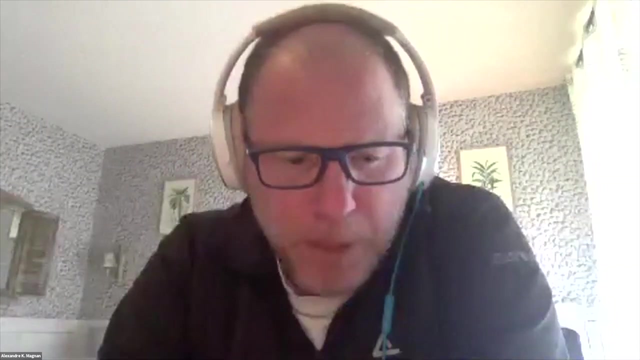 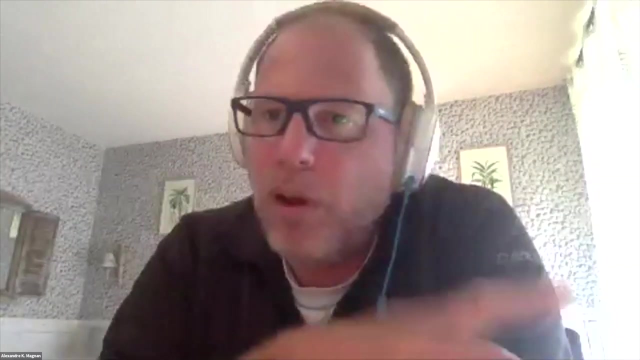 So I stop here. I will give the floor to Jean-Pierre in a couple of seconds, Just before a brief technical points. you are now about 150 people online. The three presentation will ask for about an hour and then we will have a 30 minute question and answer session. 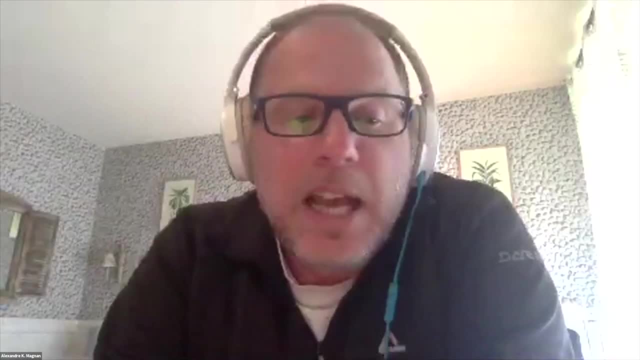 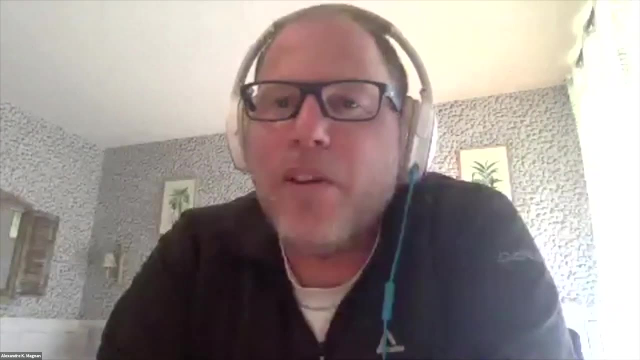 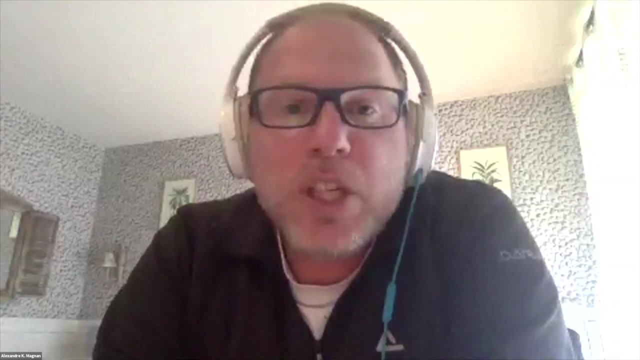 But all along the presentations you can ask questions by using your Q&A button. at the bottom right of your screen, I think there is a small button Q&A. You can post your question and my colleagues Pierre Barthélemy and Karine Antunes will help me select. 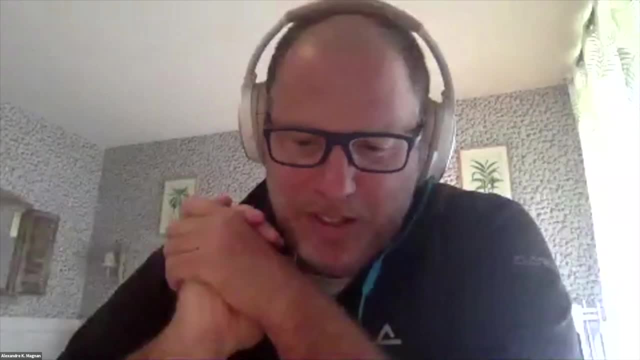 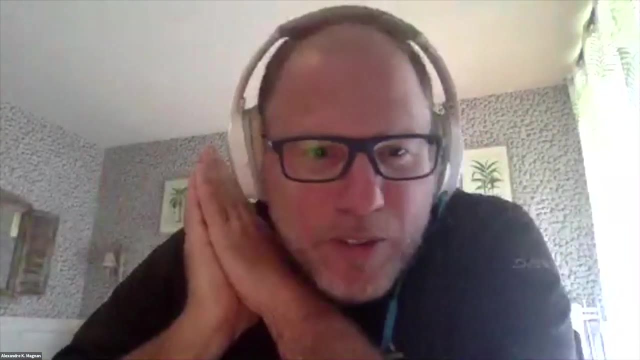 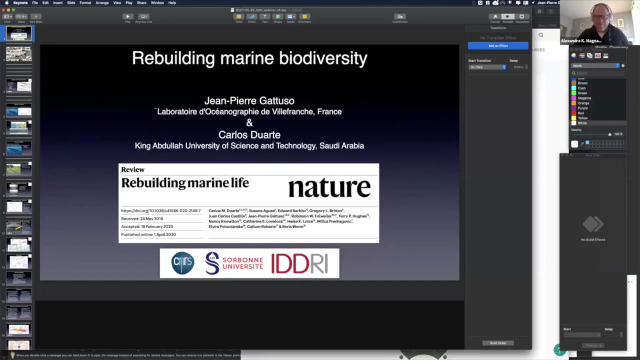 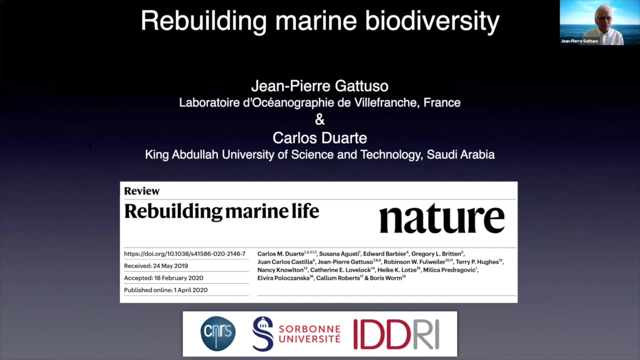 a bunch of questions to ask to our speakers. So, Jean-Pierre, you are the surface of the sea. I see that, So the floor is yours, Jean-Pierre. Hello everyone, Let me start this. So I'm going to today to let you know about this paper. 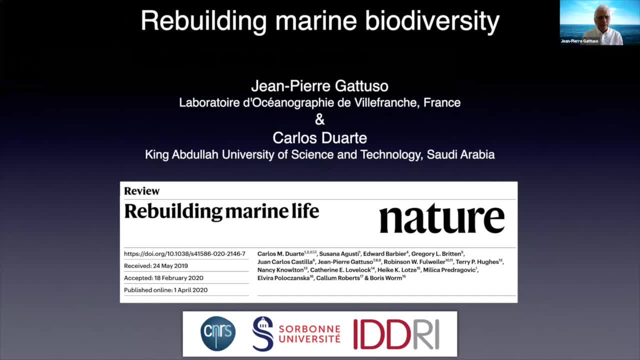 which was led by Carlos Duarte, who, I want to acknowledge, is my co-author on this presentation: rebuilding marine biodiversity. So, together with 15, in total 15- colleagues looked at the potential to rebuild marine life and I will provide in the next 20 minutes a brief overview of that. 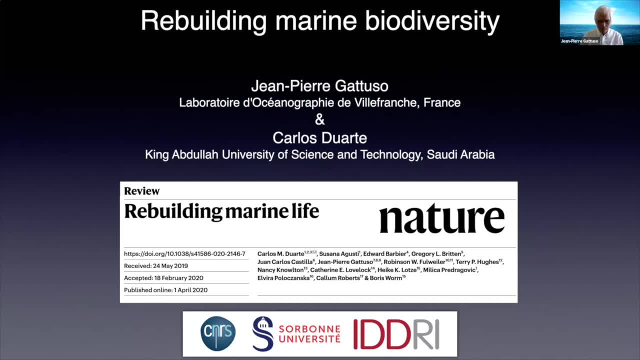 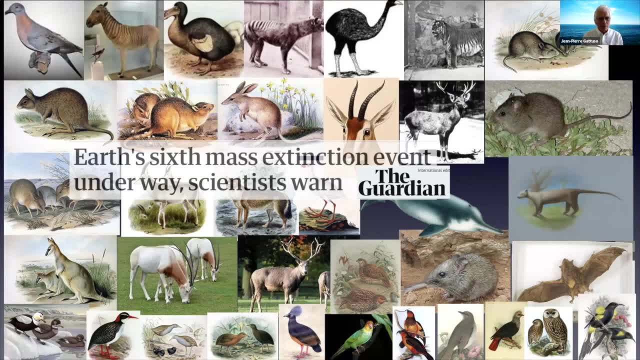 and Nancy Knowlton will specifically discuss coral reefs. So, as you know, there is a lot of worries about the loss of biodiversity, and, especially recently, the report of the International Science Policy Platform on Biodiversity and Ecosystem Services, IPBS, highlights the fact of this erosion of biodiversity. 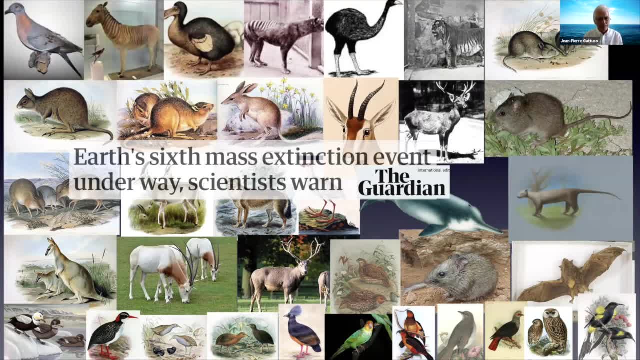 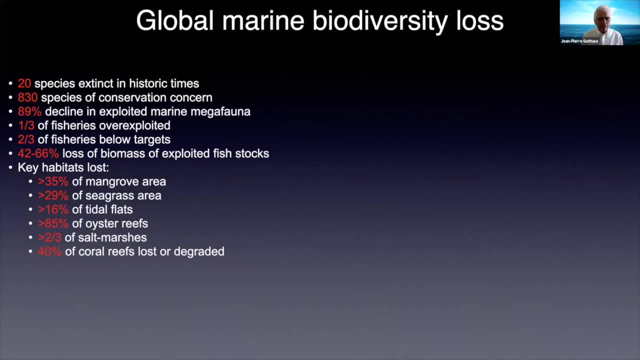 and, of course, the mass media took this on board and there are some projections of the Earth going through its sixth mass, which is a very large extension event. So, and indeed the loss is quite stunning In terms of species: 20 marine species are now extinct. 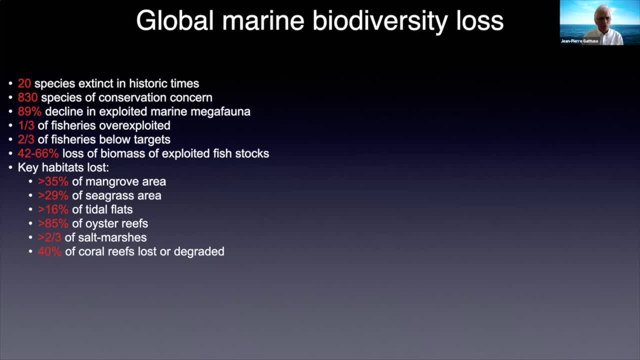 More than 800 are under conservation concern by the IUCN, the International Union for Conservation of Nature. Almost 90% of the marine megafauna which is exploited is lost. Almost 90% of the marine megafauna which is exploited. 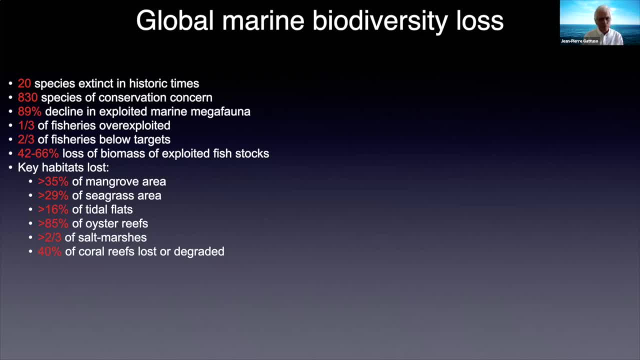 has declined. One third of fisheries are overexploited. Two thirds of fisheries are below the targets of sustainable use, sustainable fishing. And also- let me go back- A number of key habitats have been lost in terms of mangroves, seagrass, tidal flats, oyster reefs, salt marshes and coral reefs. 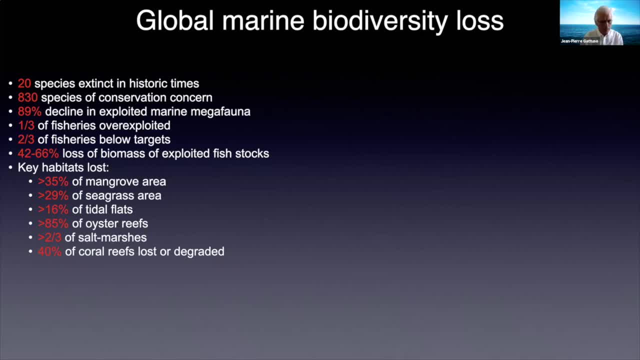 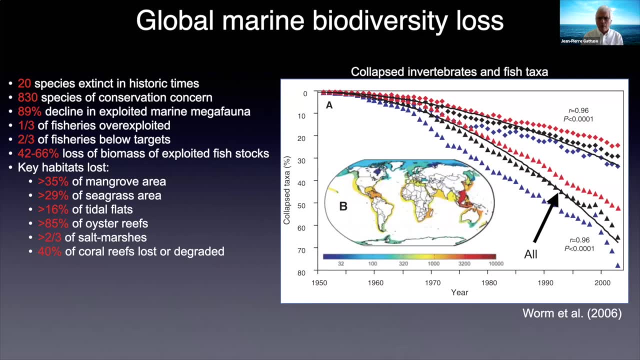 which again will be discussed by Nancy in a few minutes, And a colleague of us looked at the collapsed Endlertagration fish taxa and the black line here represents all of the taxa he looked at and indeed the decline is quite significant. 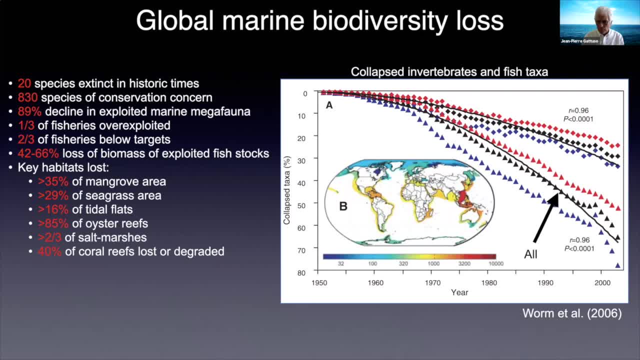 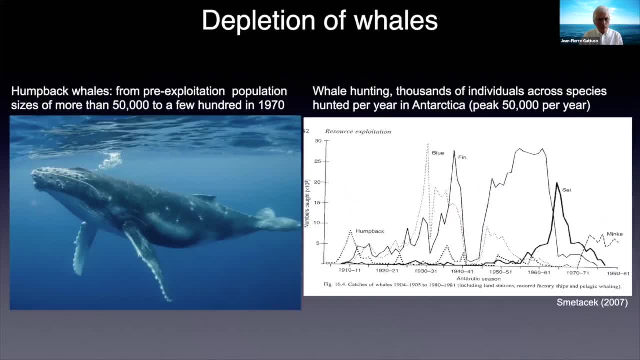 So this is why this paper is quite dramatic, this paper by Ivo Metalin, also a co-author on this paper I am discussing. So the depletion goes from top mammals. so the depletion goes from top mammals, the biggest, the largest mammals here in Unpacked Wells. 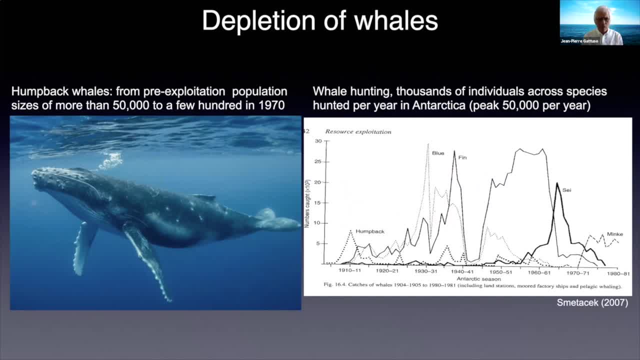 which went from 15,000 individuals before they were exploited, which went from 15,000 individuals before they were exploited, which went from 15,000 individuals before they were exploited to a few hundred in the early 70s. And on the right here, the exploitation. 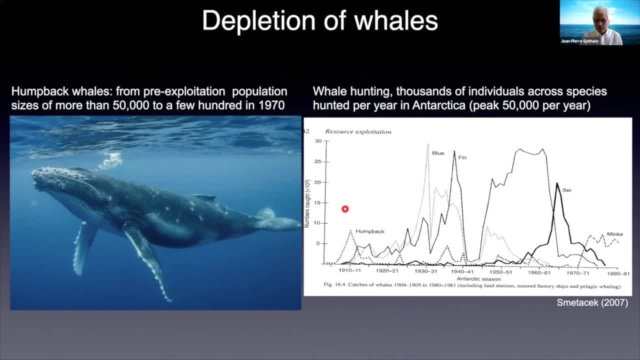 of various species of whale in Antarctica which, when one- the first one- got extinct or largely depleted, then another one was exploited, and then another one, another one, et cetera. So the loss of marine mammals has been quite dramatic. 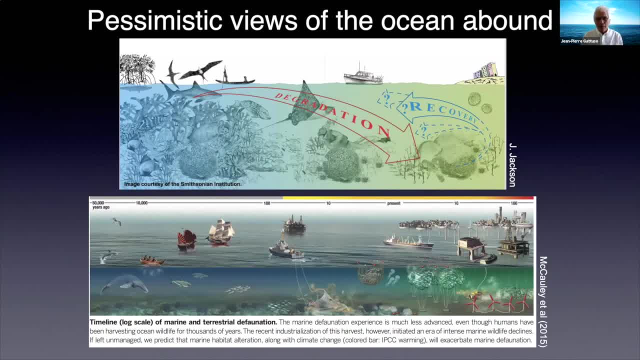 And indeed the pessimistic views are plentiful about the loss and the degradation of the ocean. Here on the top, a cartoon put together by Jeremy Jackson to illustrate his PNAS paper a few years ago, which shows the the large degradation and with recovery here: 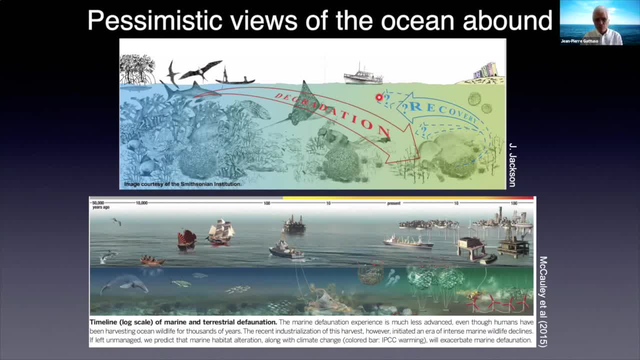 with the question mark: will ecosystems and species be able to bounce back? And at the bottom, a cartoon by Mac Collier showing the increased use of the ocean. on top, and the decline and defonation, as they call it, the defonation, the progressive defonation of mammals. 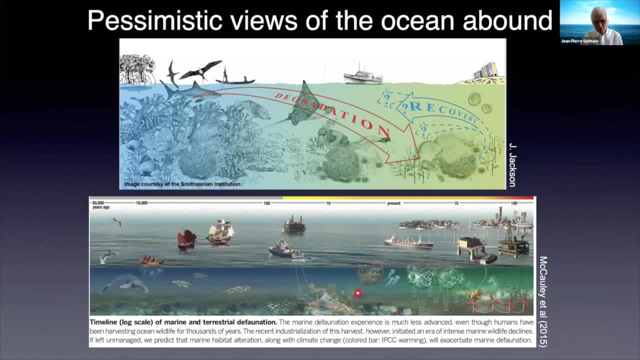 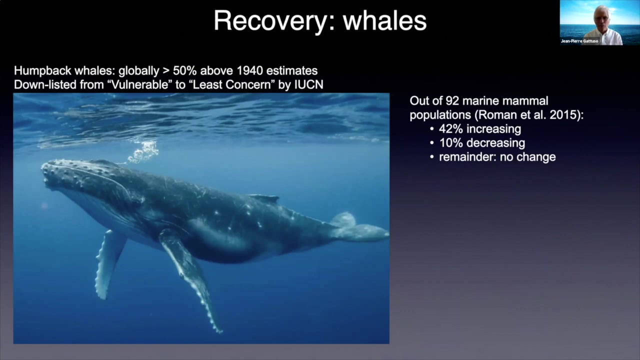 and big fish, smaller fish, large scale fisheries and the development of aquaculture and an ocean dominated by jellyfish. So very pessimistic view. So in this review we looked at the recovery, the documented recovery in the scientific literature. 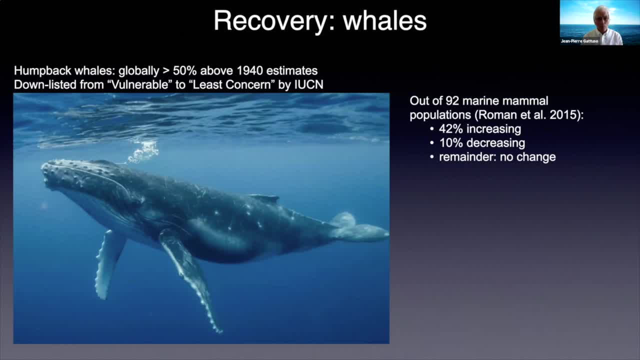 So for the humpback whales: globally, their population is more than 50% above the population estimated in 1940. And in fact these whales have been non-listed by the UCN from vulnerable to least concern in terms of conservation. 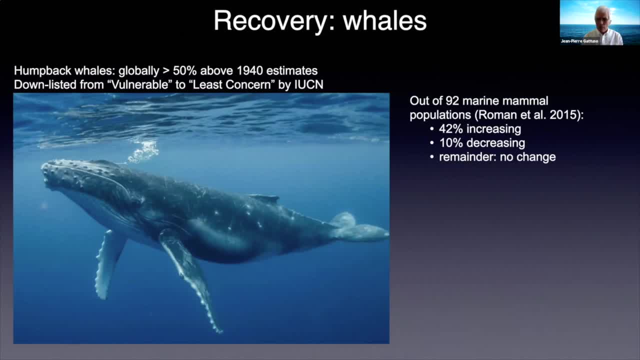 And globally, out of 19 marine mammal populations which are well documented, 42 are increasing, 10% are decreasing and the reminder is showing no change. So the recovery of whales seems to be underway, of course, largely because of the change in the environment. 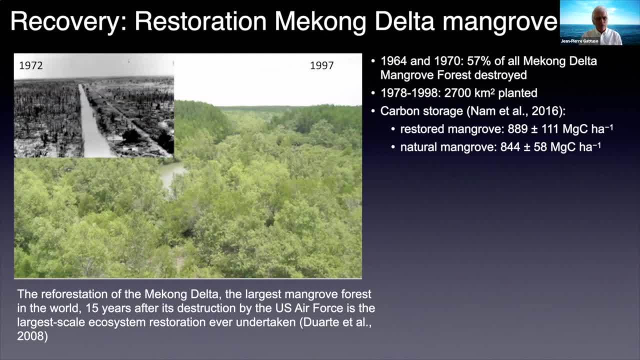 management and regulations. another spectacular recovery is the restoration of mangroves in the Mekong Delta in Vietnam. this mangrove forest, the largest forest in the world, was largely destroyed during the Vietnam War due to the use of herbicides by the US Air Force and, starting in 1978, there is 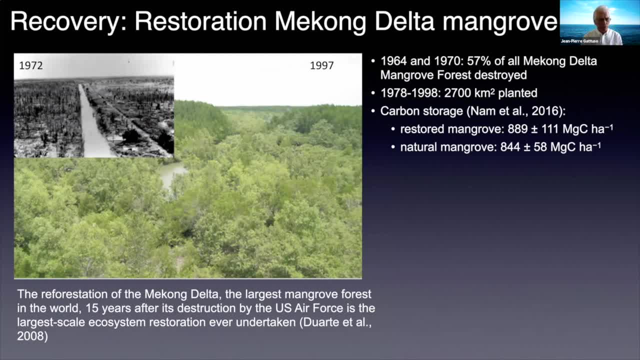 there has been a very large restoration effort, which in fact is quite astounding, and it was shown recently that those mangroves- one of their benefits is that they store carbon and can contribute to the mitigation of climate change. their carbon content in in the best store mangrove is about the same as the one 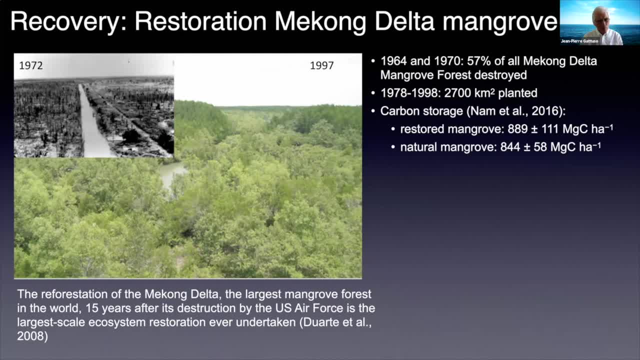 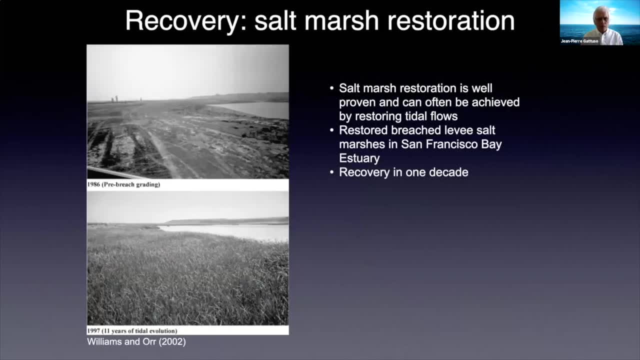 that the carbon content in natural mangroves, so they continue to provide this carbon storage service. similarly, salt marsh restoration is well proven and and has been very well described here. an example: in the San Francisco Bay estuary, where in in just one decade, this salt marsh was largely restored, as documented by William et al in 2019. 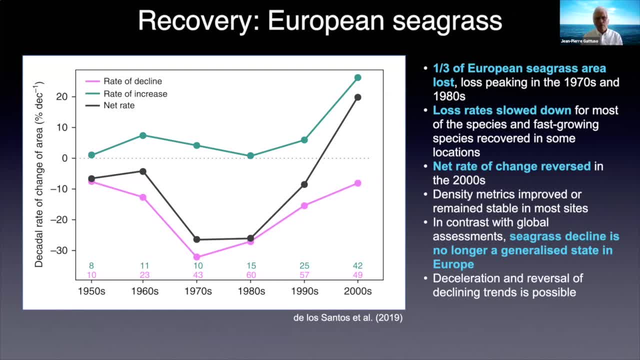 a spectacular recovery of European seagrass. this recent paper looked at the population locations of seagrass extent and they show that one-third of European seagrass has been lost, especially in the 70s and 80s, and among the locations they were divided into, the green ones. 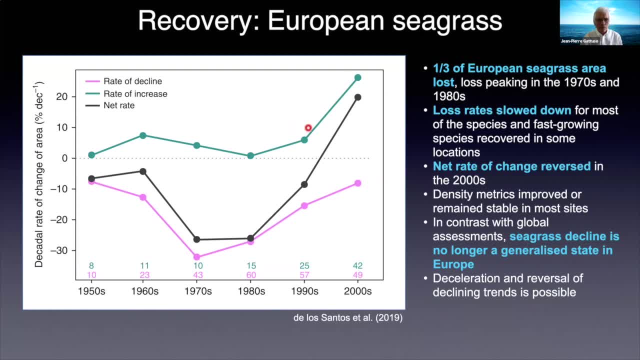 where seagrass surface. the surface area of seagrass is increasing and the ink here where it is decreasing, and the black line here is the, the net change in the extent of seagrass, and you see that in the 2000s the rate of change has. 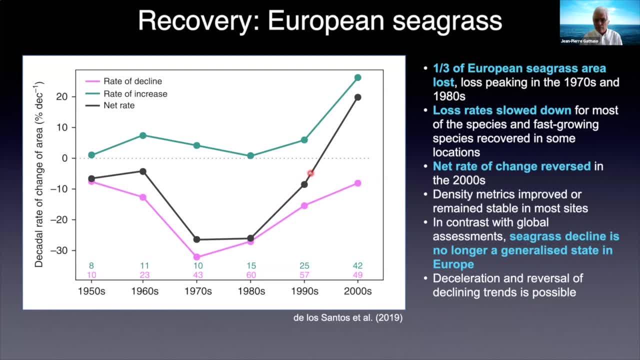 has gone from negative to positive, showing that, in fact, nowadays the seagrass decline is no longer generalized State in Europe. demonstrating, and in fact it has been observed in other locations, not so many, but in in Florida, in Japan and some locations in Southeast Asia. 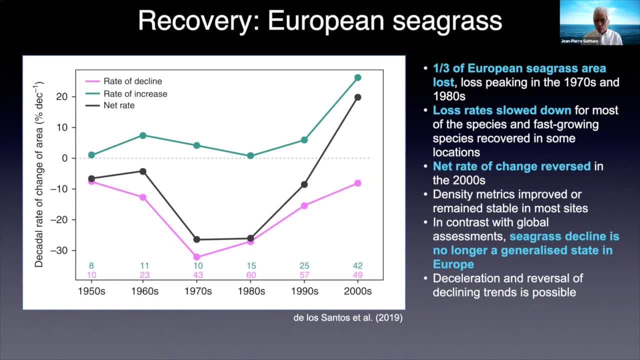 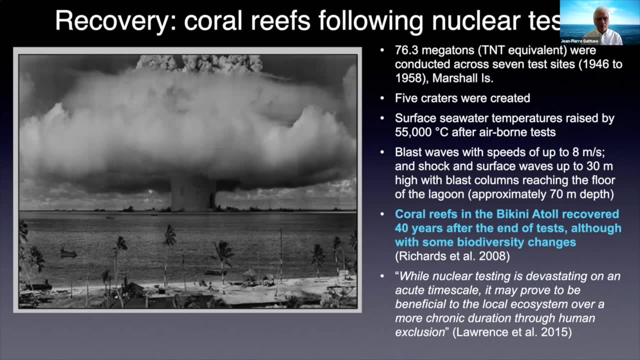 So there is definitely an opportunity to stop the decline and reverse it in the seagulls. Here an example of recovery of coral reefs with the largest destruction you can think of, That's nuclear testing in the Marshall Islands with tremendous destruction with surface seawater temperature. 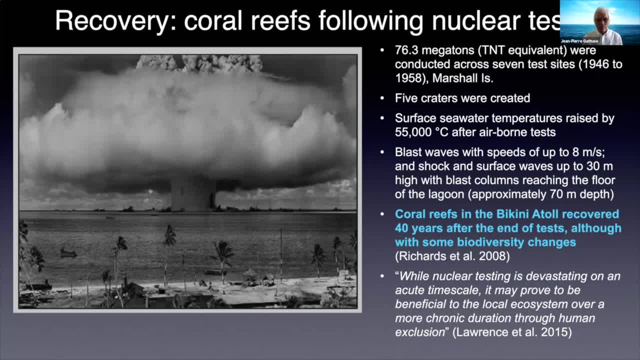 more than 50,000 degrees, shock waves, incredibly powerful, and down to the bottom of the atoll 70 meters. And 40 years later, the coral reefs in the Bikini Atoll have have recovered, although with biodiversity changes. 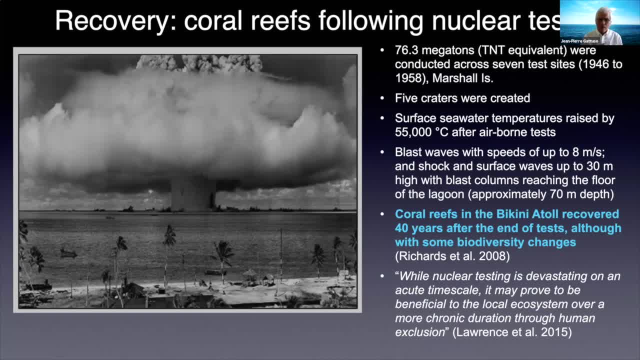 And this is a common aspect of restoration projects. Very often the diversity of plants or animals is less in the restored ecosystems. That's the case also for mangroves, And it even led this recovery to this more, perhaps more problematic view that in fact 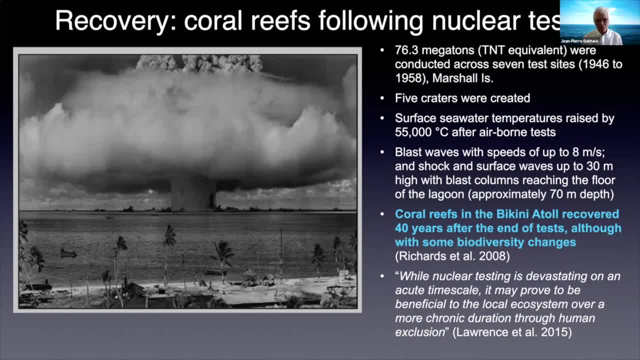 the nuclear testing is devastating on short timescales But it has proven to be beneficial to local ecosystems over a more chronic duration for human exclusion. So this is for Nancy to build on. So in the paper we looked at the development of NPAs. 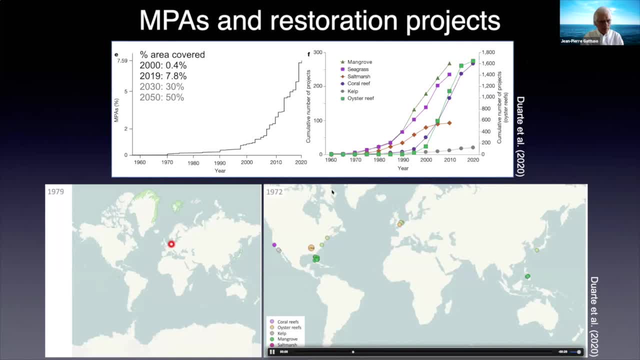 This is the first one, This is the first one, And in this panel, here this movie shows the increase in extent of marine protected areas as a function of time And here the number of locations of restoration projects for various ecosystems which are shown here. 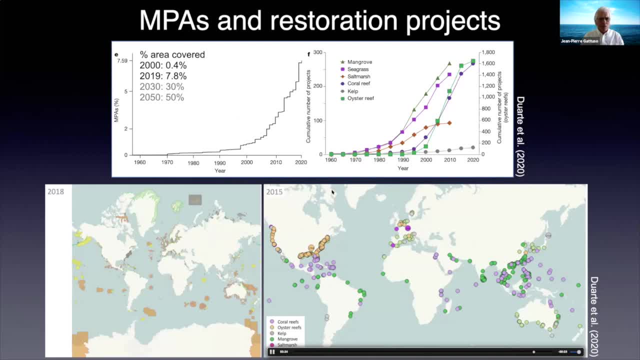 In terms of NPAs, the surface area covered by NPAs globally was less than 1% In 2000,. it is now almost 8% And there is a goal to reach 30% in 2030. And we contend that it is possible to go up to 50%. 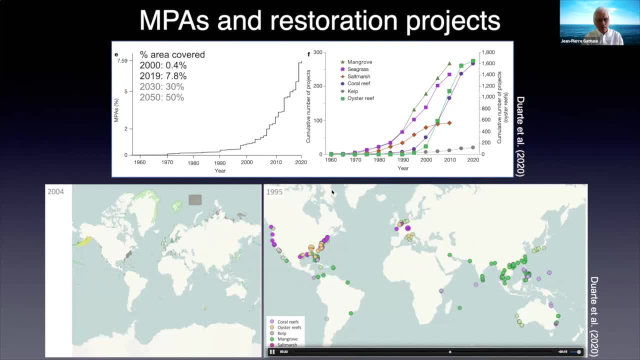 surface area of the ocean covered by NPAs by 2050. And here, on this side, this panel. this panel shows the number of projects, the cumulative number of projects, restoration projects of various types of critical coastal habitats- And this number of projects has increased tremendously. 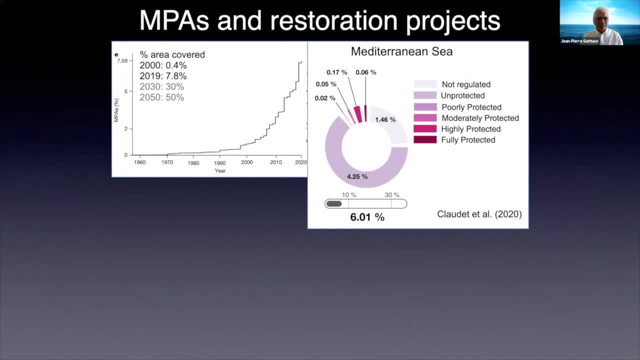 Of course, everything is not rosy Here. I take the example of NPAs in the Mediterranean Sea. a recent paper by Joachim Clodet and the NPAs- It's just a few months ago- which shows that 6% of the Mediterranean Sea. 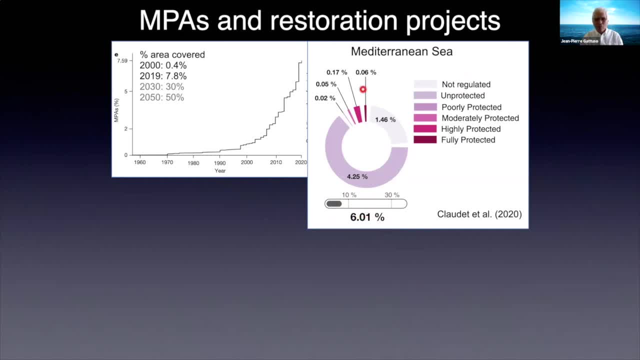 is covered by marine protected areas But in fact only 0.6% are fully protected, less than 2.2% highly protected, And you see that, in fact, protection is on a very small amount of the surface area. 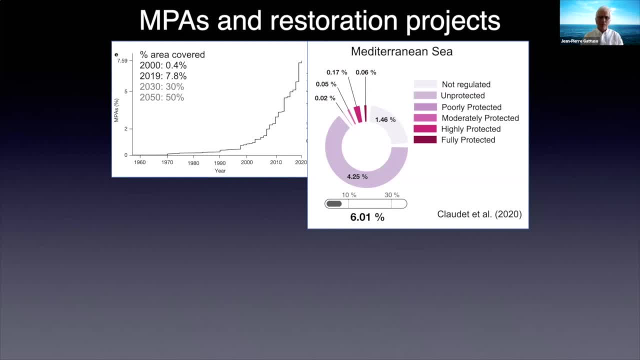 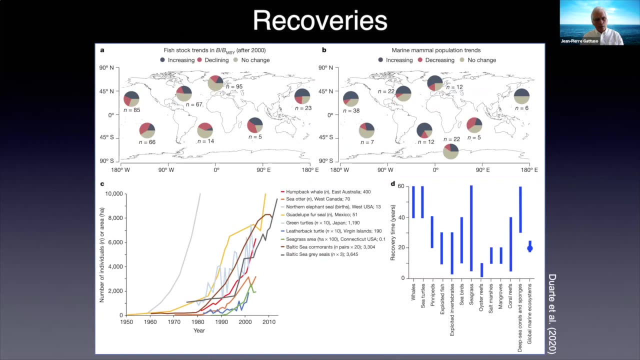 So it's important, And as marine protected areas have developed, that they are enforced And they are really protected areas and not NPAs and data In terms of recoveries. the review that we have done is summarized here. I'm going through it now. 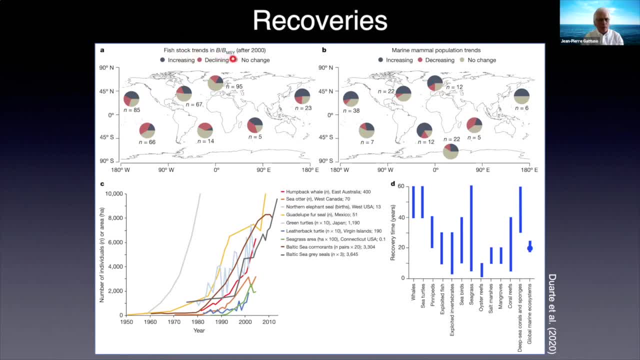 So here on the top left, the fish stock trends In the biomass, the ratio of biomass versus sustainable maximum sustainable biomass, showing that the fish stocks, still, some of them, are declining, But many here, this color, this grayish color, do not change. 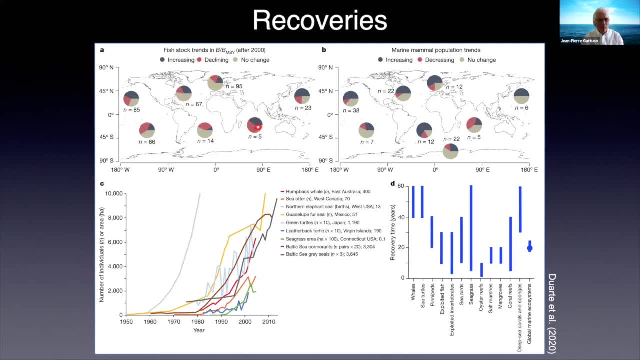 Some decline in the red And some increase, especially here, as we see in the Western Pacific. The numbers here show the number of stocks. In terms of marine mammal population trends, the situation is as follows: Few are still declining, especially here. 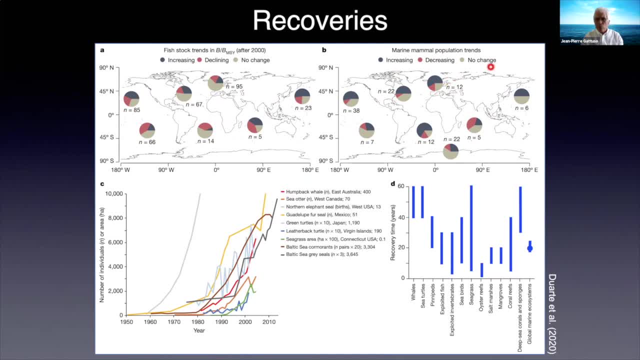 in the Indian Ocean, But many do not change the grayish color And some are increasingly blue, So, which is a good sign, of course, Here on this panel it shows the number of individuals, So the surface area covered, depending on what is considered. 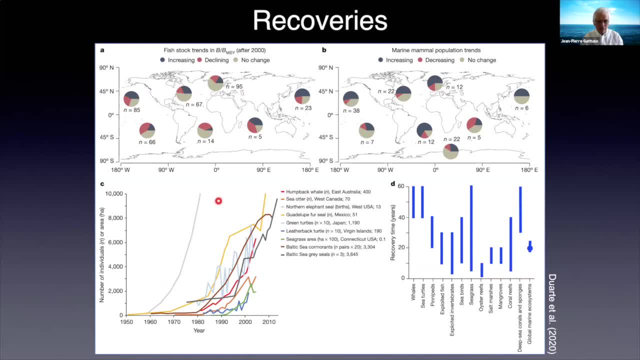 Perhaps the most spectacular recovery is here, the northern elephant seal On the west coast of the Midwest. there were an estimated 13.. But of the 11 seals at the beginning of the record, which is late 1950s And here now, more than 9,000 are currently developing. 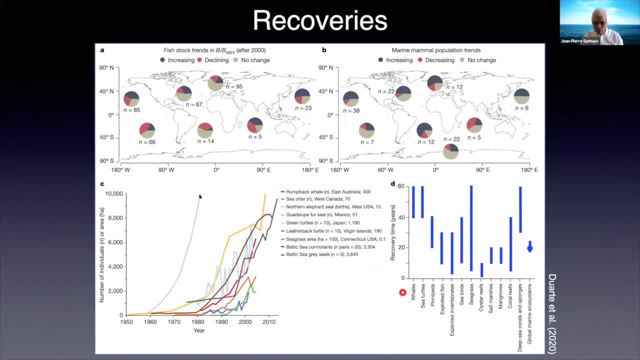 And finally here the recovery times for various species and key. it can be very fast And this is the mean of all those species and ecosystems, which is with the confidence and power showing that globally, those marine ecosystems can rebound, recover in 20 years. 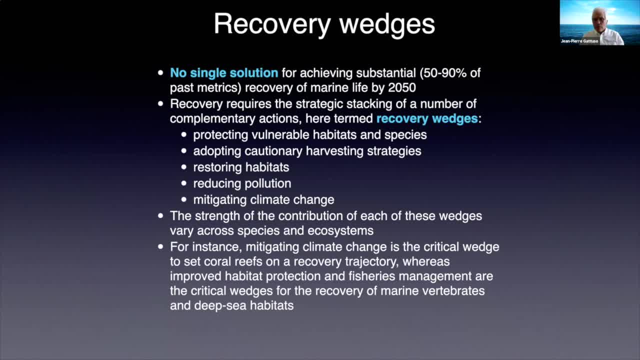 So there is no single solution for achieving what we call, in the data, substantial, that is, 50% to 90%. The recovery requires the stacking of what we call recovery wages, including protecting the mineral habitats and species, adopting our costumery and harvesting strategies. 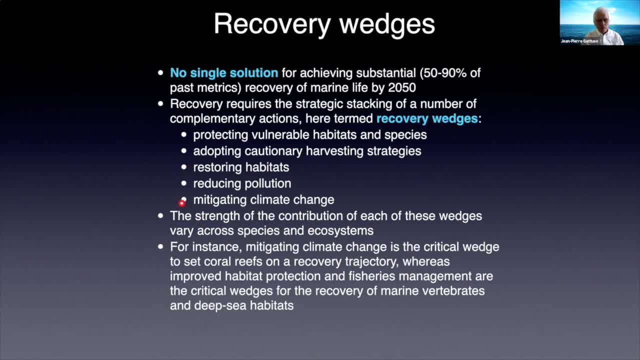 restoring habitats, reducing pollution and mitigating climate change. For the strengths of this actions, wages depend on different, of course, species and ecosystems. For example, mitigating climate change is absolutely essential to set coral reefs on. 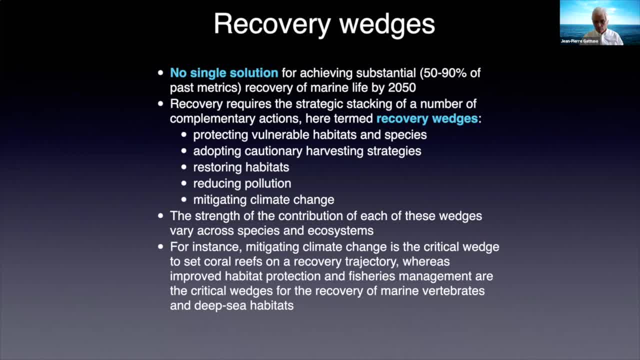 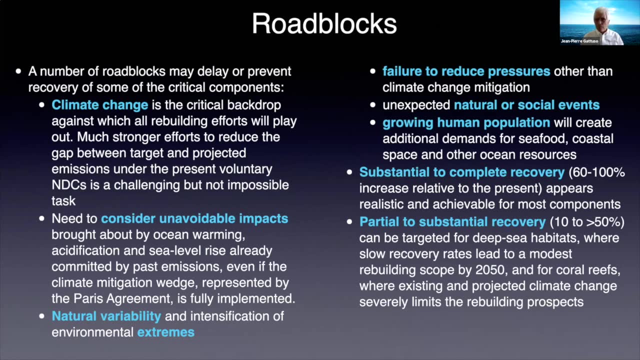 recovery strategy, whereas improved habitat protection and governance is a critical one for marine vertebrates and gypsy habitats. So there are roadblocks, obviously, and they are detailed in the paper. The main one is climate change roadblock, which is the critical background against which all 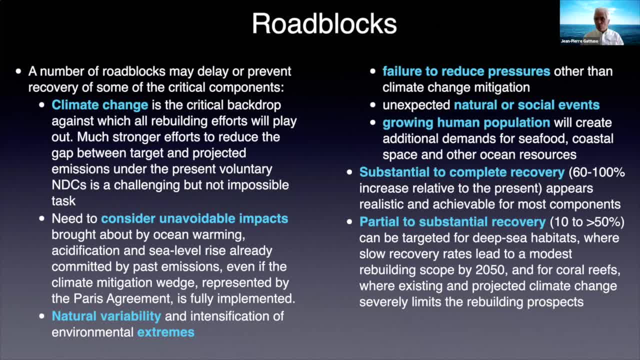 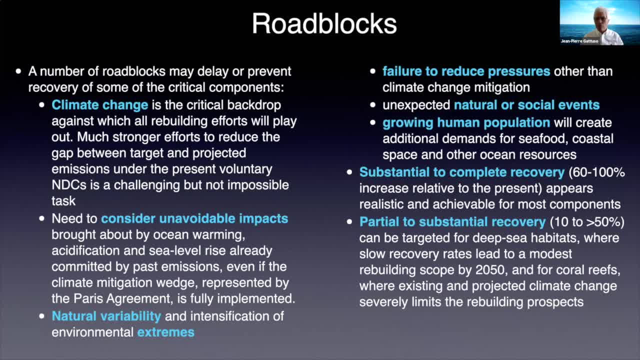 These are due to the committed changes in terms of warming, acidification and sea level rise. Natural variability also can impede recovery: The failure to reduce pressures other than climate change, such as pollution, for example, and expected natural or social events, and also the growing human populations which will have additional. 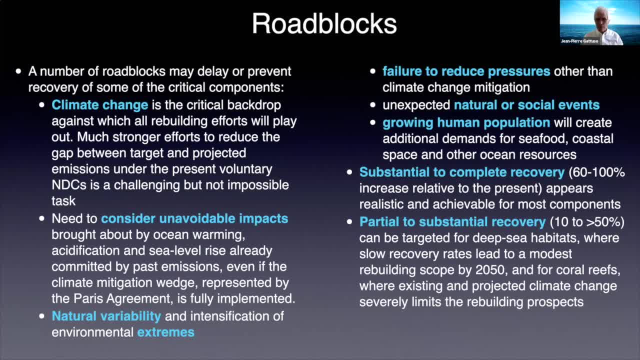 demands, The failure to reduce pressures other than climate change, such as pollution, for example, and also the growing human populations, which will have additional demands, And also the greater demands on the oceans for space, seafood and other ocean resources. But we contend that substantial to complete recovery appears to be realistic and achievable for most components, not all of them. 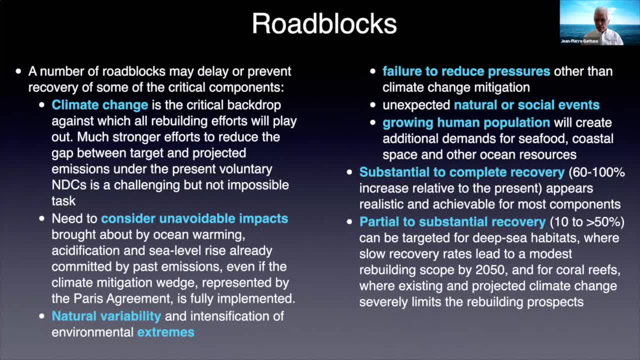 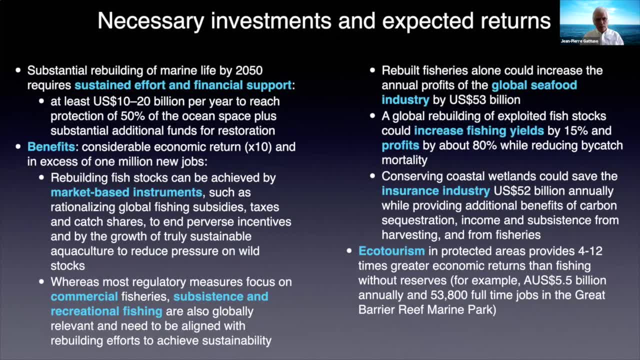 For most components if those roadblocks are lifted. So this will need investments But it will also provide a lot of growth. But it will also provide returns. In the paper it is estimated that at least 10 to 20 billion US dollars a year. 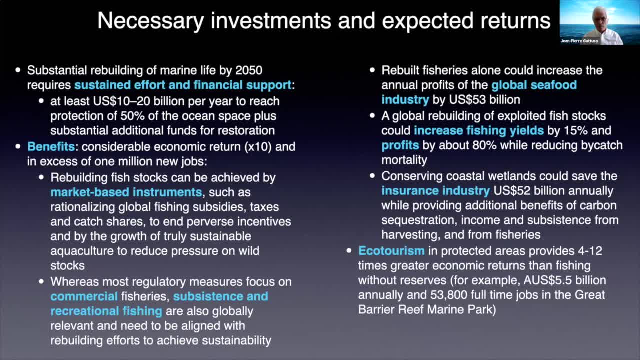 is needed to reach protection of 50% of the ocean space, plus substantial additional funding for restoration, It can be seen as a lot of money, but when you think of it- and I just went this morning on the Internet and saw that the profits of Apple 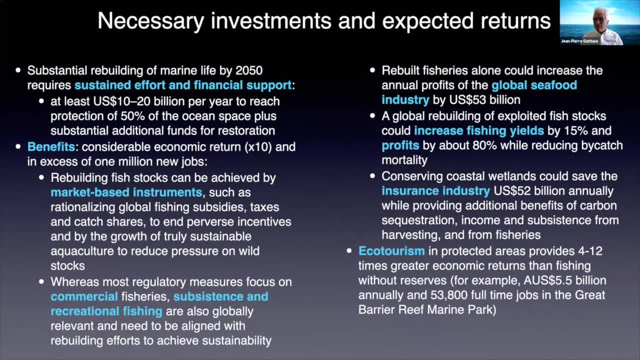 is 57 billion a year and the cost of ITER, this large-scale international effort, is 13 billion. So I think humanity needs this kind of investment, especially considering the benefits, which are considerable. Ten times for $1 invested, $10 can be expected back. 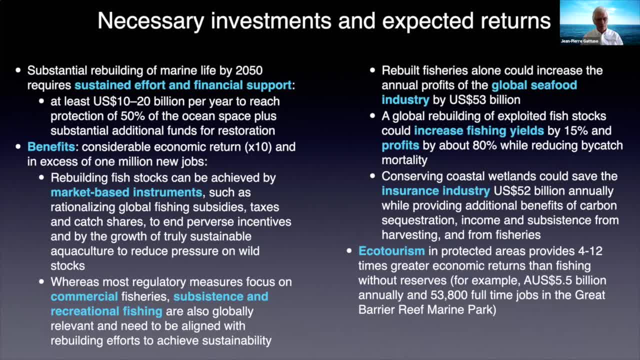 In excess of 1 million jobs can be expected also, So this will need using market-based instruments to rebuild fish stocks. It will also need to have regular, regular regulatory measures on commercial fisheries and also subsistence and recreational fishing. 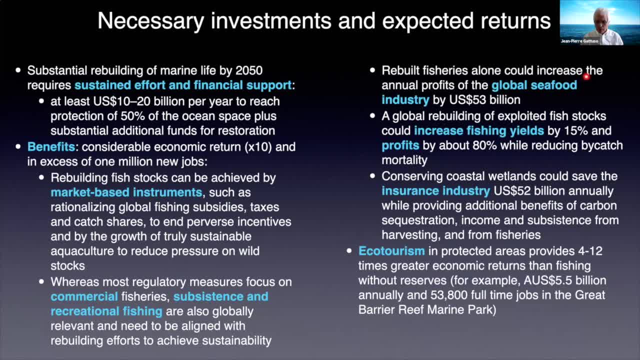 And the rebuilding of the fisheries alone could increase profits of the global seafood industry to 53 billion. Finally, this increase of profit by increasing fishing and also by reducing by 50 billion, reducing by-catch mortality. The insurance industry can benefit from this also by conserving coastal wetlands. 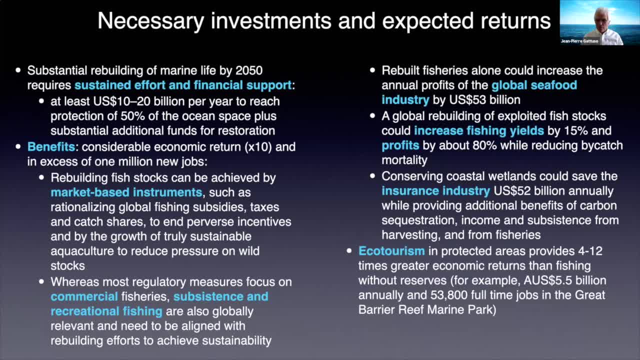 which will minimize, reduce destructions by flooding and provide additional benefits. And finally, ecotourism is also a big benefit of having a protected area, And it is also mentioned that the Great Barrier Reef Marine Park represents 5.5 billion US dollars annually. 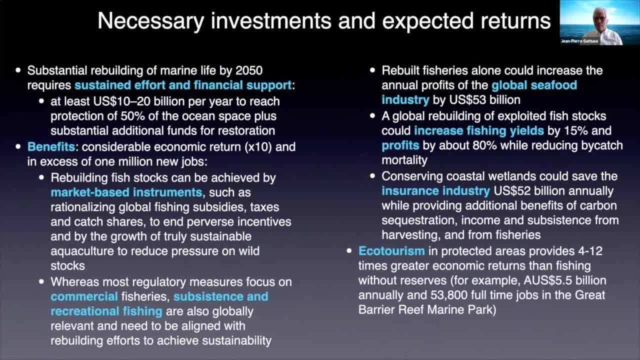 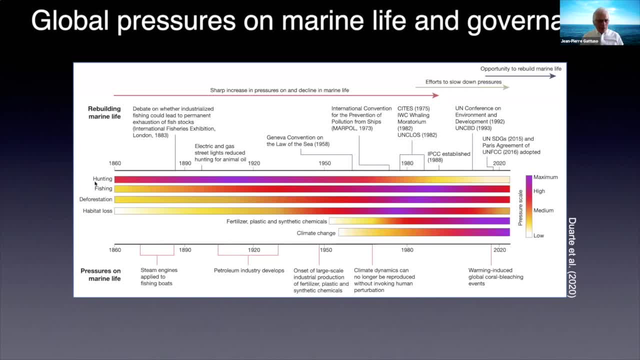 and maybe Australian dollars and more than 15,000 jobs. So here, hunting, fishing, deforestation and habitat loss have all peaked already at different times. The peak is shown by this purple color. But still pollution- chemical pollution and plastic pollution- is still increasing. 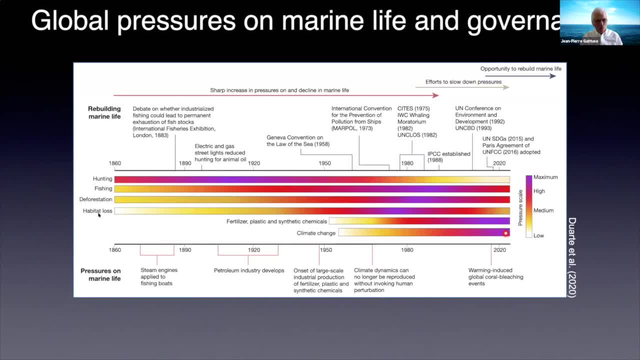 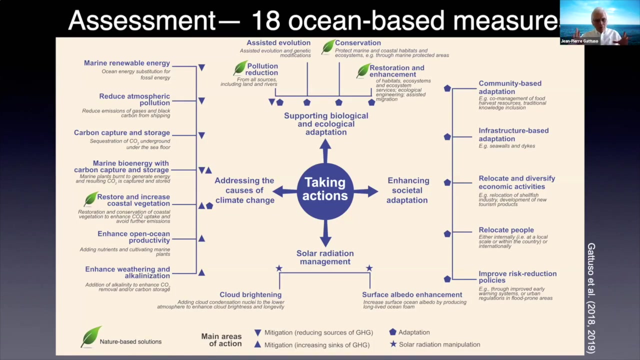 as we speak and climate change also is still increasing. So this increase in pressure has gone parallel to various governance instruments and I will let Daniela discuss those instruments. So, in the global, when we look at ocean-based measures to minimize climate change and its 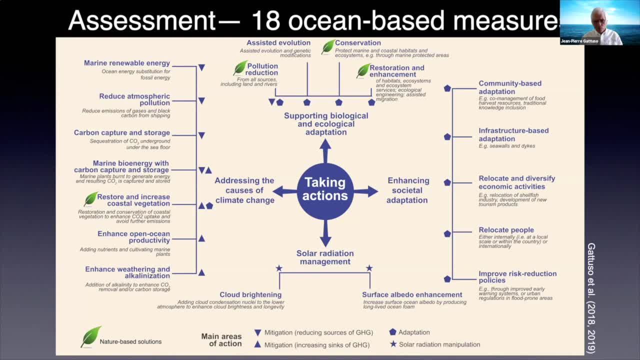 consequences. this is the outcome of a study we did at TIGRI with also my colleague Alexandre Magnon. We looked at various measures. they seem the causes of climate change, supporting biological and ecological adaptation and enhancing societal adaptation plus. 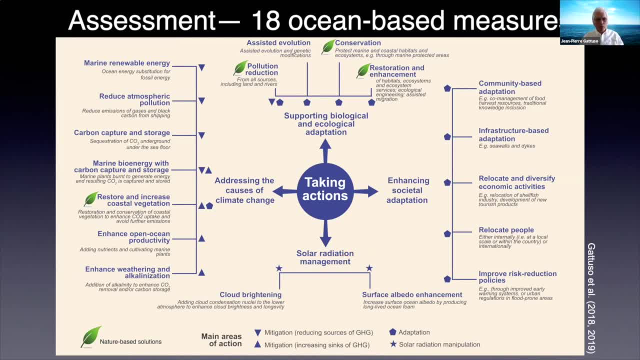 So we looked at various measures- they seem the causes of climate change, supporting biological and ecological adaptation and enhancing societal adaptation and enhancing societal adaptation, plus solar radiation management. We looked at all those measures and the ones I have discussed today with respect to the 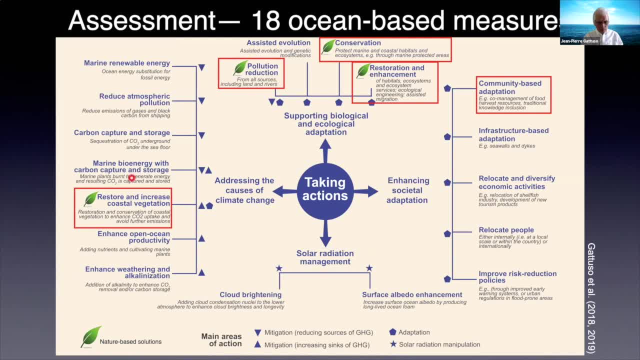 building marinas is only a few of them, And here restoring and increasing cost of vegetation, pollution reduction, conservation, restoration and enhancement of habitat and ecosystems, and community-based adaptation. There are many others that can be used with various effectiveness and in fact we. 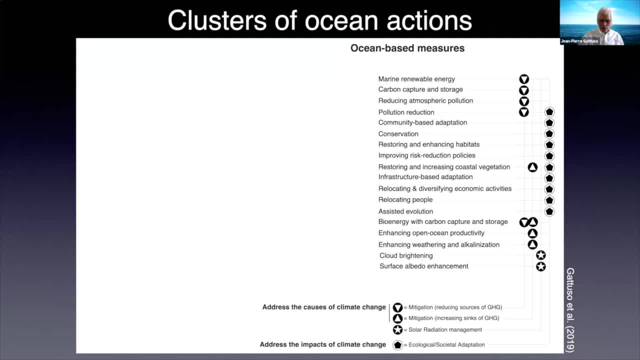 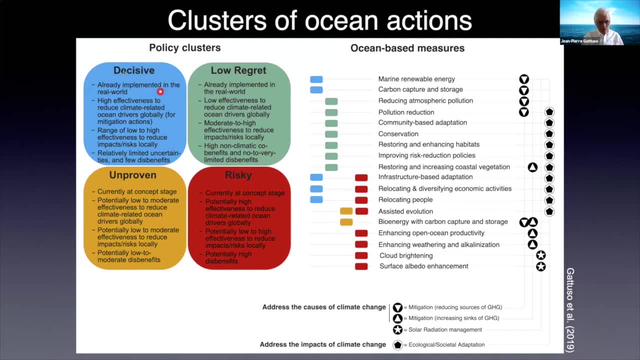 clustered those solution actions which are listed here, 18 of them- in four policy-relevant clusters: The decisive actions, the low-regret actions, the unproven ones and the risky ones. I don't have the time to spend today on this. 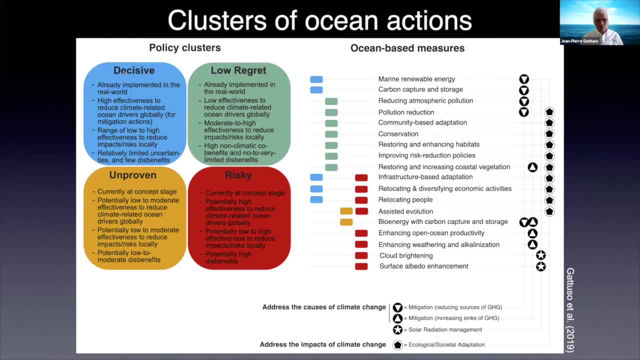 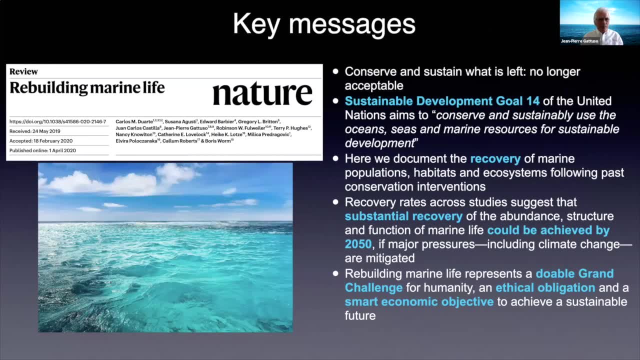 study, but I would be happy to answer any questions you may have. Finally, the key messages of this review article is that conserving and sustaining what is left is no longer acceptable. It was the goal in 1992 at the Earth Summit. 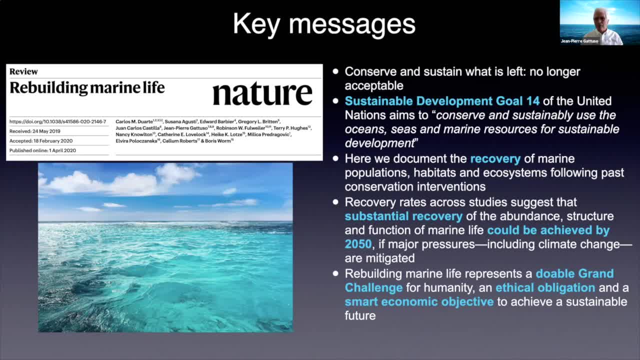 but, considering the degradation which took place since the 1990s, active interventions are needed to be able to reach this SDG 14 goal of the United Nations to conserve and sustainably use the ocean. Here in this paper we document the recovery of marine populations, habitat and ecosystems following past conservation interventions. 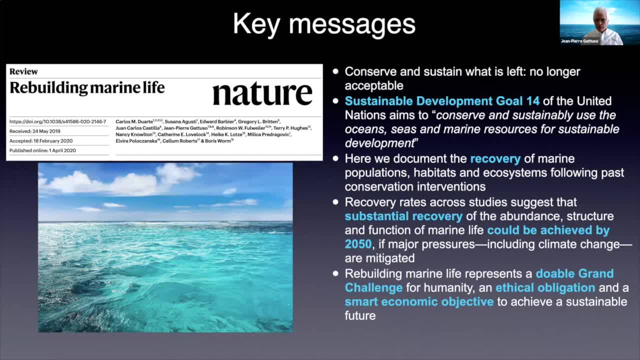 We show that recovery rates across studies suggest that substantial recovery, that is, 50 to 90% improvement, could be achieved by 2015 if major pressures, including climate change, are mitigated. And to conclude, rebuilding marine life really, we believe, is a doable, grand challenge for humanity. 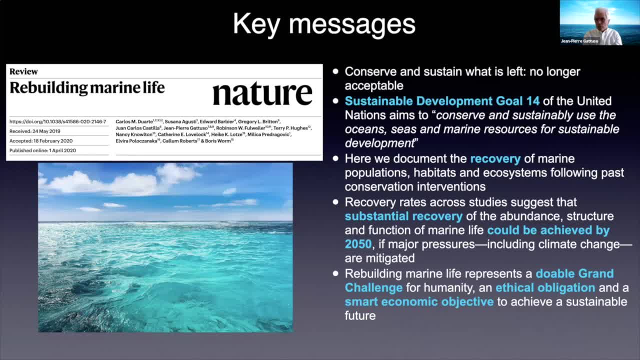 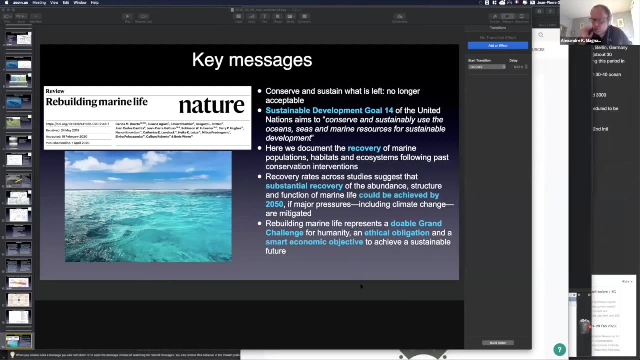 It's an ethical obligation for future generations and it is also a smart economic objective to achieve a sustainable future. Thank you very much. Thank you, Jean-Pierre. We had a lot of questions here, so maybe I can ask at least one for the moment, and then we will come back on others. 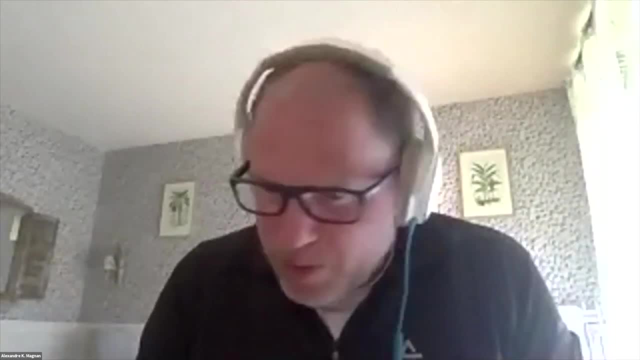 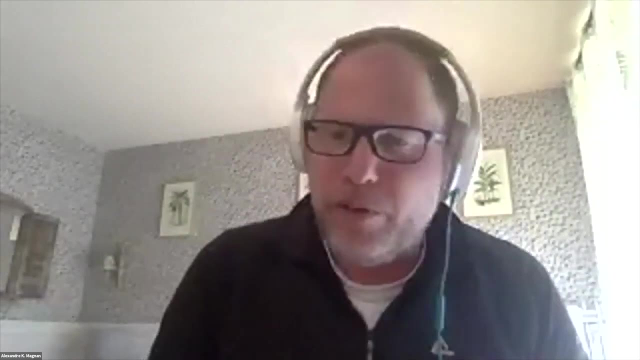 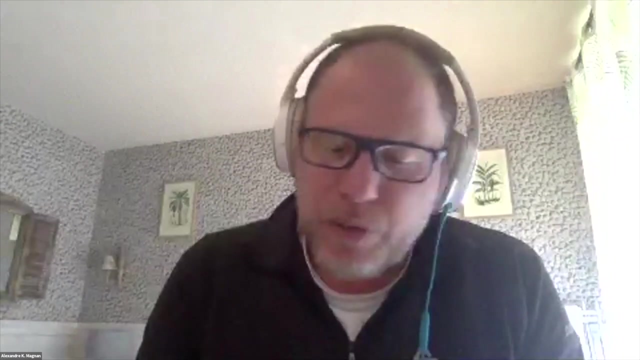 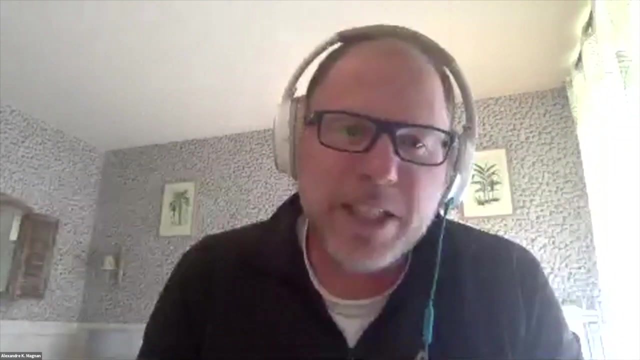 Later. the choice is difficult between the questions. Maybe one is Jean-Pierre. someone is asking and it's converged with other questions. We understand that a huge restoration effort could be beneficial under certain conditions, But we know that our investment capacity in economic terms, but not only. 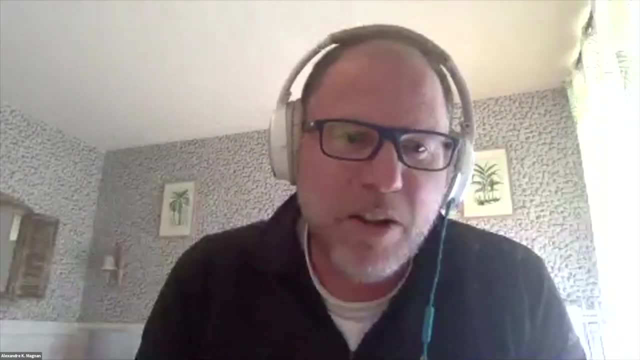 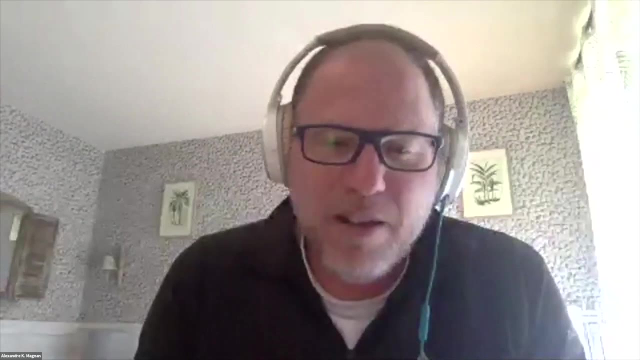 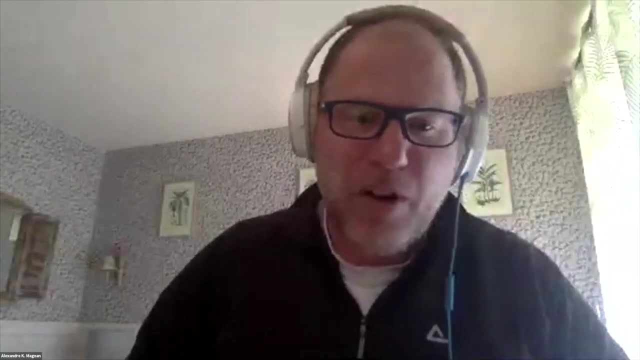 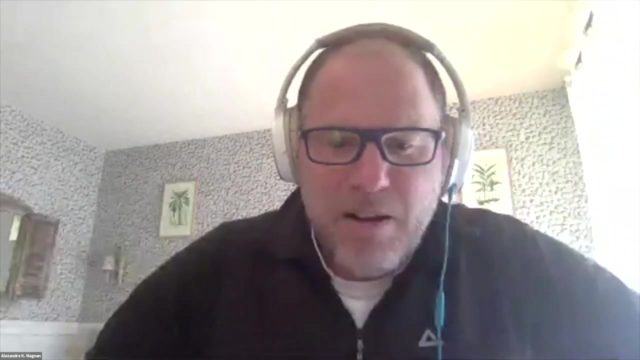 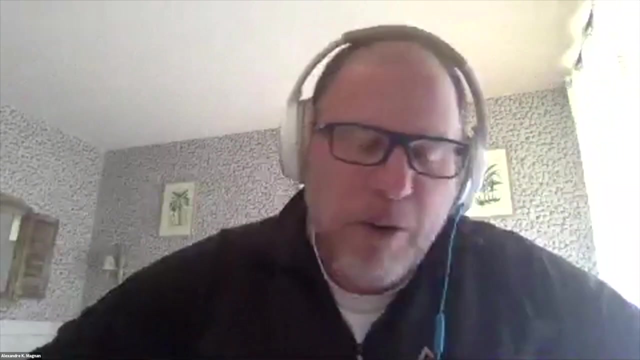 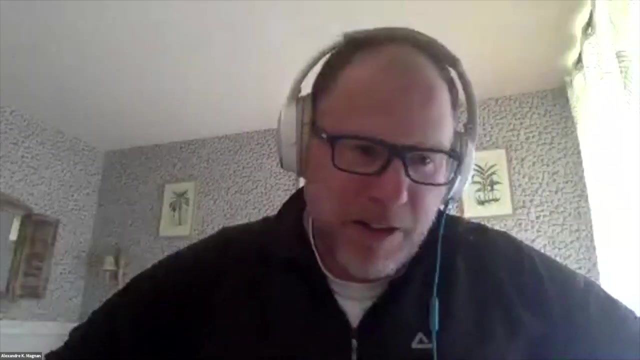 I mean on the policy side and so on- is limited. So the question of the priority raises: do we have to put some priority on restoration or rebuilding marine life in terms of priority species or priority areas? And a parallel question. I know you won't be able to answer everything, but a parallel question is: do we need to prioritize areas or species that are already seriously damaged? 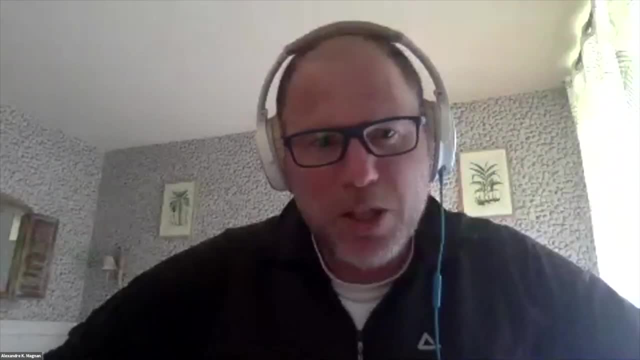 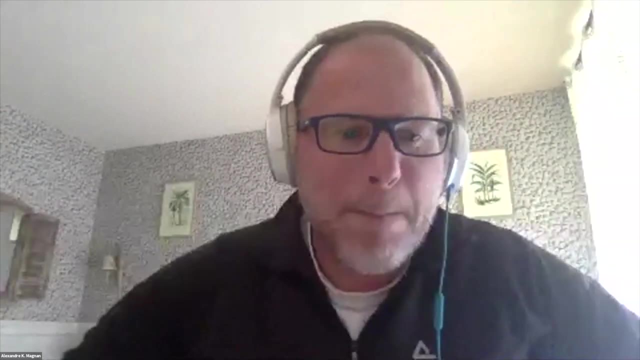 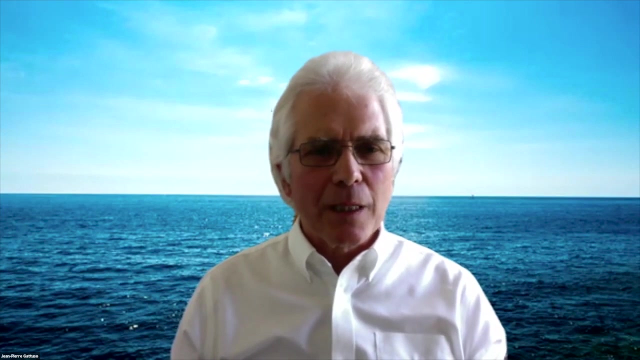 Or do we have to prioritize species or ecosystems or geographies that still have some natural adaptive capacity? OK, the first part of your question was about financial possibilities. I believe the financial possibility is here. Look in Europe. The European Commission is about to release 700 billion euros to deal with this acute pandemic of COVID-19.. 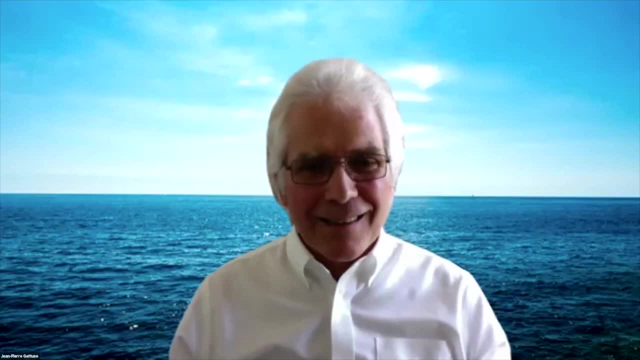 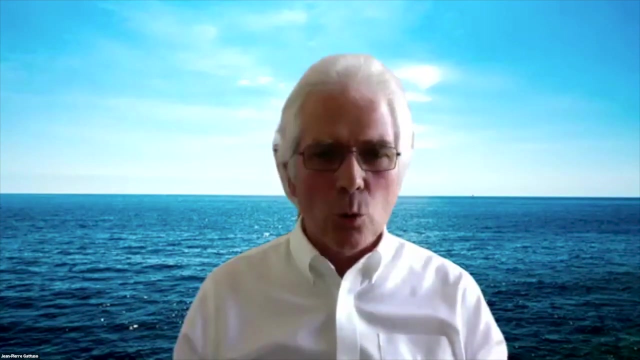 And this was mobilized within a few weeks. It is a wise investment, of course, to do that. I mean no doubt about it, But it shows that when there is a huge problem coming up, such as the pandemic, the human societies are able to mobilize a huge amount of funding. 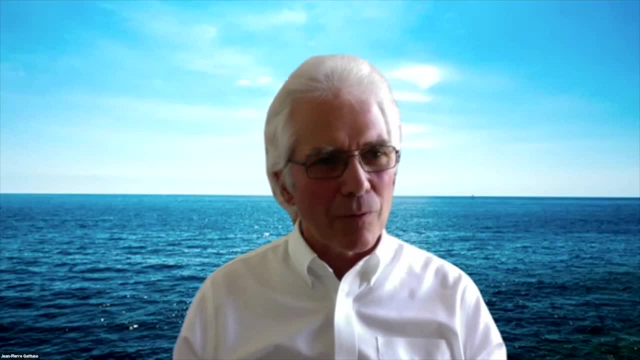 And the money we are talking about with rebuilding marine life is not that big And the benefits are tremendous. I would argue that the consequences of climate change and the loss of biodiversity probably exceed the destruction of the COVID-19 pandemic. I think the resources can be mobilized. 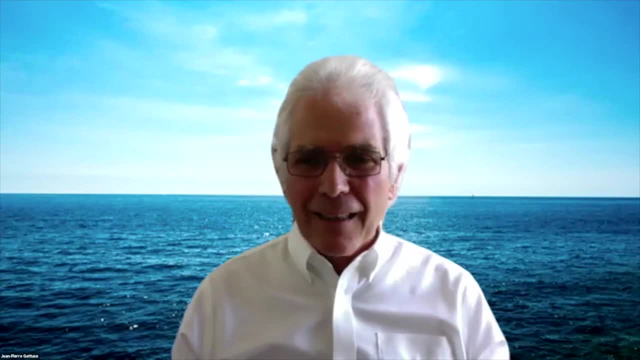 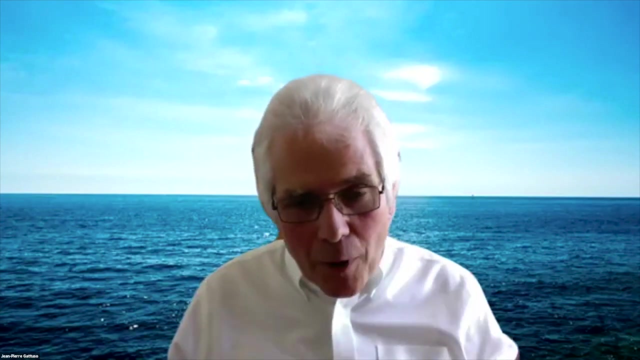 It's a matter of will. The second part of your question was whether we need to focus on specific areas. Look for the climate change roadblock. Of course climate change can be minimized globally. of course It's not at the local scale. 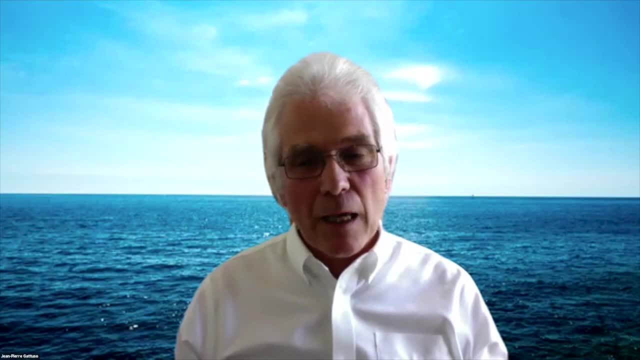 But working efficiently to minimize climate change will benefit every coastal and marine ocean system, So there is no need there to be specifically focusing on specific areas. If you ask me which are the ecosystems that are the most threatened, there is, of course, coral reefs. 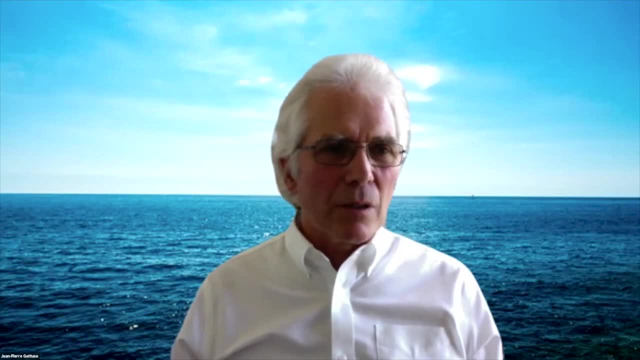 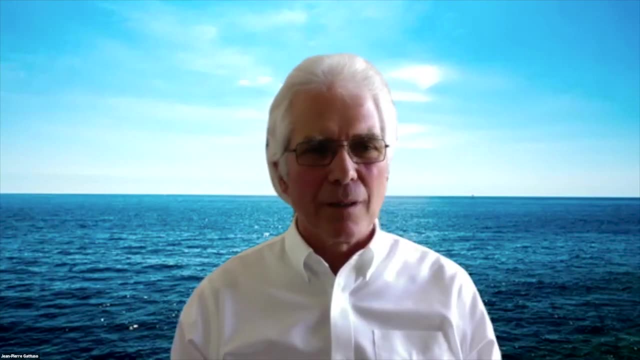 I'm sure Nancy will address that- And every coastal ecosystem because of the big demand on the coast: mangroves because trees are cut back to build roads, coastal infrastructures to build aquaculture ponds, So seagrasses also are very affected by increased delivery of silt and sediments. 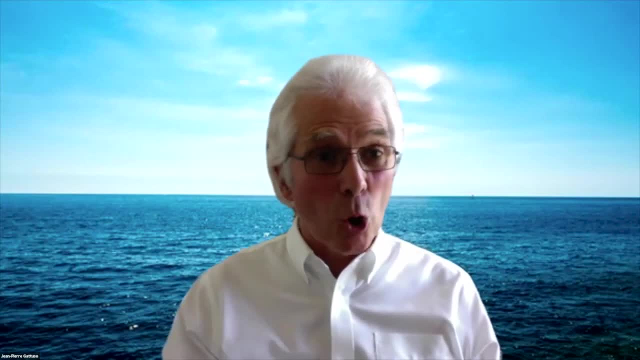 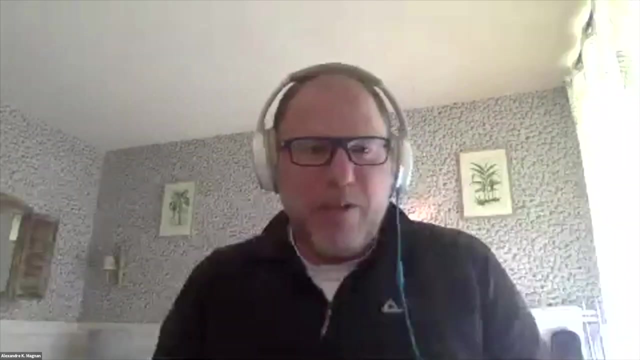 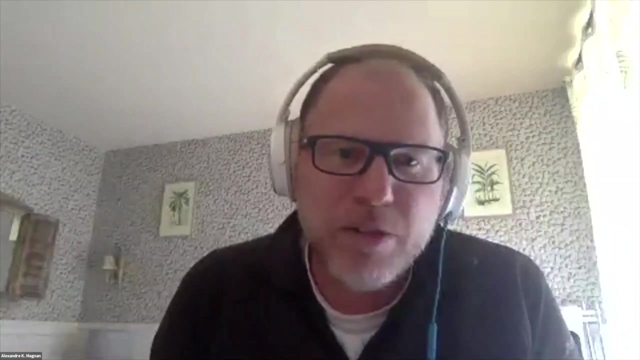 Because of deforestation on land. So all those coastal ecosystems are pretty much the ones on which we should focus the attention. I think Yeah, thank you, Jean-Pierre. It's true that the topic is complex because we are with this study. which is interesting is that it deals with multiple threats and multiple drivers of stress. 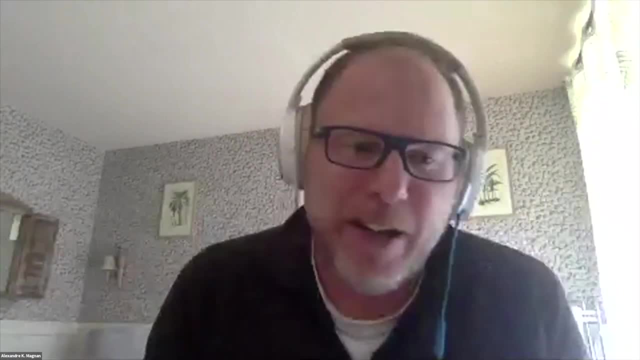 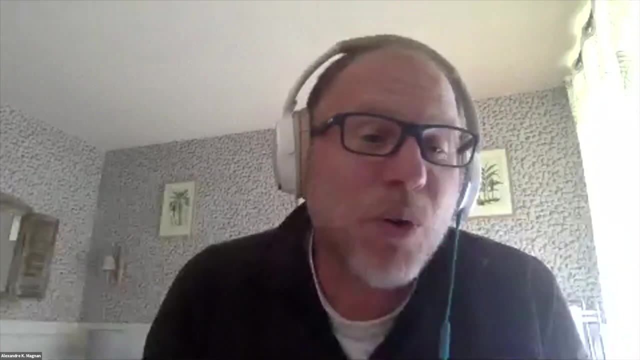 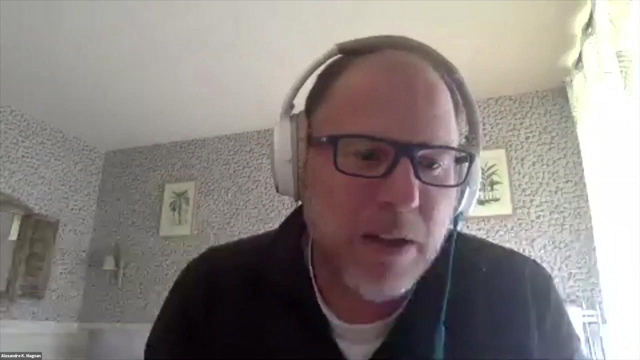 And when we are in the multiple driver of stress area, a lot of ecosystems, also in the open ocean, are threatened. And, of course, you mentioned coral reefs. So, Nancy, that will be your turn, of course, And coral reefs are really both highlighted in media and maybe with wrong messages. 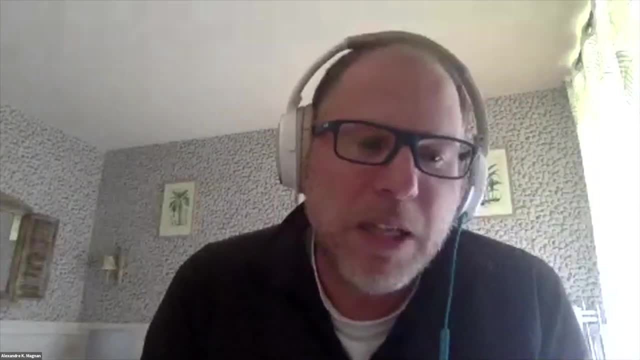 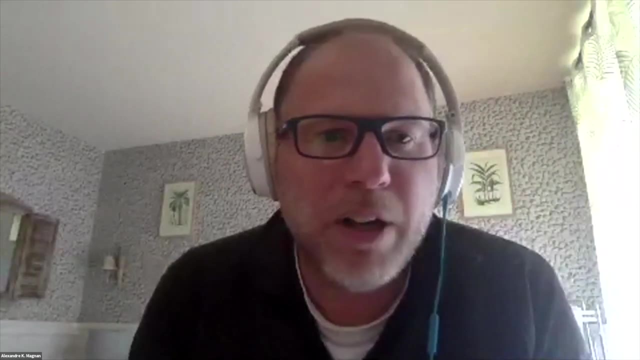 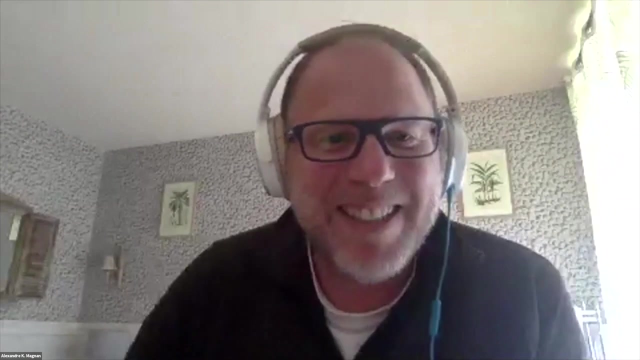 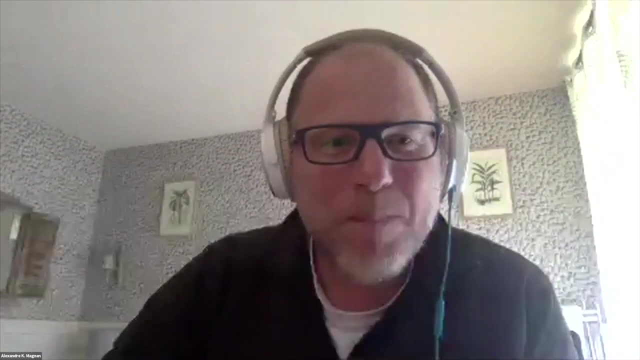 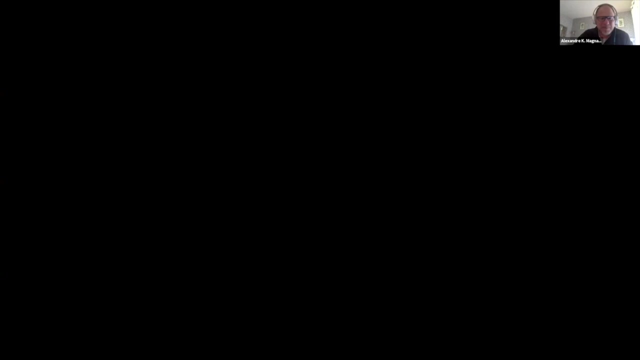 It's hard to know when you are not an expert, But a lot of attention is paid to coral reefs around the world, also because of recreational activities and so on. So we would like to hear more about this fantastic ecosystem, Nancy, So we can see your screen, Nancy. 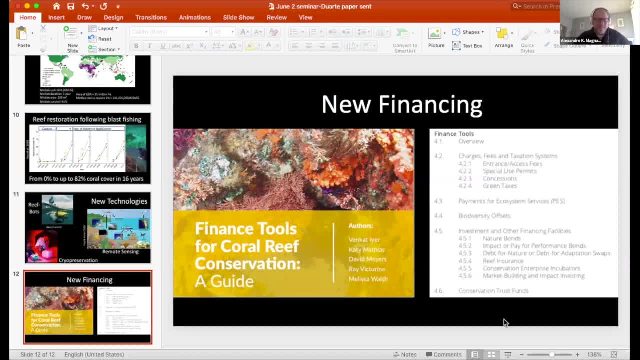 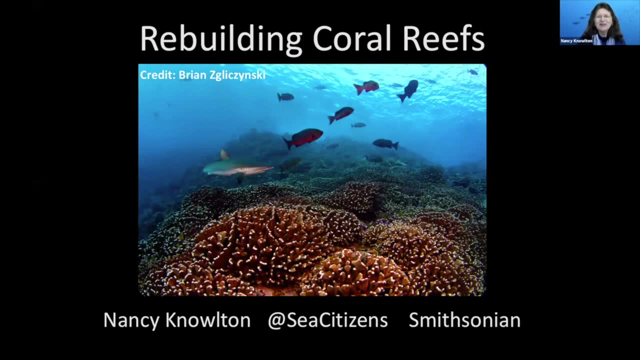 That's good, Thank you, Can you see me? Can you see my screen now? Yes, and we can hear you. Perfect, Can you see my screen and hear me? Yeah, Excellent, Okay, I'm getting that little message on my computer saying the Internet is unstable, but hopefully this will keep working. 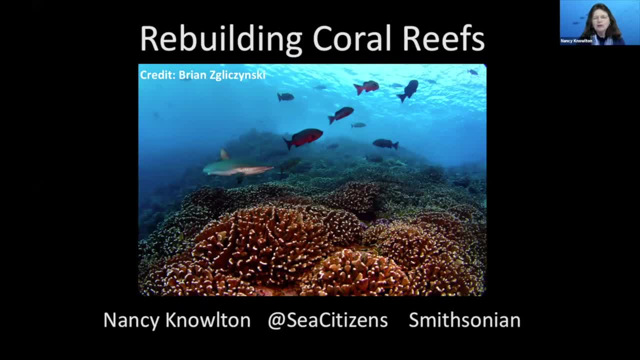 Well, thank you very much for this opportunity to talk about coral reefs. As has been alluded to in the previous discussions, in some ways they're the most challenging of all the marine ecosystems we have to worry about, And indeed in the Dwarte et al paper that we're referring to repeatedly, it was one of only two ecosystems where the prediction was more along the lines of partial to substantial recovery, rather than substantial recovery. 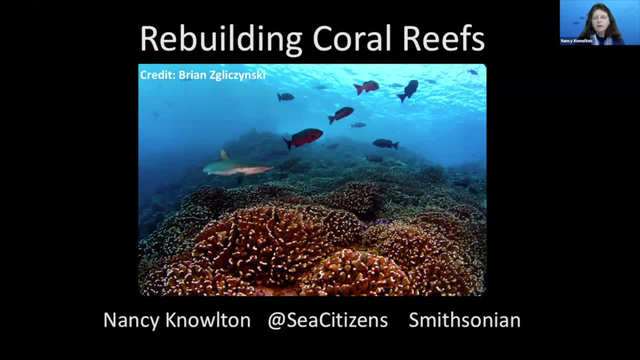 So it is a challenge. It's a challenging ecosystem to work in in terms of thinking about how to make them healthier and rebuild them, And in fact, they've often been called the canary in the environmental coal mine because they are so sensitive to so many different aspects of human activity. 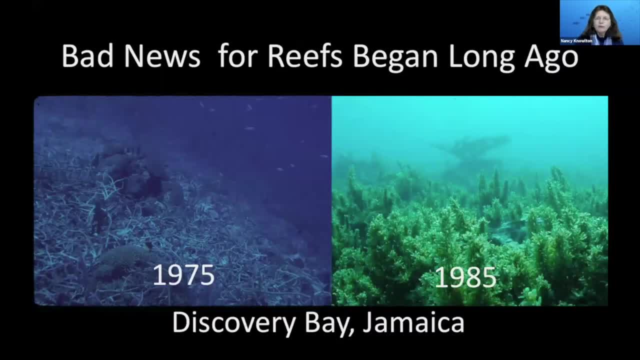 So the bad news for reefs actually began a long time ago. You see on the left A picture I took, actually as a graduate student, which is dating me a bit, And although you can see that reef was covered with living coral, all those little branches and heads, that's all live coral. 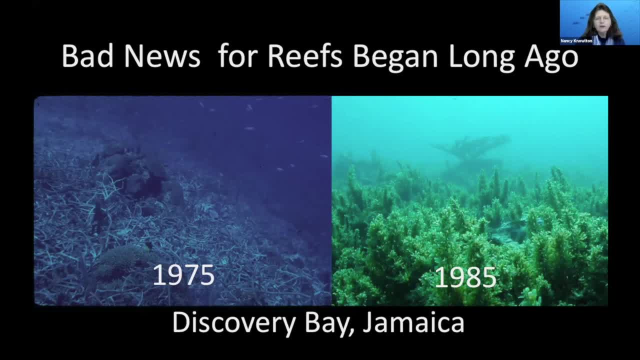 So it was. in that sense it was a very healthy coral reef. But even back in 1975, we realized that it was not certainly far from pristine, And that was because what's not in the picture that I took, Which is any large fish. 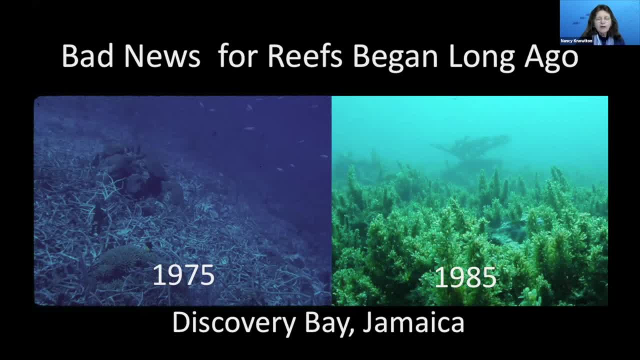 And when we were there during our research, we, although we noticed the absence of healthy fish communities, we didn't really worry about them In terms of the health of the coral. And that turned out to be a huge mistake, Because within 10 years, those reefs, the corals, were mostly dead and covered with seaweeds, which is what you see on the right hand side. 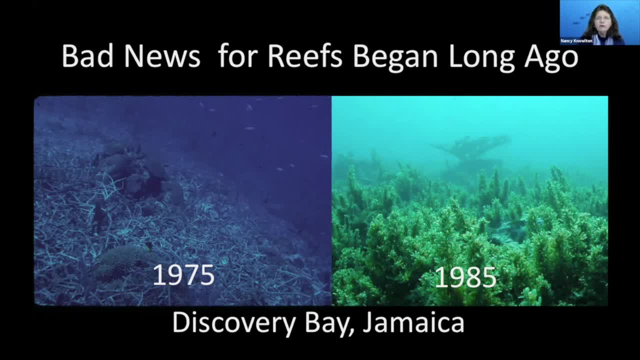 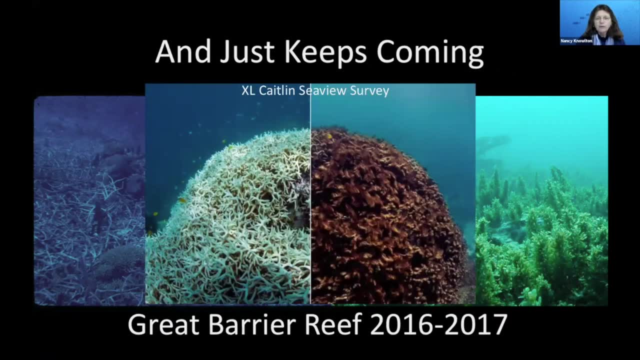 Now, of course, this bad news Just keeps coming, And I'm sure all of you have read something about what happened to the Great Barrier Reef between 2016 and 2017.. Back to back: major bleaching events caused by water that was too warm. 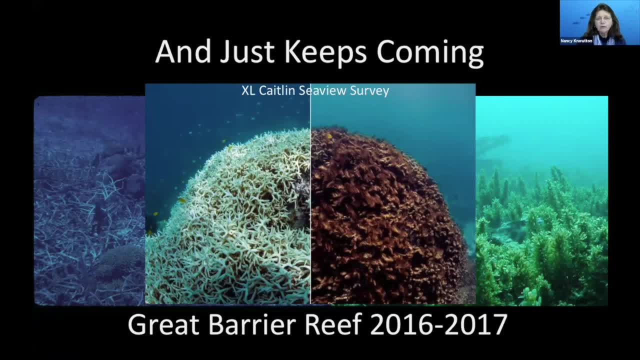 And in fact, there's even a bleaching event that has been going on this year as well. So when I started working on coral reefs, The biggest problem was actually not climate change. In fact, the collapse of those reefs had to do with, as I mentioned, overfishing. 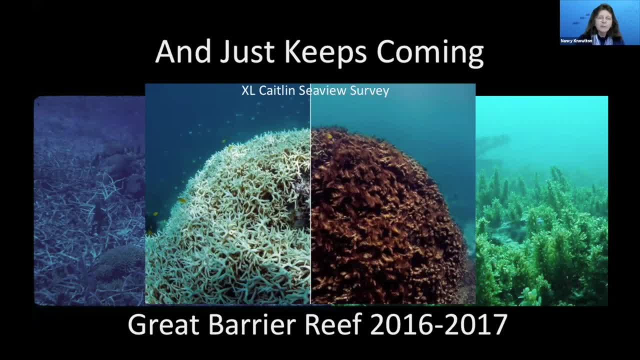 And combined with a disease that eliminated most of the remaining herbivores. That's a disease that struck a particularly important sea urchin, So that earlier collapse in Jamaica was not a function of climate change. This, on the other hand, in the Great Barrier Reef and increasingly around the world, with massive bleaching events occurring on a regular basis, is associated with climate change. 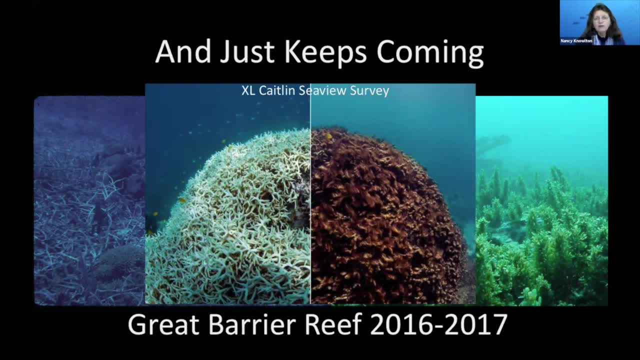 And so it's an illustration of how many different things over the course of my career, beginning in the 1970s, How many different things have impacted coral reefs to their Great Barrier Reef, And this is really a global tragedy And it affects many, many countries. 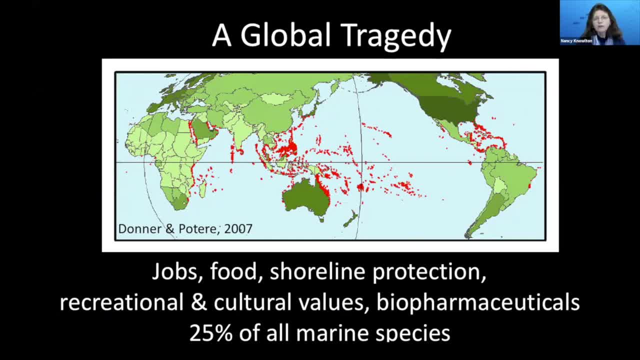 About 100 countries have coral reefs along their shores, And these coral reefs provide jobs, They provide food, They provide shoreline protection in the case of major storms or tsunamis. They also represent really important recreational and cultural values, Even the potential for important biopharmaceuticals, some of which have been explored but many of which have not been. 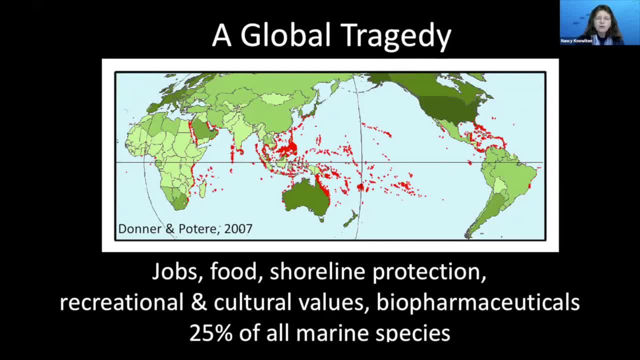 And in addition to the human values, it's estimated that coral reefs shelter about 25% of all marine species- And this tragedy, this global tragedy, is particularly affecting developing countries. You can see this map shows the presence of coral reefs in red dots. 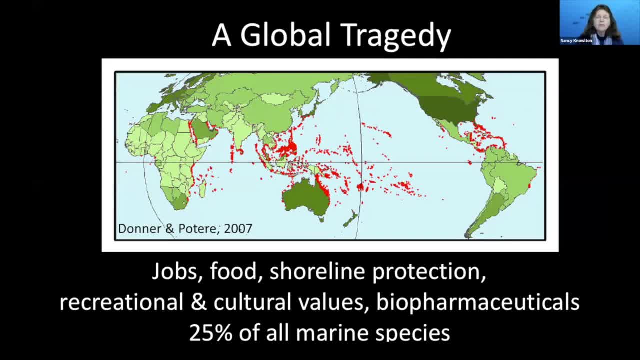 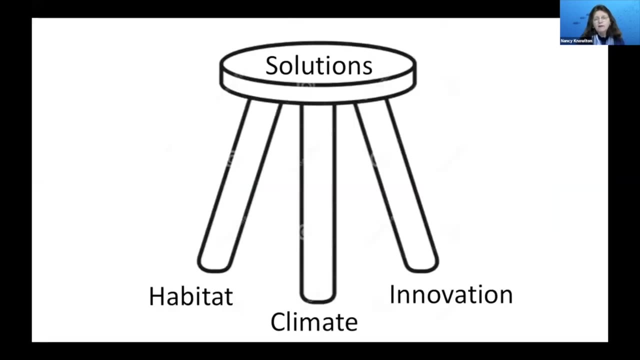 But the economic development status is indicated by the shades of green And, as you can see, most coral reefs are near countries that are developing economies, not strong economies, So the blow is particularly severe in most cases. Now I don't want to spend. I have only a limited amount of time. 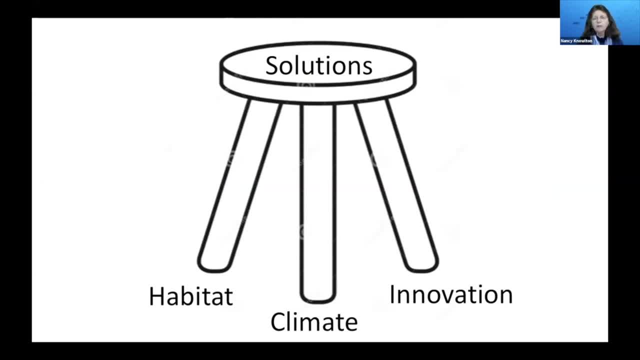 And so I could spend an hour talking about all the threats and the problems. But really the purpose of the Duarte paper and my presentation today is to talk about the solutions And why we feel that even for coral reefs it is possible to start talking about recovery and rebuilding. 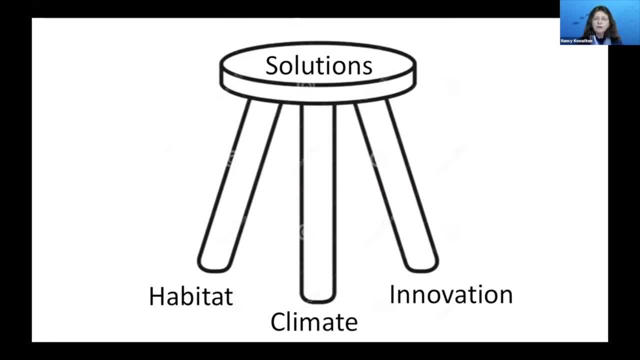 And I'd like to frame those solutions in the context of a three-legged stool in terms of what we need to do Now. obviously, as has been alluded to before, we need to address climate change, Because corals are very, very sensitive to relatively small increases in temperature. 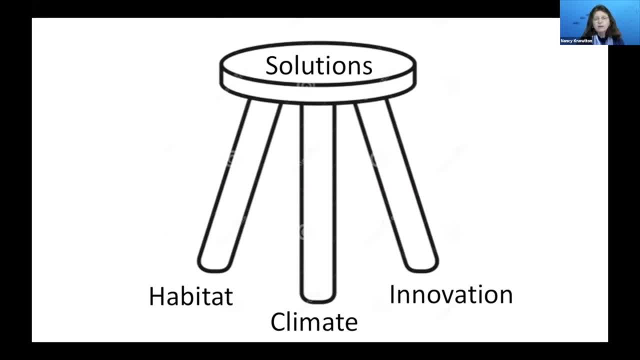 Just one degree centigrade, for example, can start the bleaching process, And so if we don't address climate, we really don't have any hope of really protecting and restoring coral reefs. But as my experience that I described in Discovery Bay, Jamaica, illustrates, 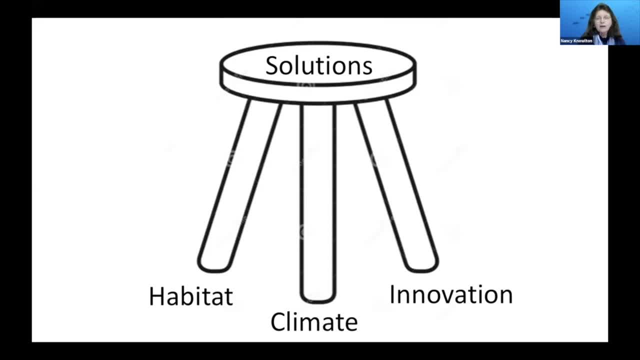 we also have to protect the other aspects of habitat, in particular, in that case, with fish. And then, finally, we're going to have to innovate, Because, even though habitat protection is something we know how to do, climate is something that, even to the extent that we know how to address it. 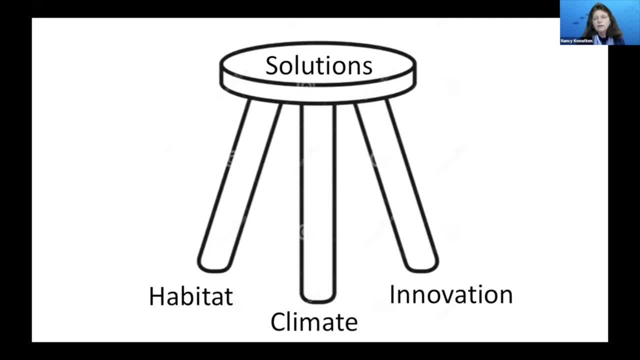 is simply going to take time because of the inertia in the physical system and the inertia in human, social, economic systems, And so this is really a three-legged stool, in the sense that all three of these aspects of the solutions are needed, And I think it's that too much time and too many people have really engaged in arguments. 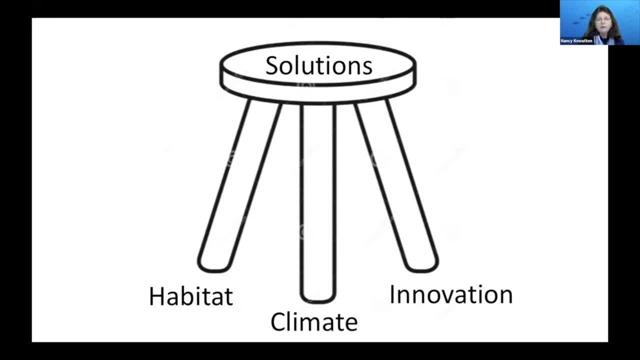 that climate's the only thing that matters, or if you don't protect fish and have clean water that's the only thing, or innovation is a waste of time because it won't be ready fast enough. We really need all three of those elements of the solution space. 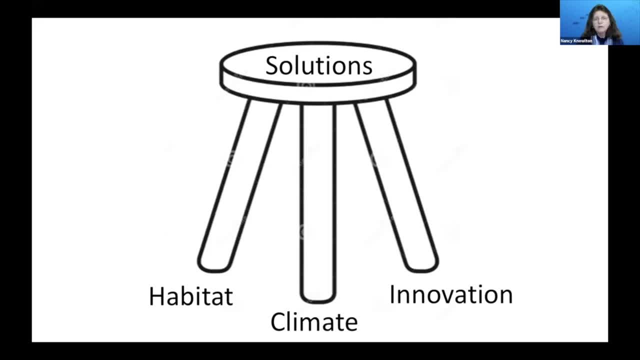 in order to make progress on coral reefs, And what I'd like to do is very quickly review some aspects of those and then give just a very few examples of things that I think are demonstrated solutions or exciting prospects in the future, And I'm not going to talk about climate anymore at all, because that's a topic. 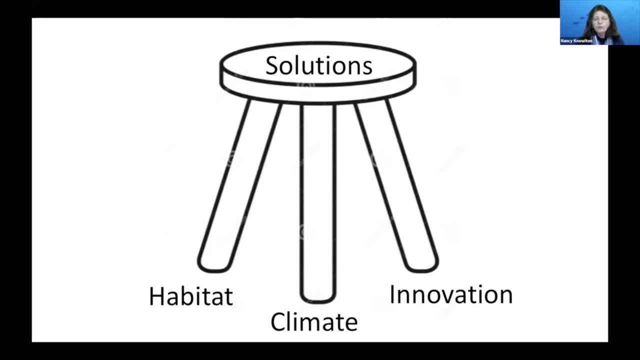 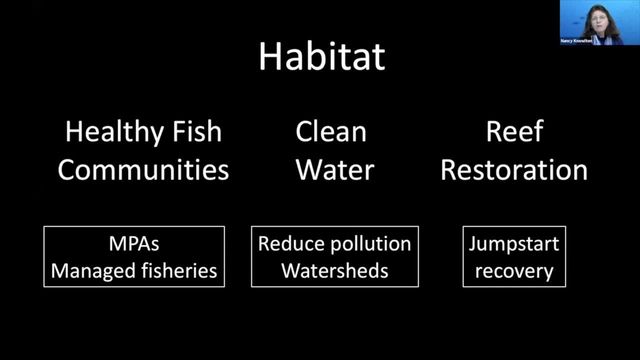 that could be a whole other webinar, So I'll focus now on habitat and innovation. So, in terms of habitat, really what coral reefs need are healthy fish communities and clean water, And we actually know how to achieve those things. These are what I would call the traditional approaches to coral reef conservation. 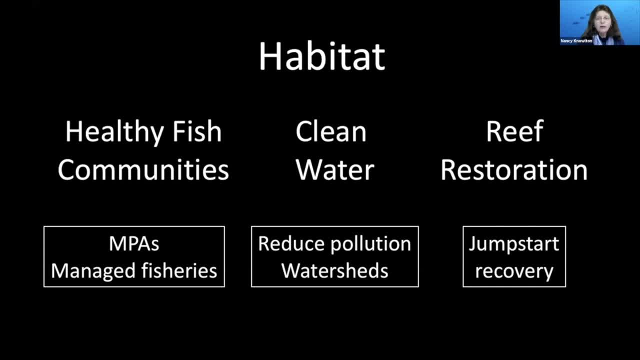 And for healthy fish communities. we need marine protected areas, but we also need managed fisheries in areas where people are using reef fish in order to feed their families, For example. they need clean water, And that is, again, relatively straightforward in principle. 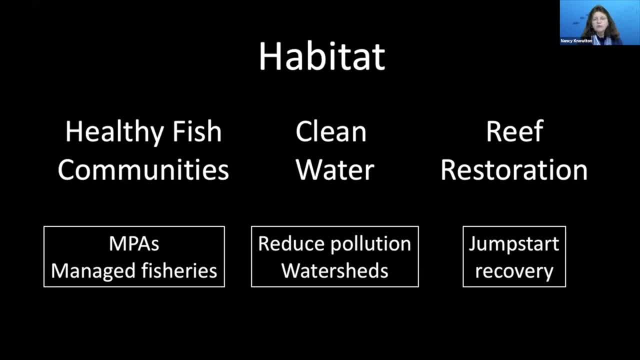 not necessarily straightforward in terms of the execution. You need to reduce pollution and you need to manage watersheds so that they can capture what pollution is being created, And then, as has been mentioned, you need to think about actual reef restoration because the damage has been so severe. 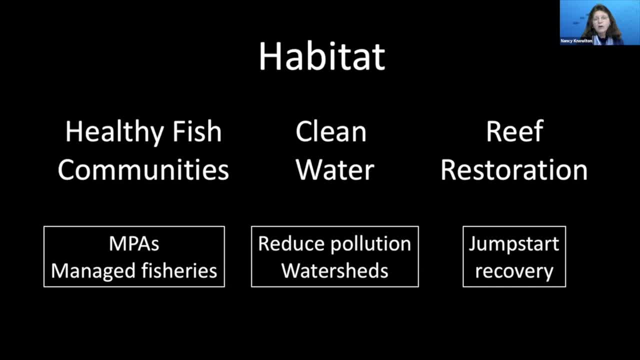 Somewhere between 40 and 50 percent of all coral reefs or corals have been lost over the last several decades. Now, this is not a discussion about physically rebuilding every single piece of lost reef, but reef restoration can be very important in terms of jump-starting the recovery process. 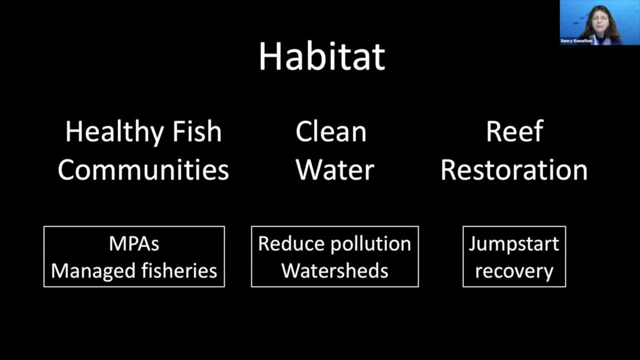 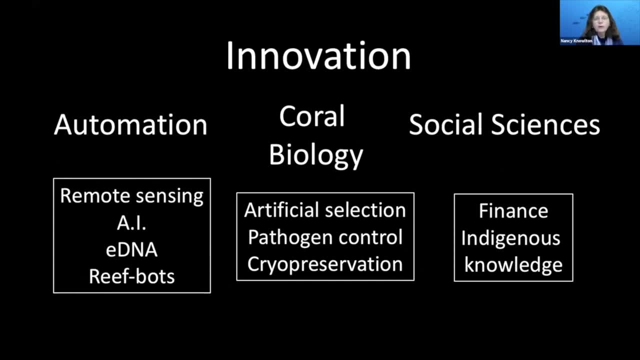 And I'll say a few more words about that shortly. And then, in terms of innovation, there are so many ways you can talk about it. These are just a few. In one case, there's the whole potential offered by automation in things such as remote sensing. 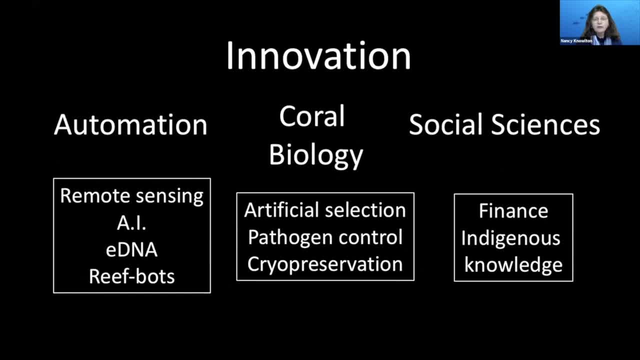 and artificial intelligence, eDNA and reef bots- machines that run around helping reefs without much human attention. And automation is important because a lot of the traditional ways of conserving coral reefs are relatively labor-intensive and automation helps that process. Then we're making also enormous progress. 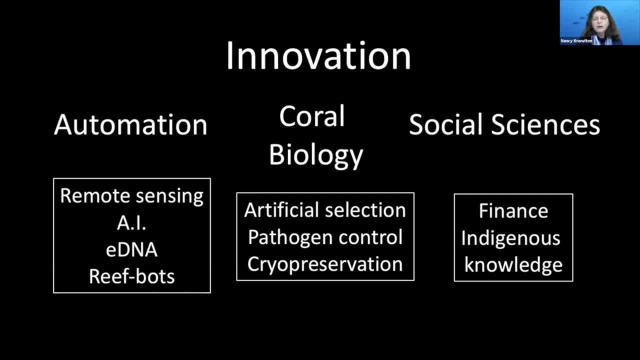 in terms of our understanding of coral biology And how to use that understanding to help make corals more resilient and more resistant to human impacts, And these range from everything, including things like artificial selection, control of pathogens to treat diseases which remain a very serious problem on coral reefs. 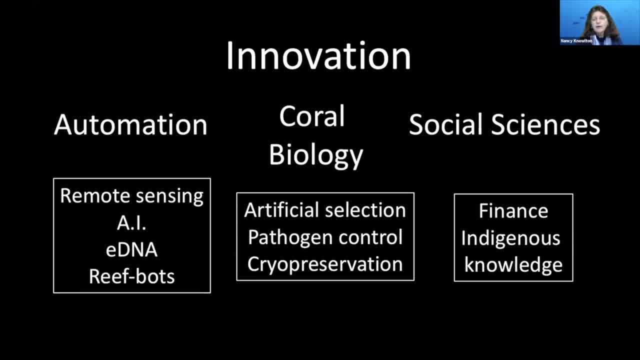 and even cryopreservation to freeze coral gametes, not only so that they're available in the future, but so that they can be used in artificial selection experiments in the present. And then, finally, there are a lot of innovations in the social sciences involving finance. 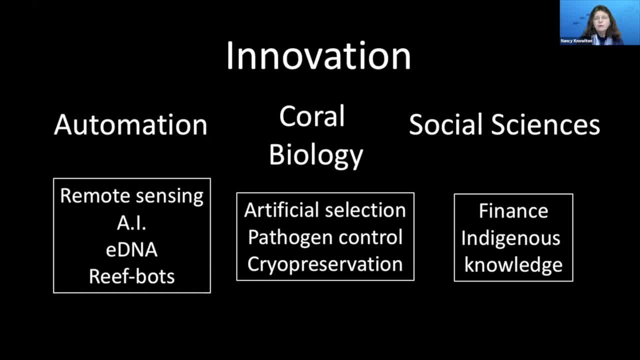 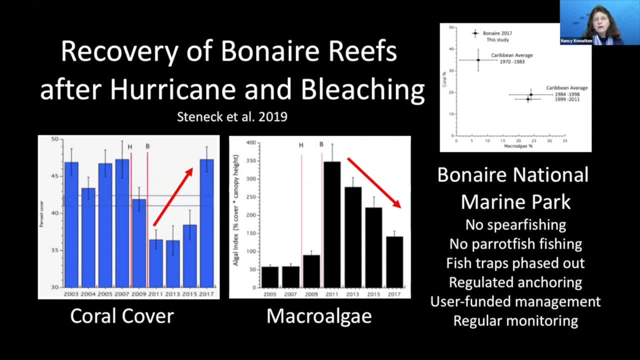 and also indigenous knowledge. So let me just give you a few examples, And the first example I want to give you is from Bonaire, which is an island in the Caribbean, And I think it's important to talk about the Caribbean because it's often viewed as the basket case. 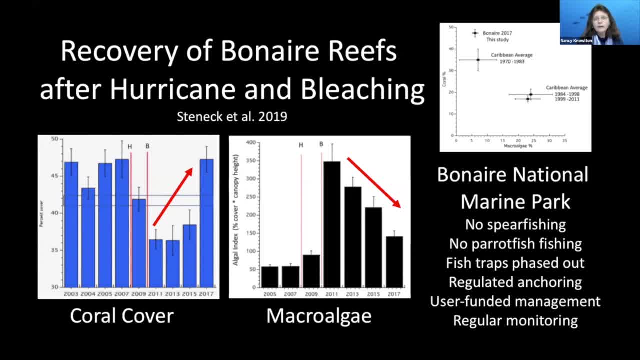 of all coral reef regions, because so many of the reefs look like that picture of Jamaica after the collapse of the reefs. And yet this is a really interesting study published recently, in 2019, by Bob Steneck, on the recovery of Bonaire reefs. 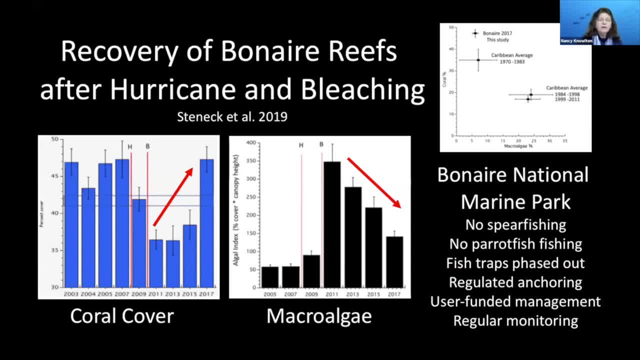 after both hurricane and bleaching events. So what you see here is under coral cover. the hurricane occurred just before 2009, and the bleaching event occurred just after 2009.. And so you can see these reefs were holding their own. They suffered from those two events. 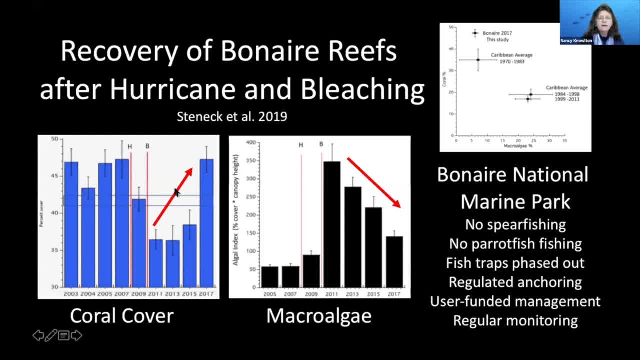 but then since 2011,, they've been on a steady increase. So coral cover is going up And in a similar way. here again, you see 2009, bracketed by a hurricane and a bleaching event, a big increase in macroalgae and then a decline since then. 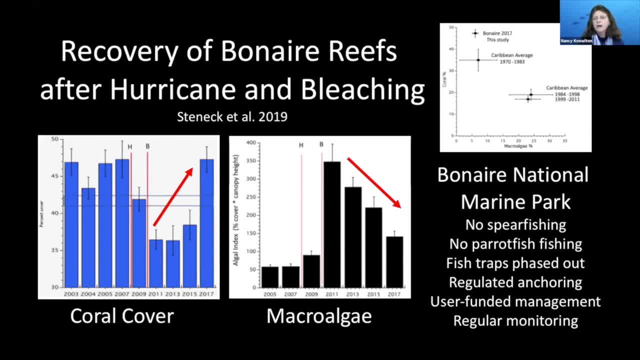 So why is it that Bonaire is doing so much better than many other Caribbean reefs? And it's because they've taken a number of steps to really protect their reefs. The entire coastline is in a marine protected area, but it's not a no-take marine protected area. 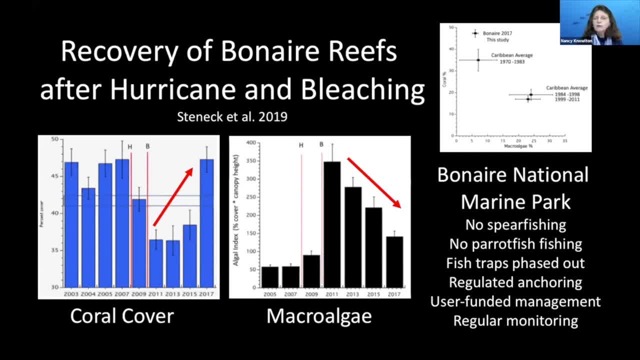 at least in totality. However, there's no spearfishing, there's no parrotfish fishing, which are very important for keeping macroalgae well-grazed. Fish traps are being phased out. Anchoring is very highly regulated, All the activities associated with protection. 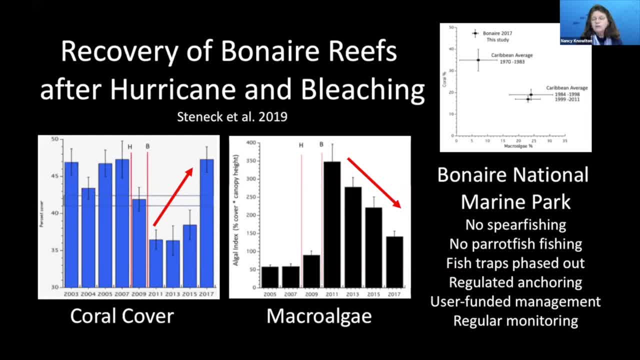 are funded by users via fees to enter the park and there's regular monitoring. So these are parts of the elements that Bonaire has used to really create a success story in coral reef conservation. And then the upper right, you can see a plot that compares. 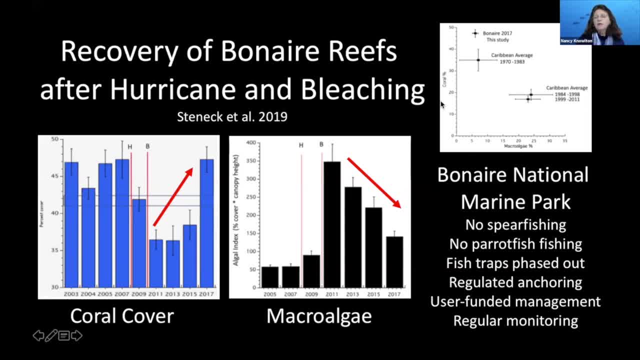 algae on the horizontal axis with percent coral cover on the vertical axis. And here you see what coral reefs used to look like: Lots of coral and not much algae. And over here is what most Caribbean reefs look like. But up here is what Bonaire looked like just recently. 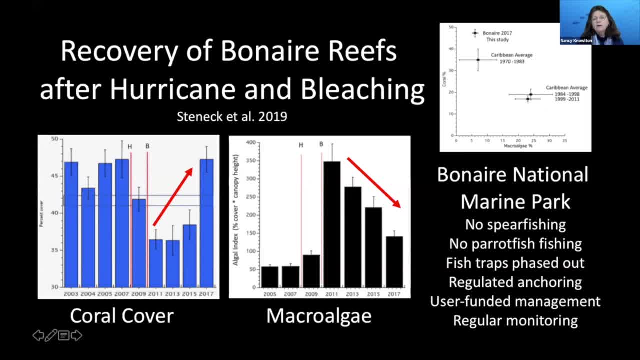 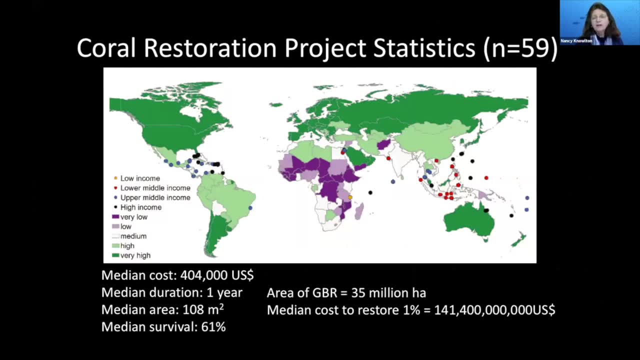 So this really is a success, And there's no reason that this kind of success couldn't be replicated anywhere in the Caribbean or, for that matter, on any coral reef around the world. I want to say a few words about coral reef restoration, because it's getting a lot of attention. 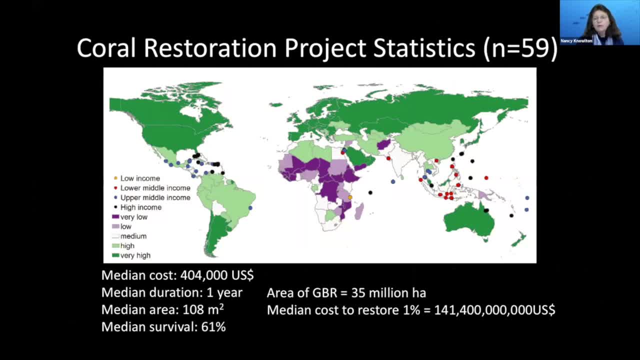 As I mentioned, because so many corals have died, people have turned to restoration as a way of stemming the losses and reversing the losses Now. a recent analysis suggested that the median cost of restoration was about $404,000 per hectare. 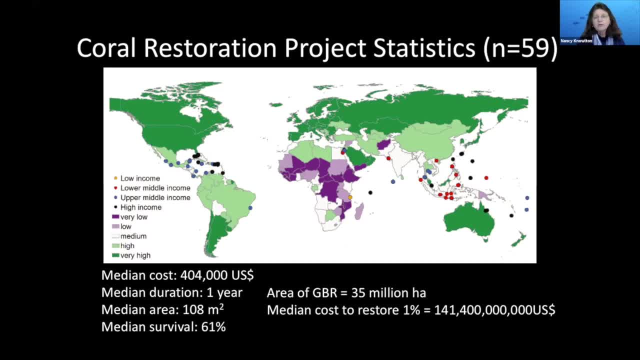 which is a pretty large coral, So that's a lot of cost, And also that these restoration projects, which had been where the results have been published, typically the results were only reported for a year. The median area covered was tiny, 108 meters square. 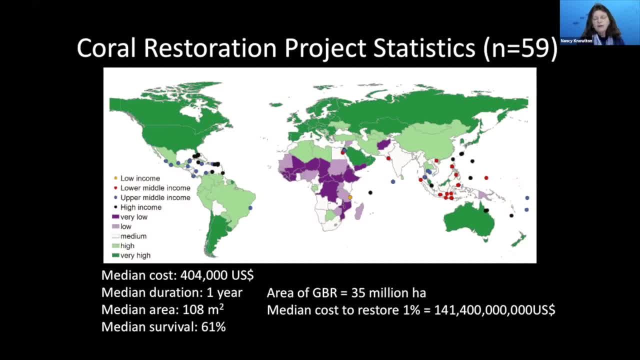 And the median survival was 61%, And that's just after one year. So if you consider the fact that the Great Barrier Reef is 35 million hectares and you wanted to restore just 1% of it, that would. you're talking about something. 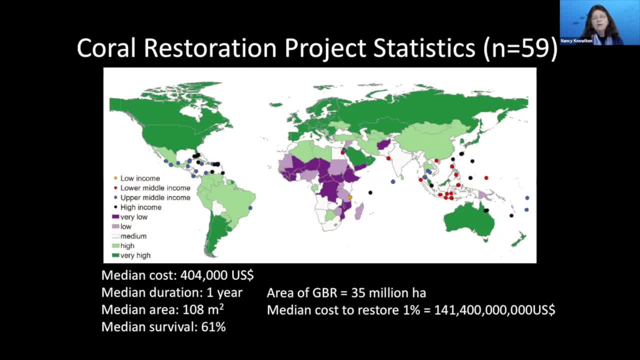 like $141 billion US. So that's really not what coral re-frustration is about, And I think it's important to separate these average statistics from the roles where coral re-frustration can be important, And I want to give you one example of this. 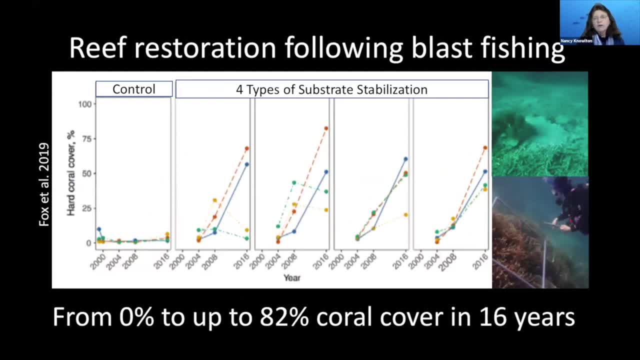 This is work by Helen Fox, who worked on restoring reefs in Indonesia after blast fishing And the places they were working. the regulations prohibiting blast fishing and blast fishing were improved, And so the destruction was enormous, But then the source of mortality was eliminated. 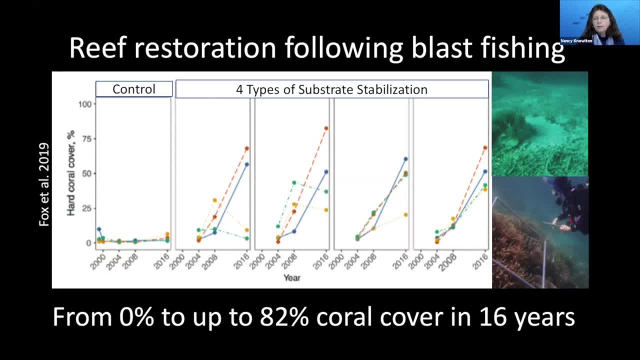 And what they did was. But the problem with blast fishing, as you can see in the upper right, is that it creates. I'm not sure if it's revealed here by the or covered by the pictures of people's faces, But there's a. 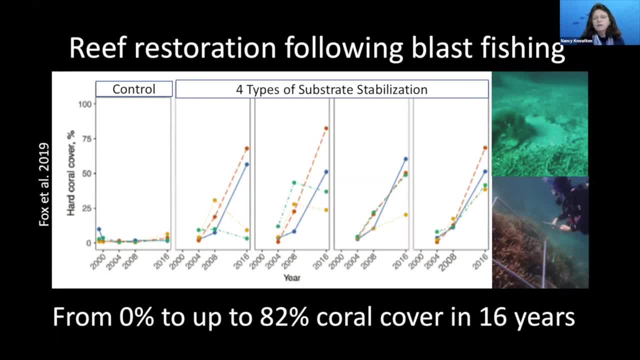 Blast fishing essentially pulverizes corals and creates a very unstable habitat, And so it's very hard for corals to recover. And, as a result of their work, which involved four different types methods, strategies for stabilizing the substrate, they documented that in the control area. 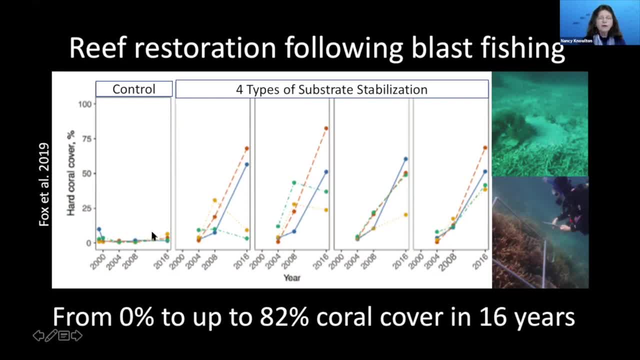 where they did nothing, there was essentially no recovery and that's what you see here. But in these various areas where they stabilized the bottom and essentially tied down the loose substrate so it wasn't rolling around, they went from 0% to up to 82% coral cover. 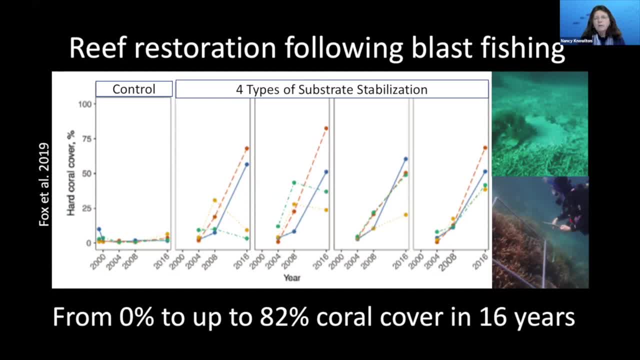 in just 16 years. So this is an example where coral re-frustration really makes a lot of sense. In this particular case, they didn't even bring in live corals, They just used natural recruitment to have a recovery take place. 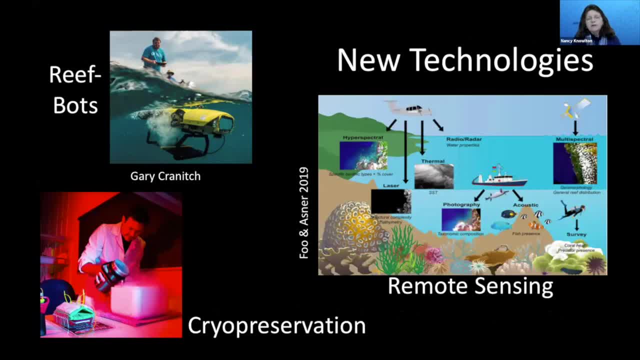 Say a few words about A few words about new technologies. There are a lot of these. Some of them involve remote sensing. As I mentioned, coral reef monitoring is typically very, very labor intensive, So there's been a lot of developments in terms of imaging. 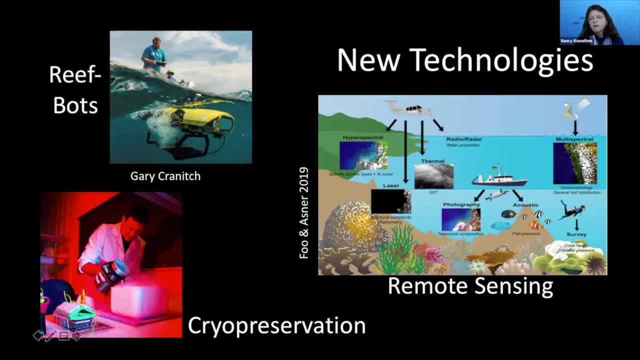 and also even with photography, which can be very labor intensive, not so much in the taking of the photographs but in analyzing the use of artificial intelligence. I mentioned before these reef bots. Here you see one that's used to spread baby corals over the coral reef. 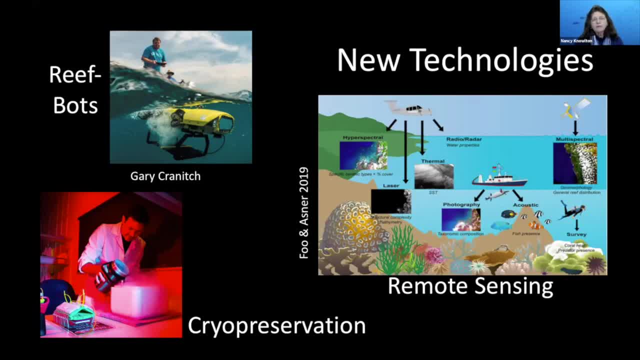 And there are other versions of these reef bots which can find crown of thorns, starfish, which cause a lot of mortality on the Great Barrier Reef, and inject them with vinegar to kill them. And then on the lower left you see here the cryopreservation. 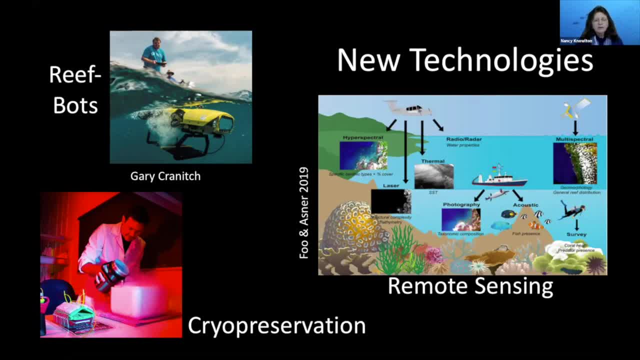 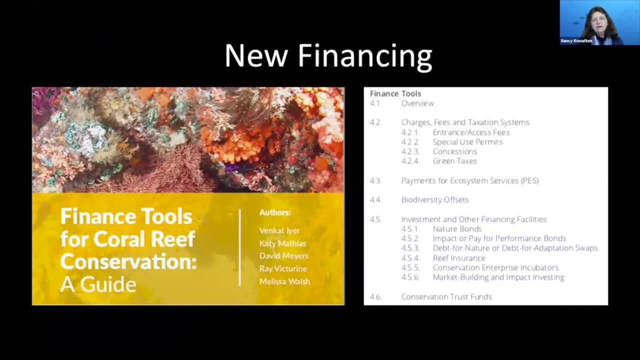 which is now based on what's being used to successfully store sperm of corals, to be used both in the future and in the present, during artificial breeding experiments. And then, finally, I'd like to say just a few words about the new financing tools that are available. 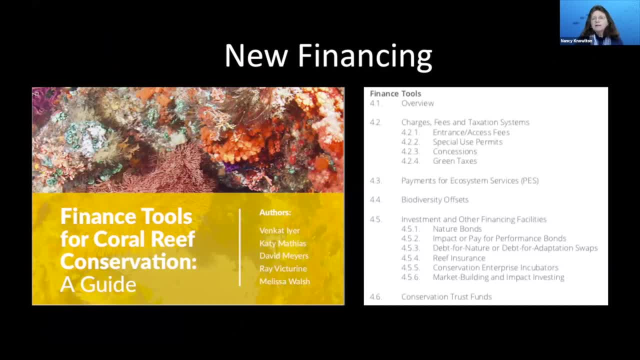 And you see these here summarized on the right. Some of them are relatively traditional, such as charging fees. That is in fact what the Bonaire government does to support the activities of conservation. They charge people to enter the Marine National Park. But then there are other things like reef insurance. 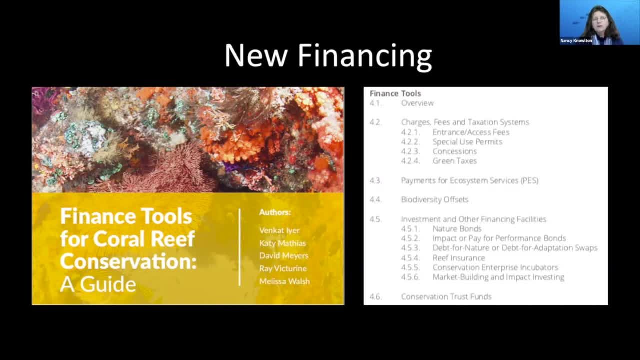 which has been used now in the Caribbean to help finance reef protection on Mesoamerican Great Barrier Reef, and also debt for nature swaps, which has just been used by the Nature Conservancy, along with other organizations, to create a vast marine protected area in the Seychelles. 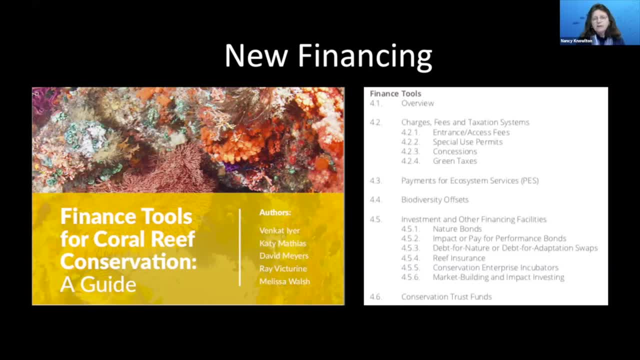 So there are lots of innovative financing methods that are being developed, as well as these innovative more science and technology side of things. So that's really all I have to say for now. I'm happy to take questions about any aspects that I've talked about. 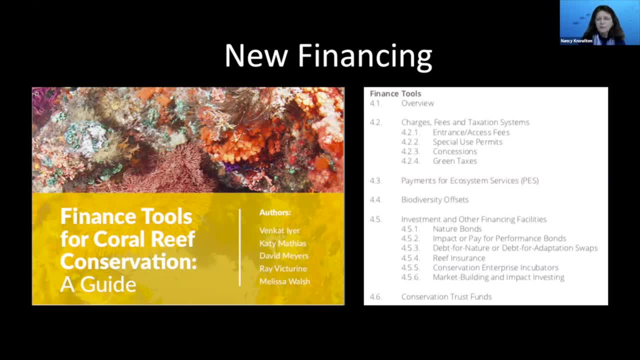 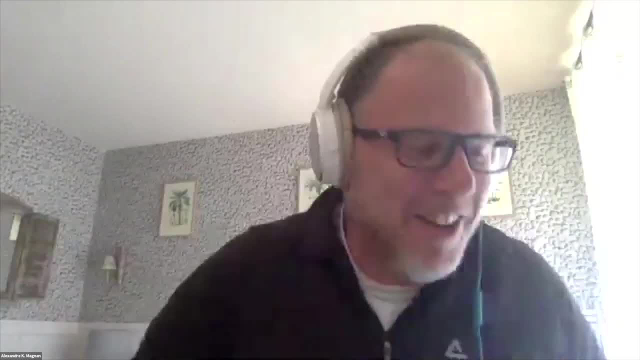 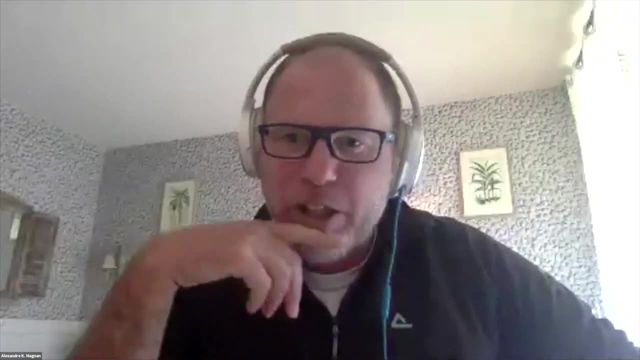 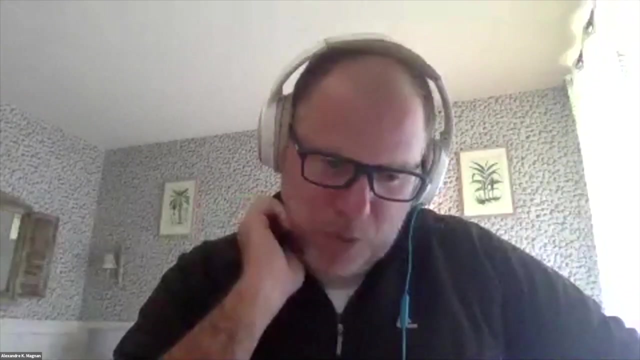 or anything else about coral reefs for that matter, Thank you. Thank you, Nancy. Yes, a lot of questions Again. not easy to synthesize all, But if I try to come up with some overarching points from the questions, this is interesting to dive into one single example. 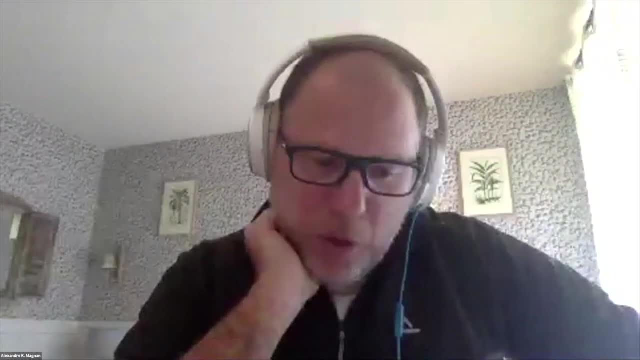 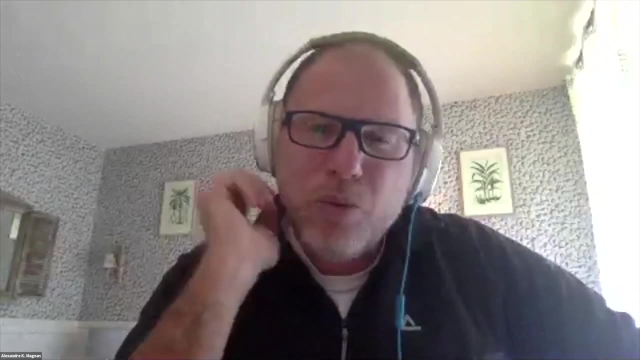 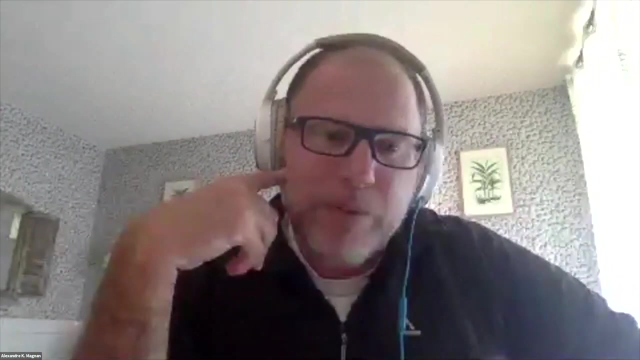 one specific species. that helps going further in terms of the detailed question we can ask about restoration and what we can do. Two different kinds of questions very quickly. One is about the natural capacity of coral reefs to do their job actually, because we see that in your presentation. 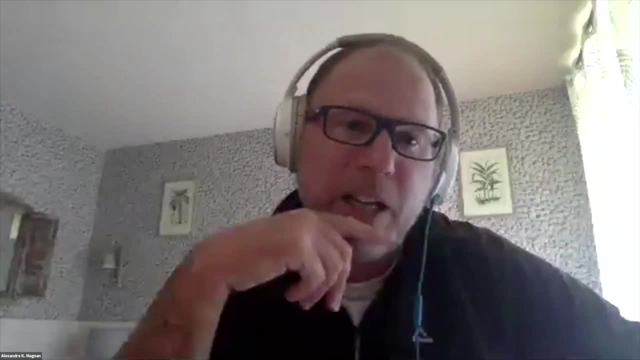 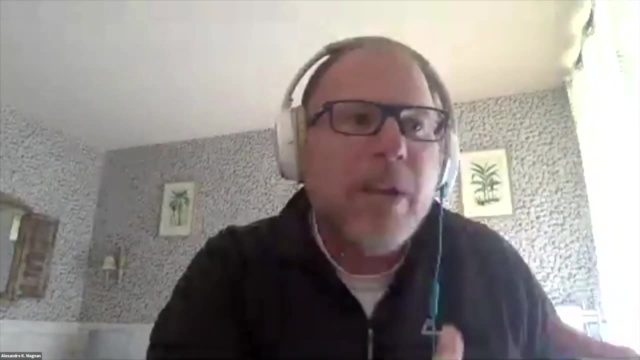 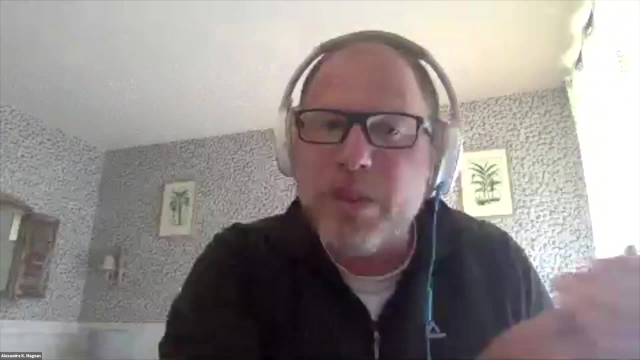 that human societies can do a lot, actually can achieve a lot. But the first question is also okay: and is it enough? That means: do the coral reefs still have the capacity to adapt and to cope with changes, especially because we all know they have? 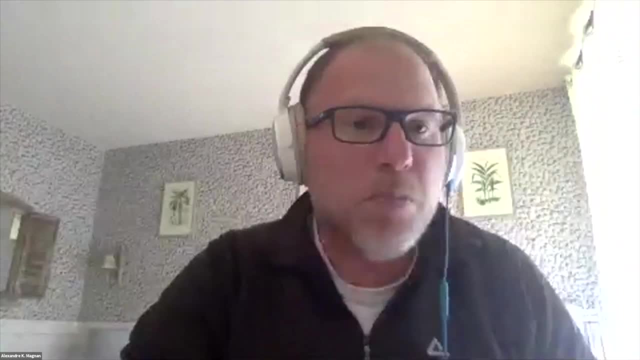 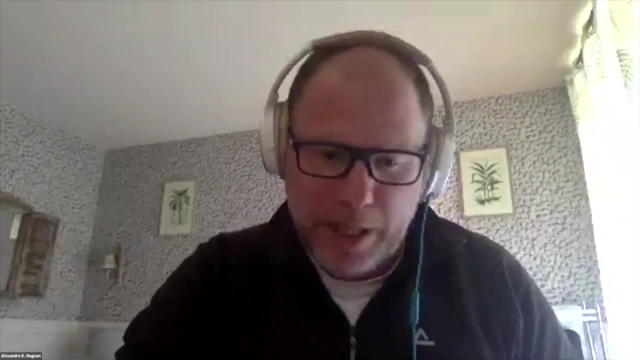 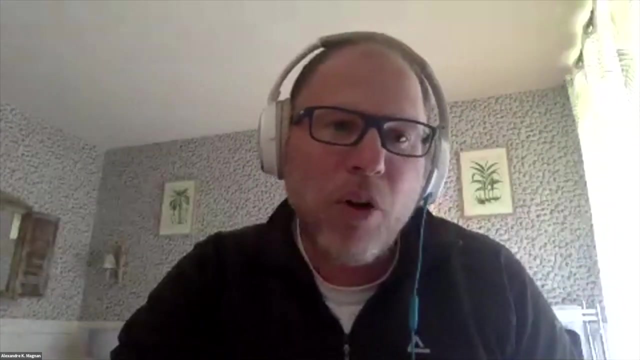 and they are still now recurring huge, bleaching events. So this is the first part of the question, the natural side, And on the other side some questions related to these finance issues. You show that at the national and local level we can find ways to develop. 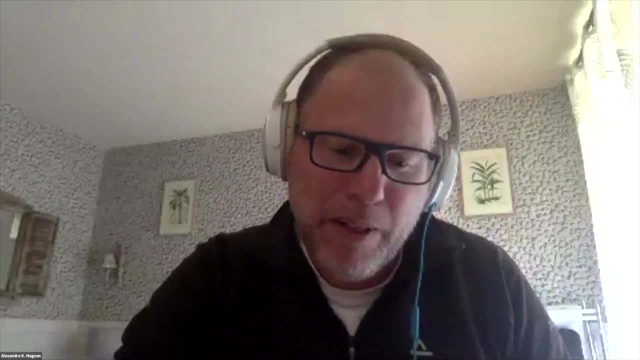 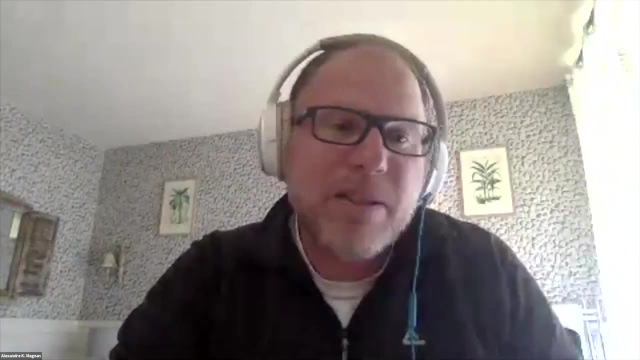 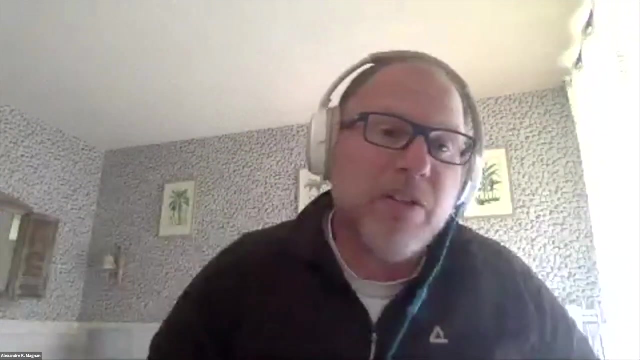 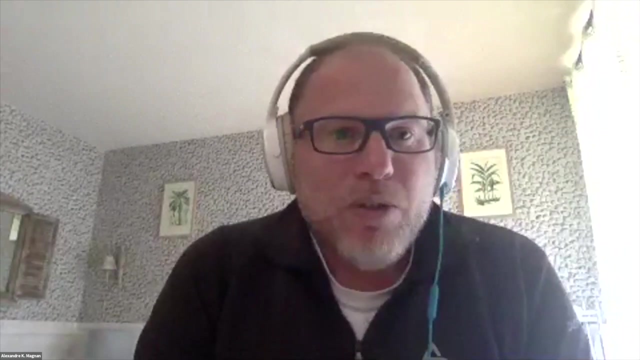 some financial instruments to help reef protection, But again, is it enough, To what extent a given country can do it by itself, Or what is the role of regional and international organizations, financial bodies or multilateral cooperation and so on? So sorry, two long questions. 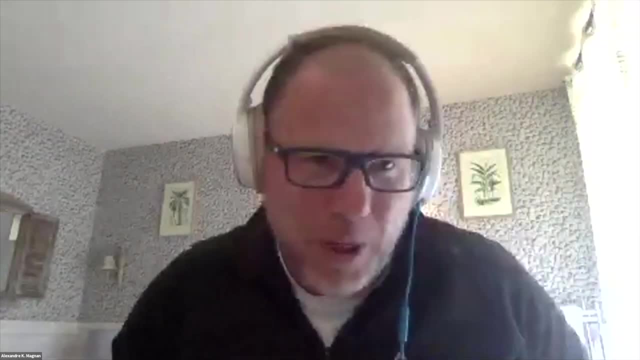 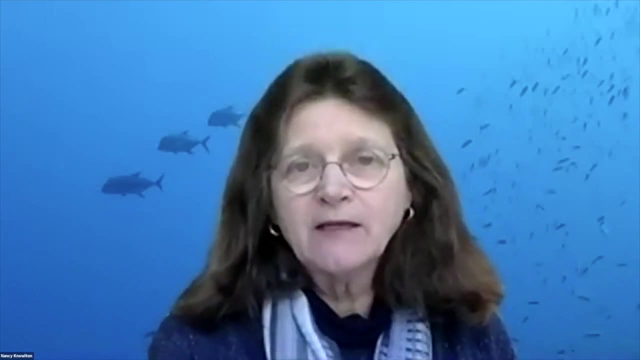 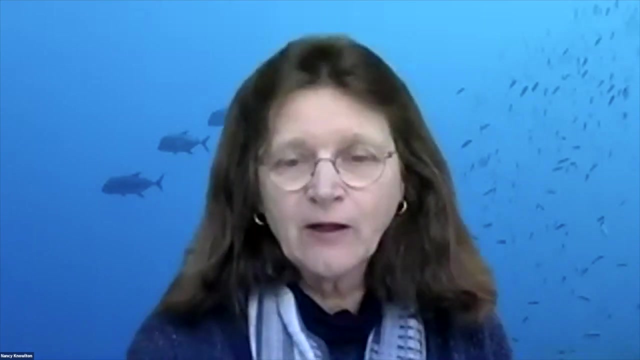 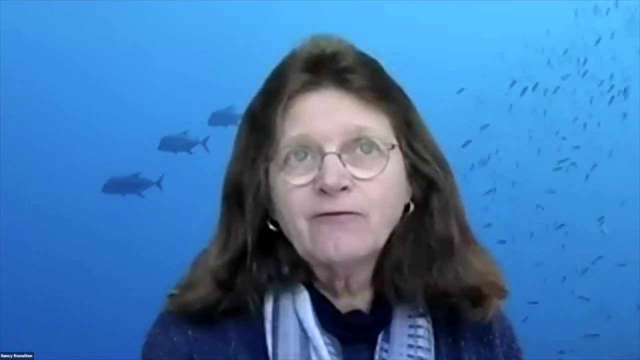 but two quick answers. The first question had to do with what was the capacity of coral reefs to make it on their own, For example, if humans just relaxed pressures? in terms of the immediate environment, The study of Helen Fox's showed that in a place where the only problem was, 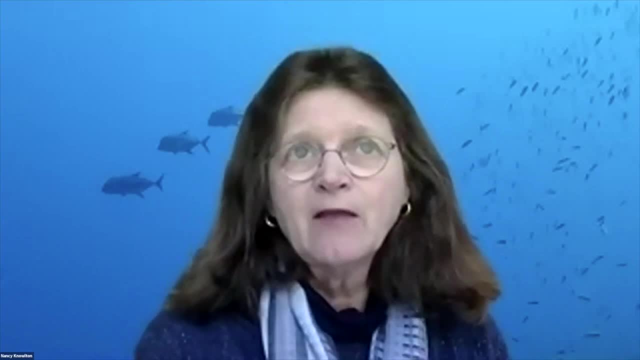 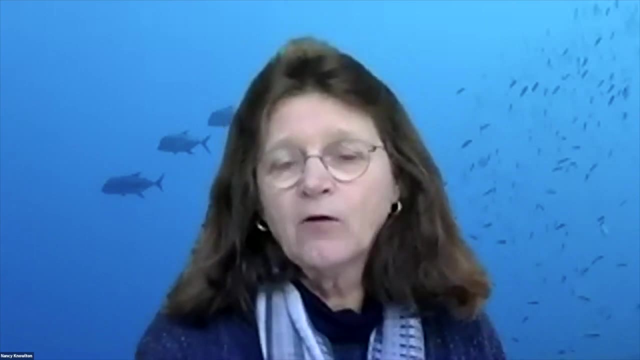 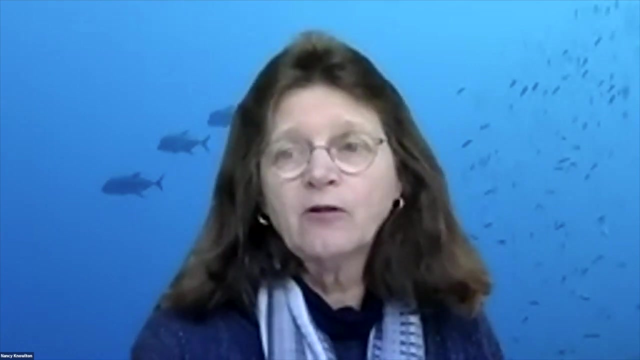 a specific disturbance, which was then stopped then. actually, reefs are pretty capable of bouncing back, and actually remarkably quickly, And that's because a lot of the corals that grow on reefs actually grow relatively fast. Not all of them- The big head corals- grow very slowly. 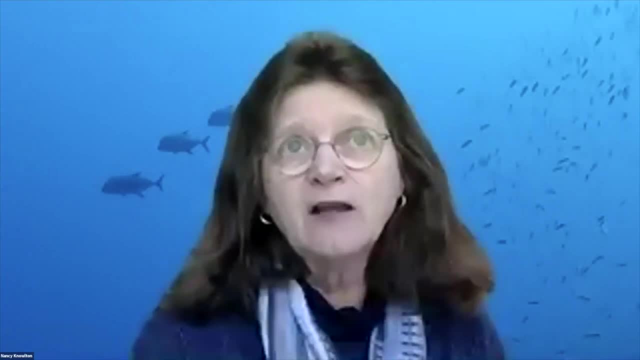 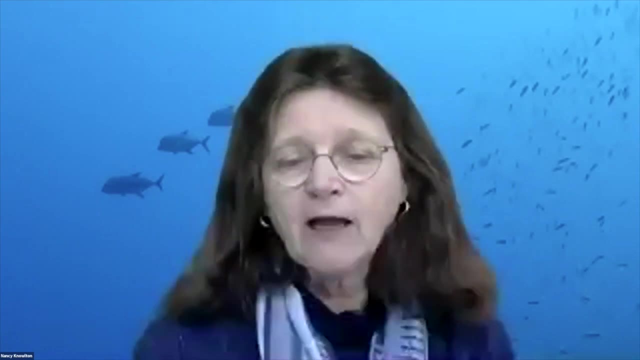 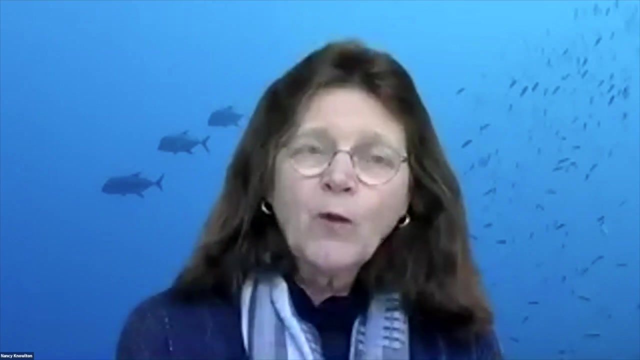 about a centimeter a year. The branching corals grow about a centimeter a month from their branch tips, So they can actually recover pretty quickly once they get going. But the second question, if I understood it correctly, has to do with whether coral reefs 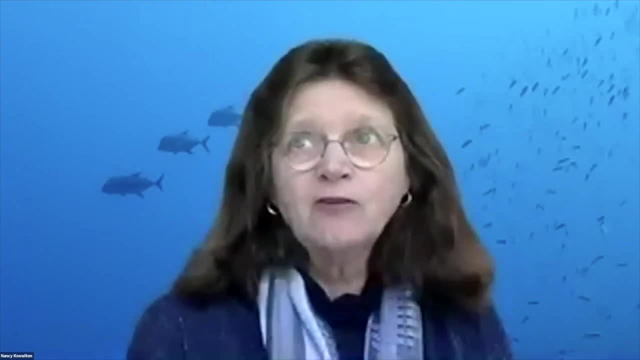 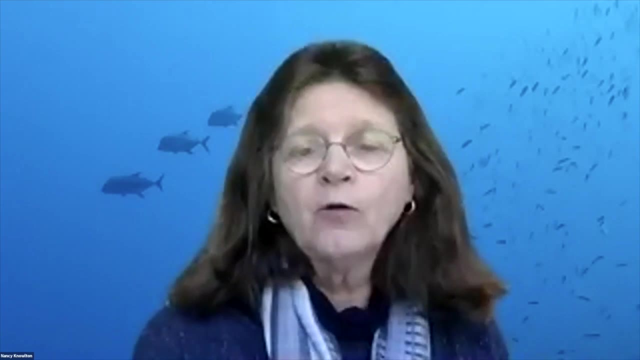 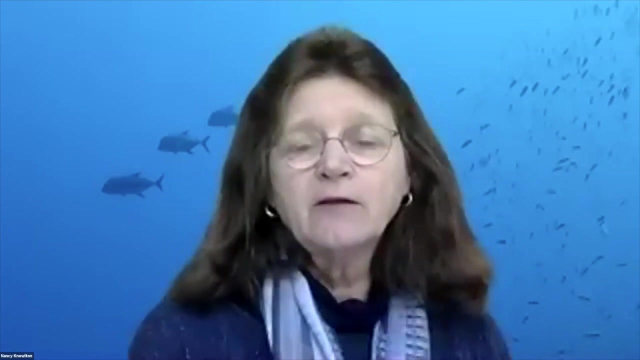 can adapt to the changes in climate And we know on some time scale that they can because, for example, coral bleaching doesn't happen at a fixed temperature. It happens when the local temperature exceeds the normal average by about one degree centigrade. 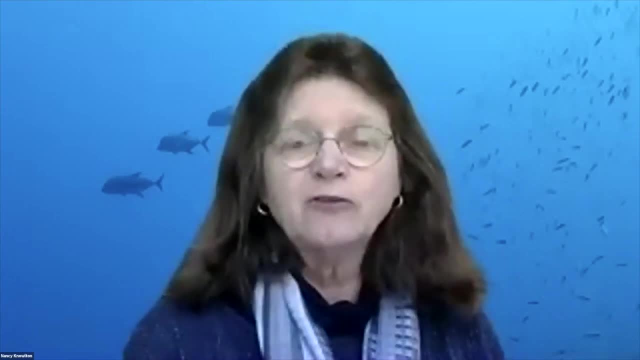 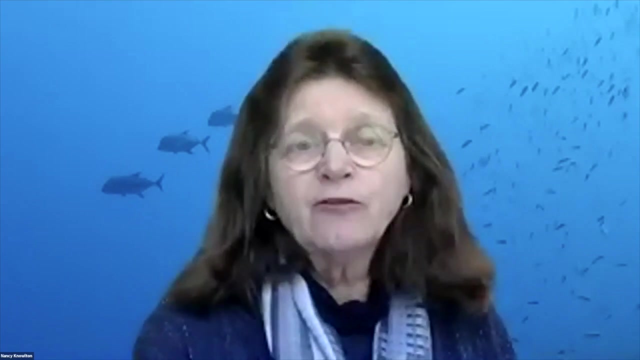 So that tells you that the corals have adapted to their local thermal environment. The problem is that the rate that we're changing global temperatures and also, for that matter, global pHs, which I haven't talked about at all, is much faster than corals are usually experienced. 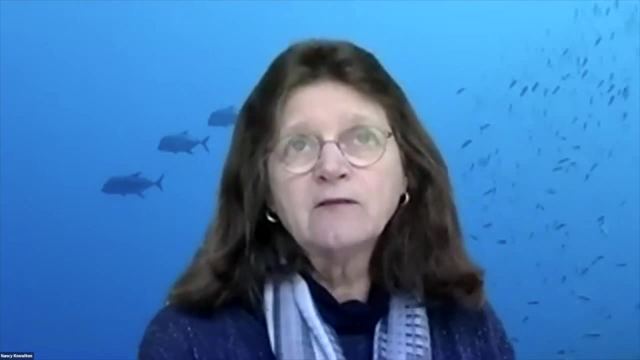 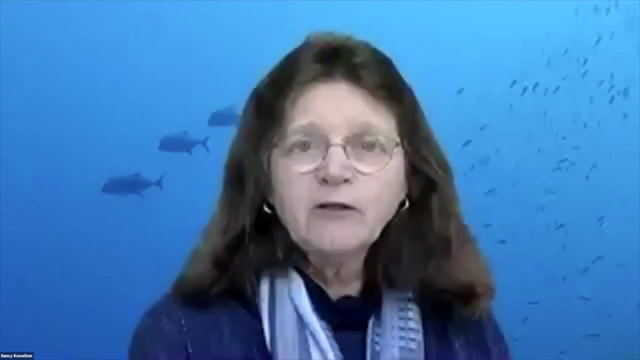 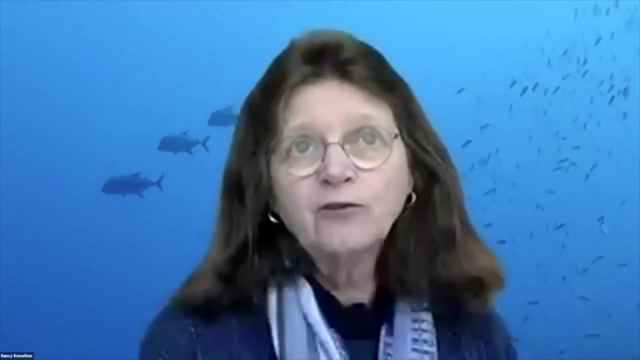 And that's why there's been a lot of interest in artificial selection, even genetic evidence and engineering. The idea is- the term is called assisted evolution And the idea is to jumpstart the ability of the corals to evolve to be better suited to the conditions. 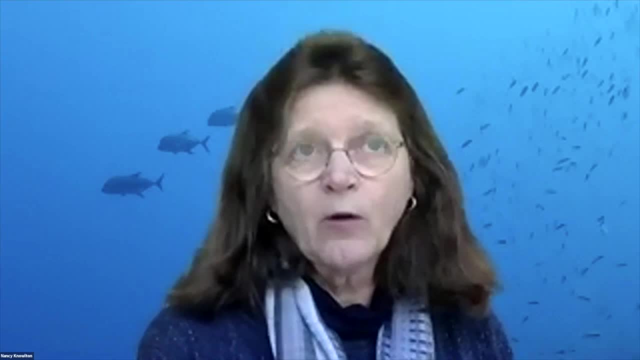 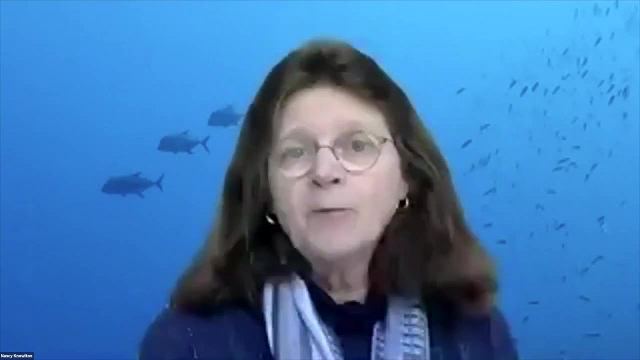 that are likely to prevail for some time, even no matter what we do in terms of addressing climate change. It's not going to be a quick fix, And so I think the answer is it really depends on the coral and depends on what you're at. 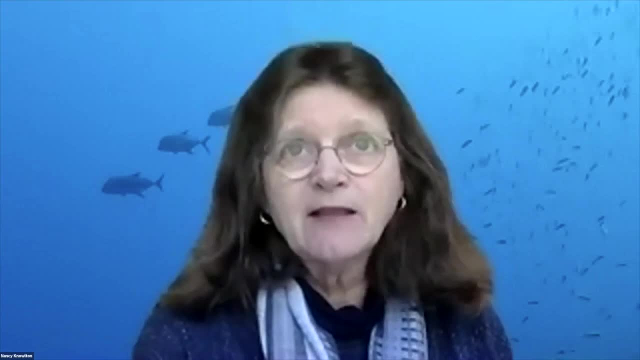 the actual threat that you're talking about. In some cases, I think the coral reefs can, if we take away the pressures, restore healthy fish communities, have clean water, the Bonaire example being a really good one, also Helen Fox's example. 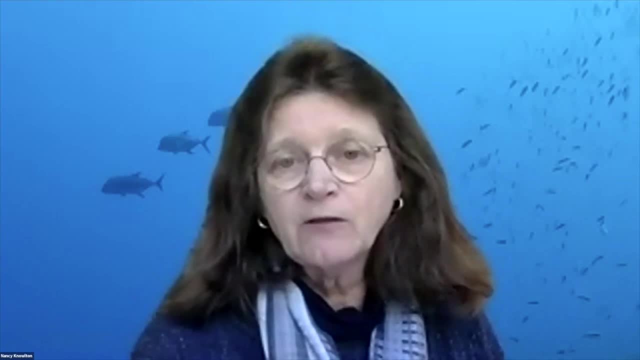 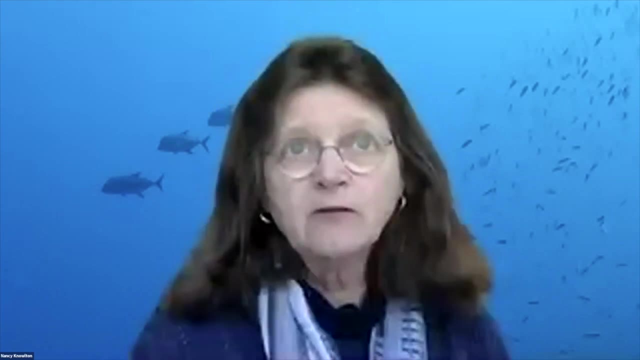 in terms of ending dynamite fishing, the reefs actually are doing pretty well, And that's good, because it's expensive- Restoration of any sort is expensive, But on the other hand, there's some elements of what corals are likely to face where they probably do need our assistance. 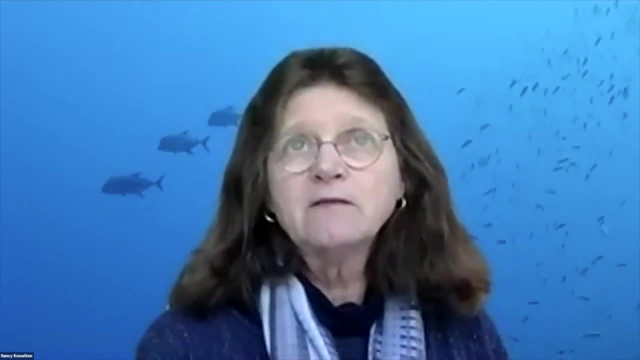 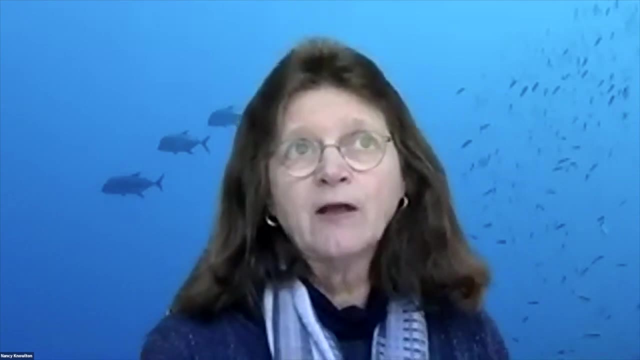 And I think, even though it's expensive and uncertain, I think it's important to look at what, say, humans have done with agriculture and selection, in terms of the plants and animals that we use, to realize that we have done a lot, And technology in general. 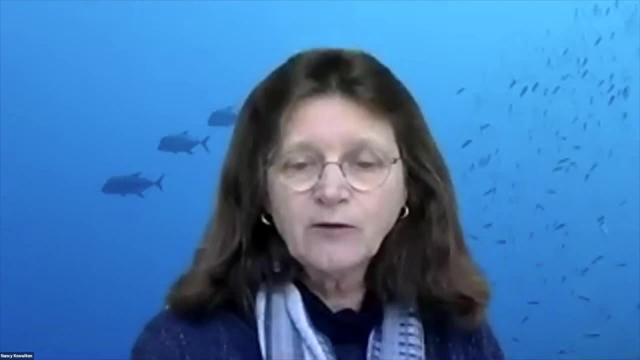 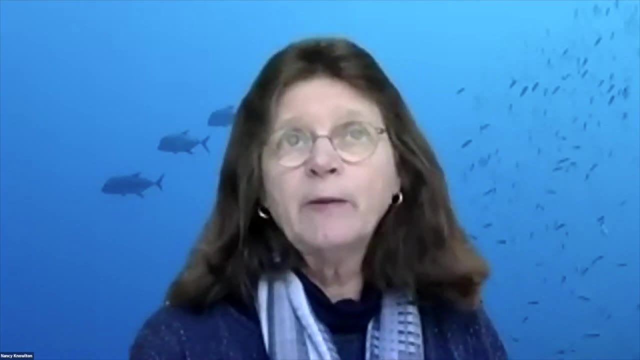 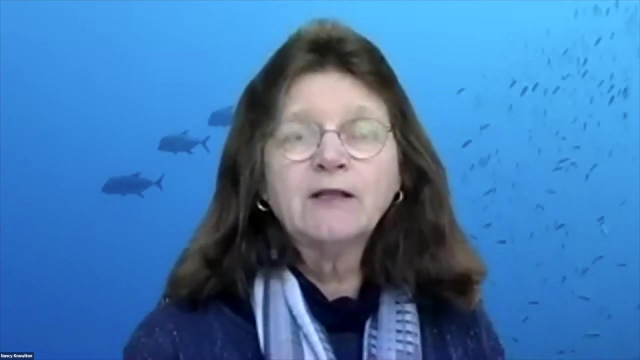 think about what has happened, say, to the price of solar power. So to simply dismiss technology and say it's too expensive and it's not fast enough, I think flies in the face of what technology has given us in terms of benefits over the last, say, five decades. 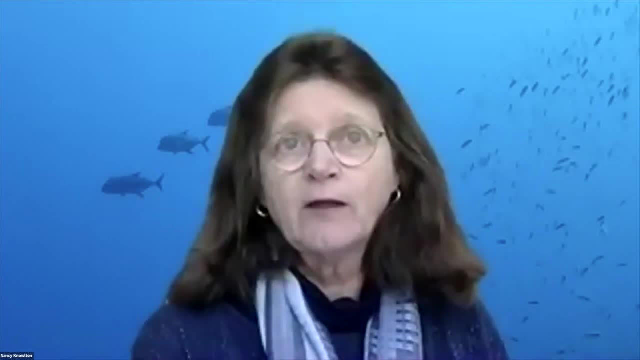 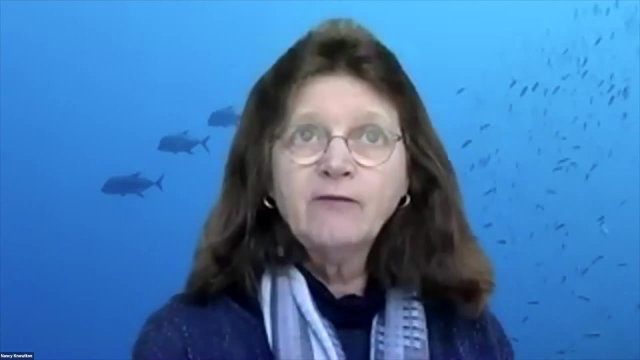 That said, technology on its own is not enough, And that's the point, And I will return to that point again and again. Addressing climate change, addressing habitat quality and investing in technology are all parts of the solutions that we need for coral reefs. 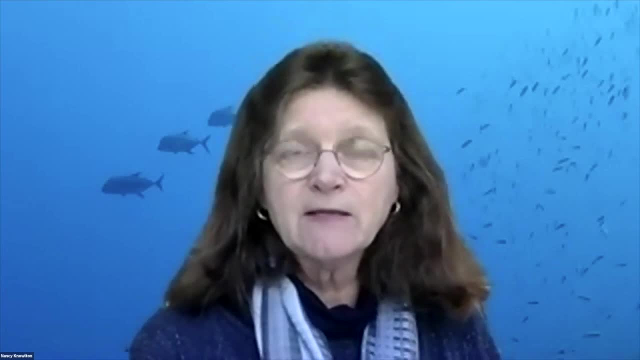 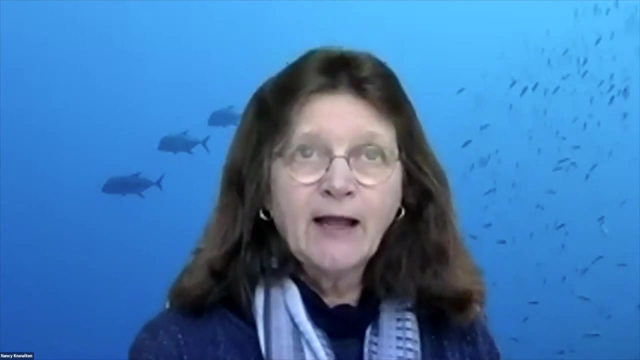 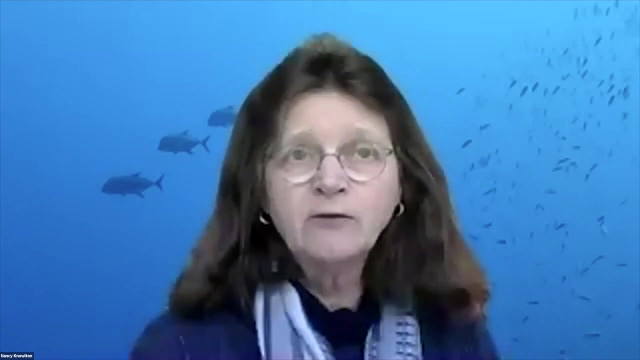 In terms of the financial mechanisms, again, it depends on the setting and the scale of what you're trying to do. In Bonaire, it is a national action where the user fee to enter the park actually is administered by an NGO, a non-governmental organization. 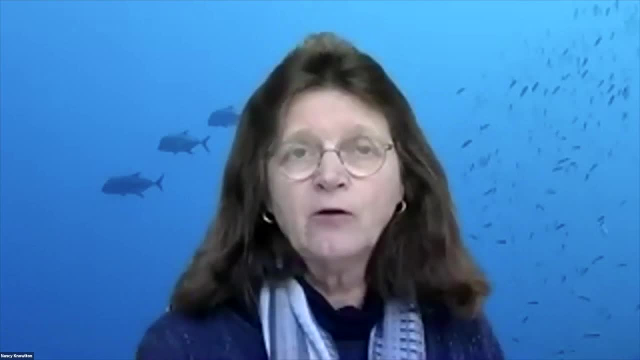 So it's a partnership between the government of Bonaire and the NGO. In the case of the Seychelles, it was a relationship between the Seychelles government and the Nature Conservancy and, I believe, the Leonardo DiCaprio Foundation. 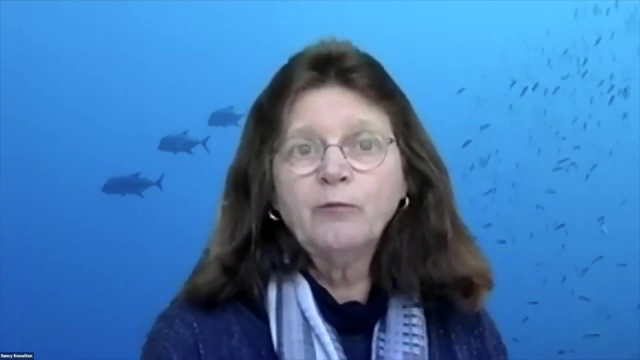 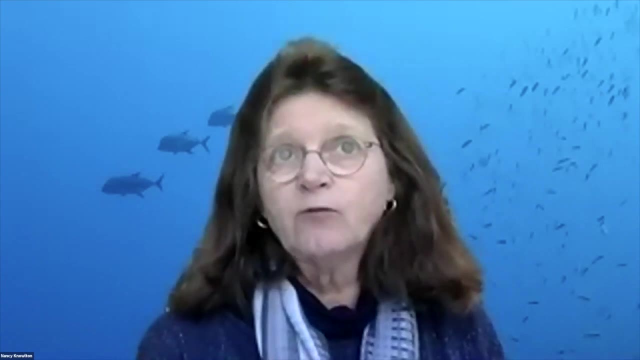 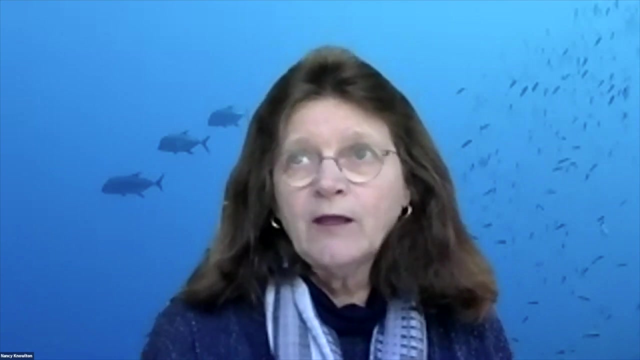 and a number of other players. It was a very big financial deal, much bigger than, say, the scale of the Bonaire financial arrangement. So it does depend on the scale of what you're trying to attempt And I think that really. 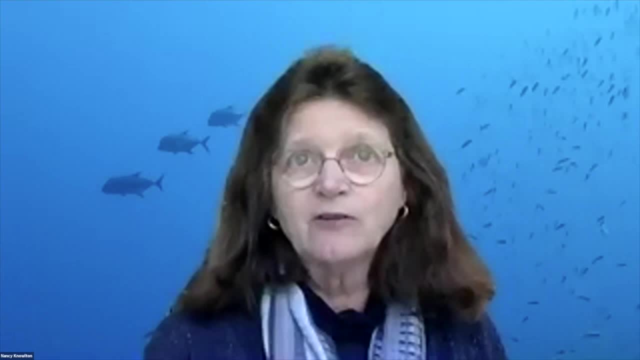 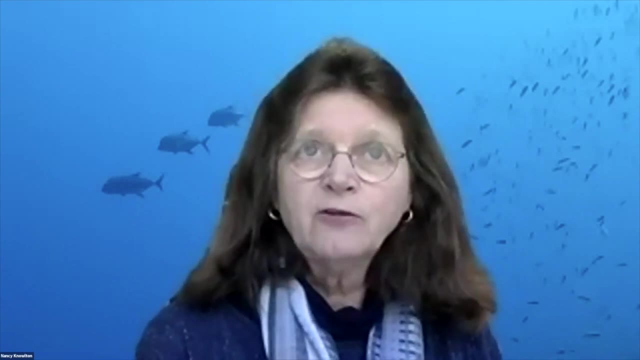 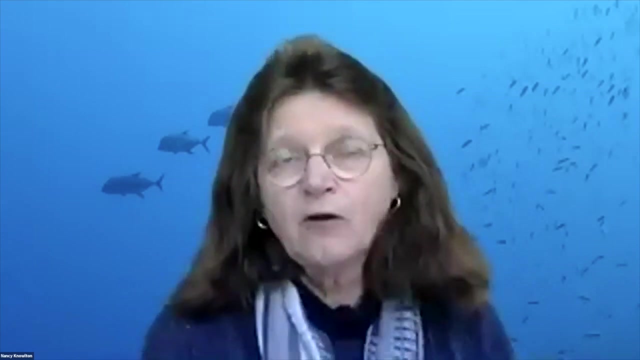 we need all hands on deck when it comes to coral reefs. The situation is dire. So everything from local communities working to preserve coral reefs to international agencies working to coral reefs, all of those partnerships and participations are important. Thank you, Nancy. 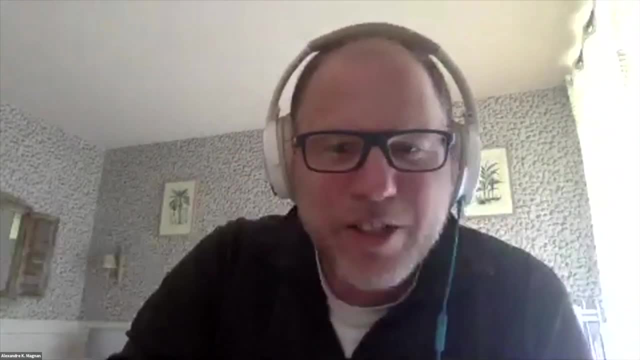 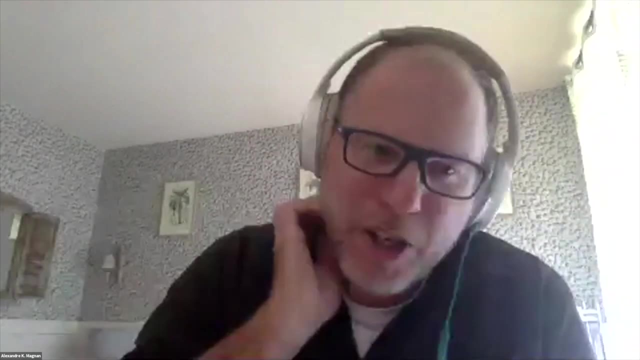 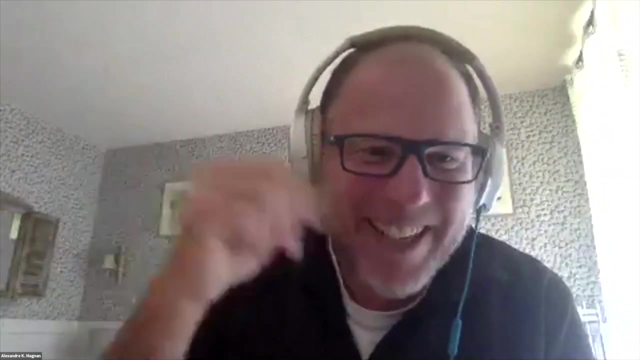 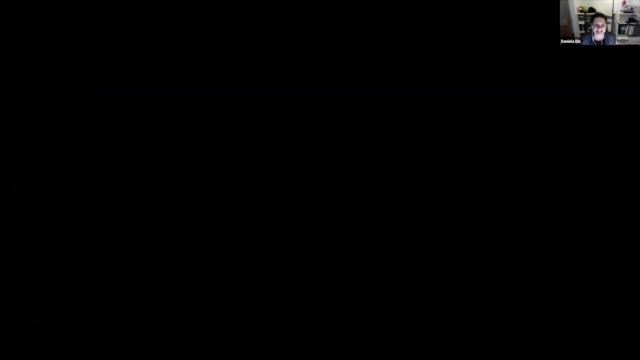 This helps understand the challenges, not only on the natural side, And Daniela will take us to these human-related challenges. So how to govern this? Daniela? please, Sure, give me one second. OK, nice, Can you see? 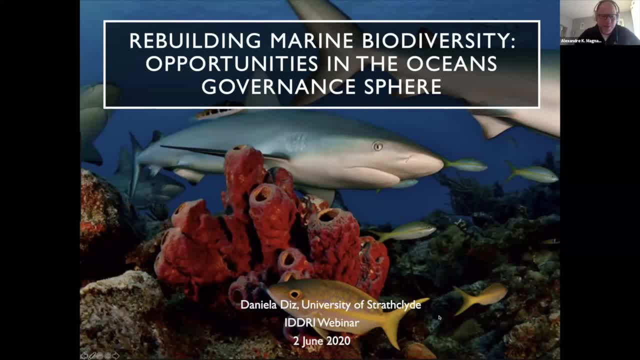 Yeah, we see your screen and we can hear you. Great, So yeah, Hi everyone, Good afternoon, Good morning, Good evening, wherever you are. I'm going to complement those fantastic presentations by Jean-Pierre and Nancy by talking about the governance sphere. 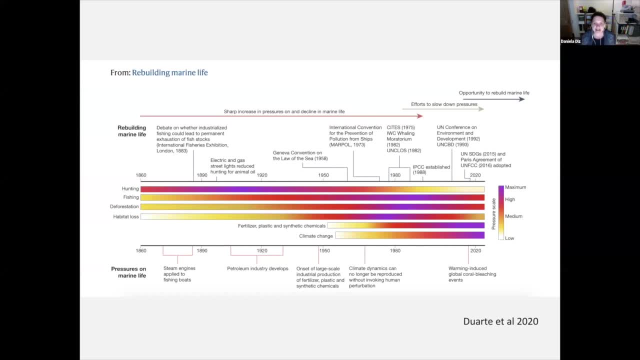 I'm starting with this graph, very nicely presented in the paper by Duarte et al. Both Nancy and Jean-Pierre were authors, but I'm not going to address all of those instruments because there are too many for a 20-minute presentation, But I'm going to focus. 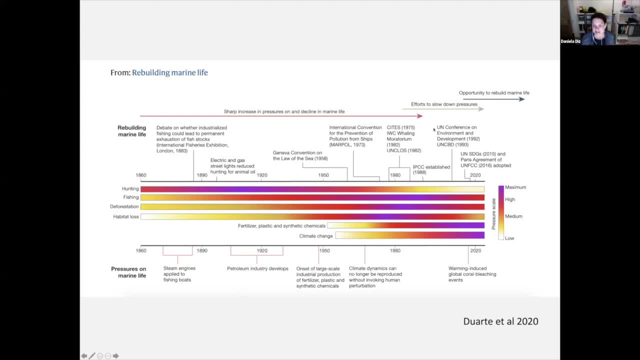 on the Law of the Sea Convention, the Convention on Biological Diversity, the SDGs. of course There is an interface with the Paris Agreement and all of that and some other ones as well. So I'll just start with the Law of the Sea Convention. 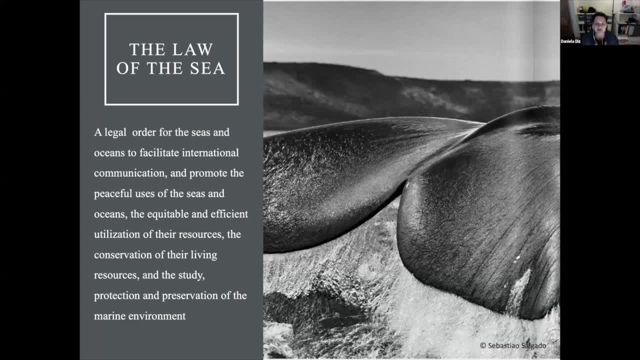 just because it's considered the constitution for the oceans, And I need to allude to that because it's, you know, has been considered by member states of the UN as the framework convention that regulates all activities at sea. Of course, not directly. 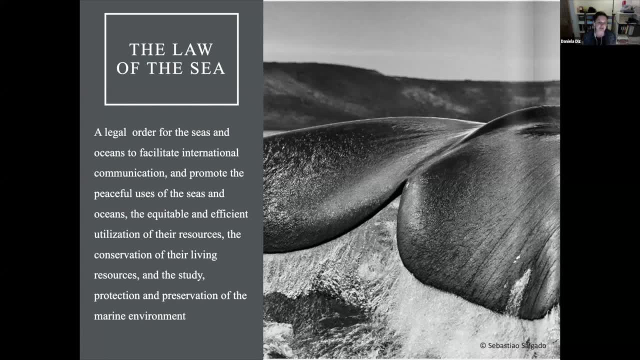 but it sets general obligations And its objectives is really to establish this legal order for the seas and oceans, to facilitate international communication, promote peaceful uses, equitable and efficient utilization of the resources and the conservation of the living resources, study protection and the preservation of the marine environment. 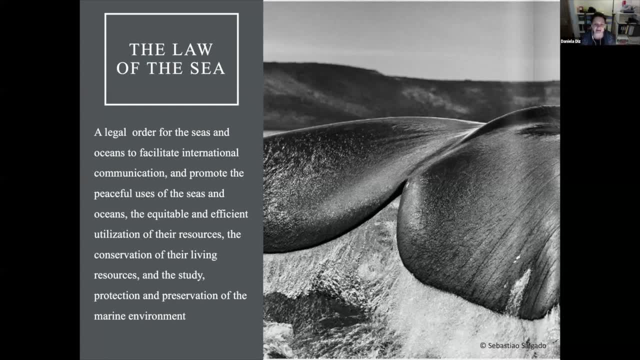 So, with this in mind, of course, not all UN member states are parties to UNCLOS and not all CBD Convention on Biological Diversity member states are parties to UNCLOS, So this needs to be considered throughout the discussion. But a number of its provisions. 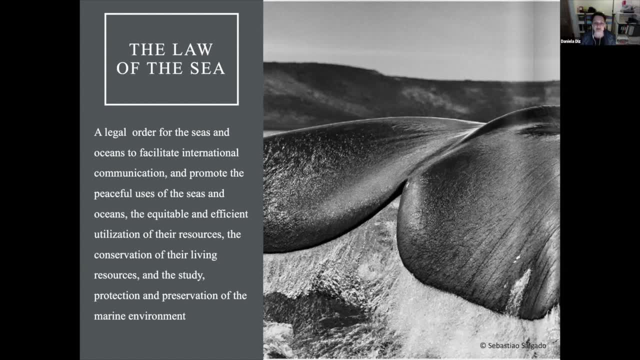 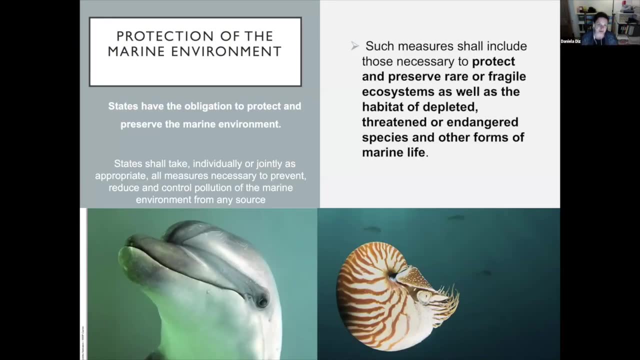 including around the protection of the marine environment has been considered rules of customary law, So it's applicable also to non-parties just to an extent. So in its part 12, UNCLOS, the Law of the Sea Convention, talks about the protection. 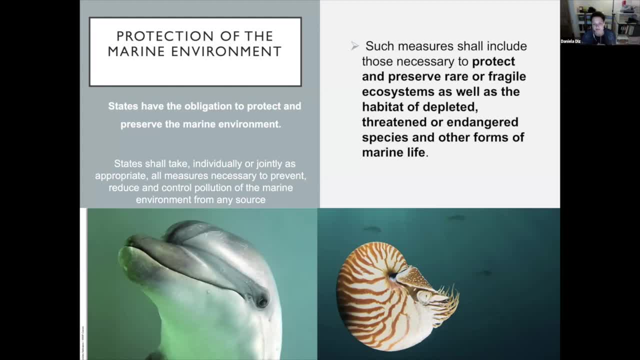 of the marine environment. It's part of the convention that's focused a lot on marine pollution, but it's not only about marine pollution. There has been decisions by international tribunals saying that that part also applies. the protection of the marine environment entails other uses as well. 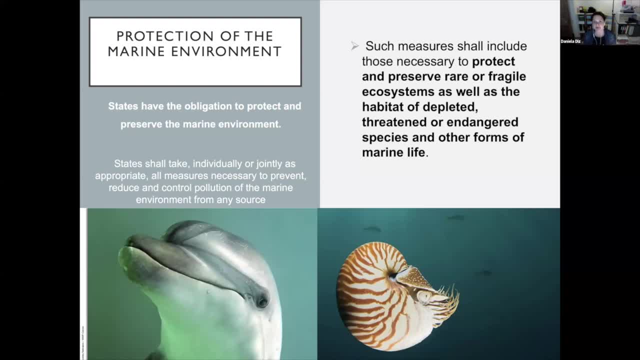 other pressures, but it's very focused on pollution And one particular provision that I'd like to focus because it will take us throughout this presentation today. sorry, what happened here, Apologies, It's this one: that measures taken, that states shall take. 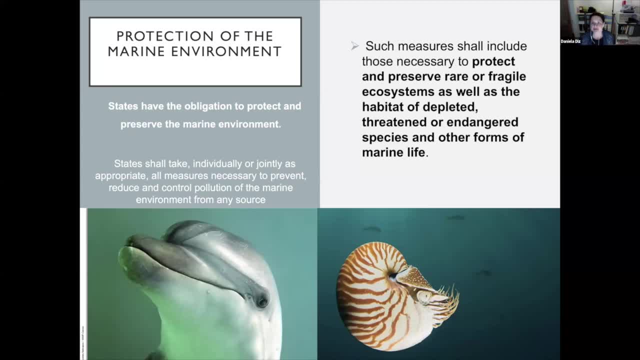 shall include those necessary to protect and preserve rare or fragile ecosystems, as well as the habitat of depleted, threatened or endangered species and other forms of marine life. So coral reefs, mangroves, all of those ecosystems that we have been hearing about today. 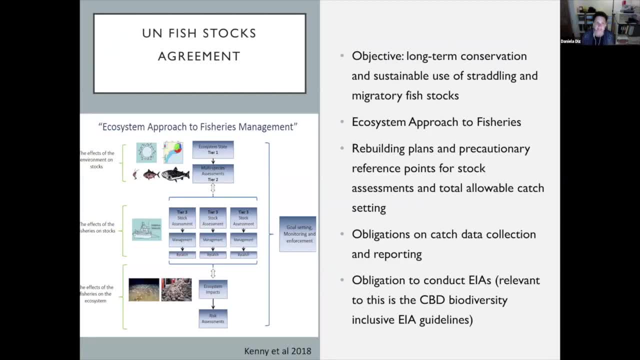 are included in those provisions. Related to that, there is part five and part seven of the Law of the Sea Convention talks about the conservation and sustainable use of living marine resources. So in reference to fisheries, both in the exclusive economic zones in part five, 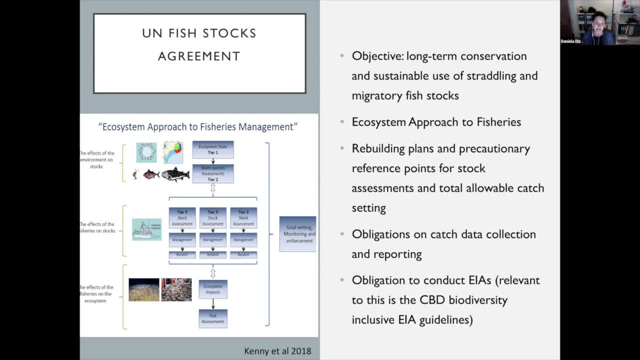 but also in areas beyond national jurisdiction on the high seas in part seven, And to implement some of the provisions contained in part seven related to the high seas, especially around stocks that straddle between areas within and beyond national jurisdiction, a very important implementing agreement. 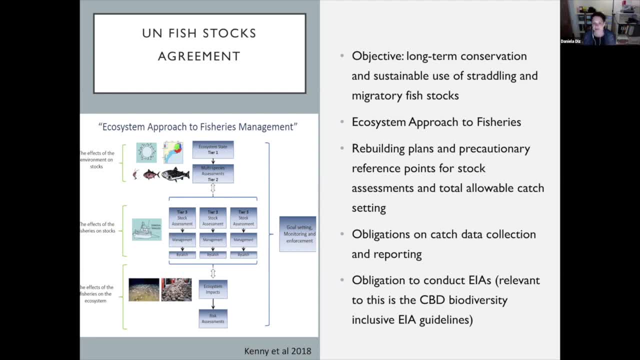 was adopted in 1995.. Which is the UN Fish Stocks Agreement And most of its provisions are applicable to the high seas. but very important provisions- articles five, six and seven- also applies to areas within national jurisdiction. Article five, for example: 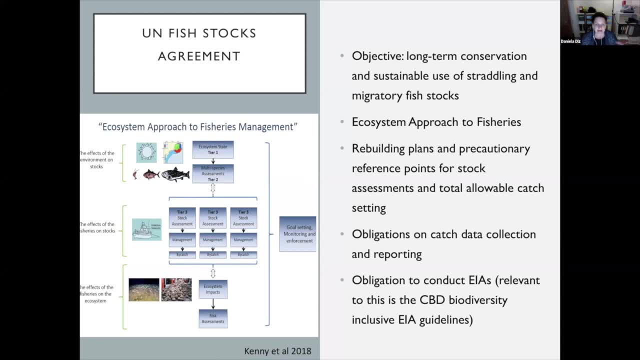 provides a number. It's the general principles that guides the implementation of the agreement, but it also contains very important obligations, And article six is within respect to the precautionary approach to fisheries and how to set precautionary reference points, for example for rebuilding stocks. 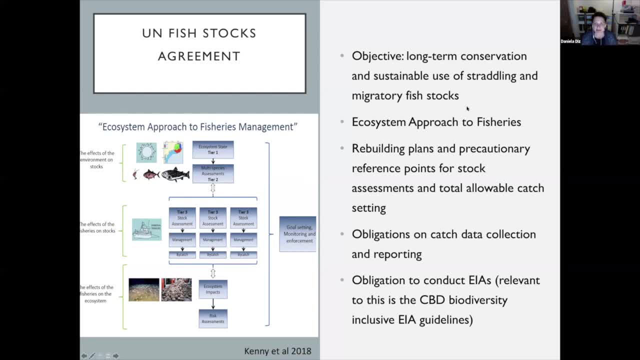 And article seven. it's a little bit contested about compatible measures between areas within and beyond national jurisdiction. But some of the flavor of those provisions first of all, starting with the objective of the conditions: the long-term conservation, sustainable use of straddling. 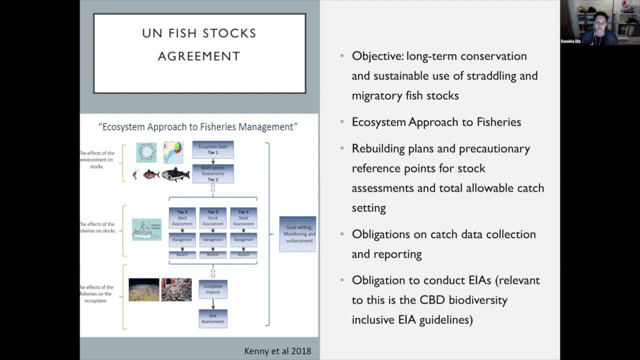 and highly migratory fish stocks. So, moving away from that short-term type of approach that usually humans have, Ecosystem approach to fisheries is embraced through a number of those obligations that I alluded in article five, So you need to when managing fisheries. 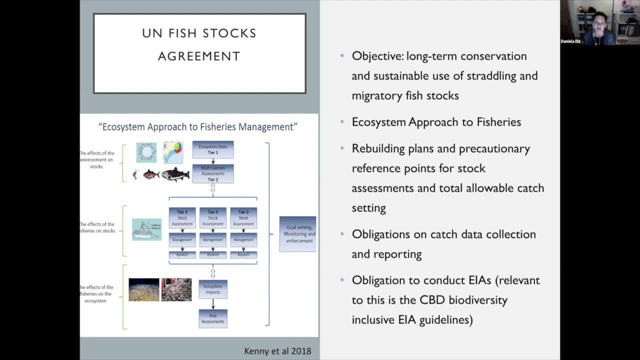 need to take into account the interdependence of stocks. So in this graph here on your left side, you can see that this is just a diagram from Kenny et al, A paper that we published on the ecosystem approach of fisheries that's being put in place. 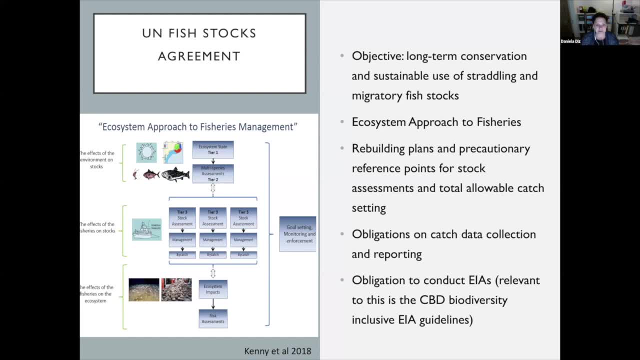 a roadmap that we developed for the Northwest Atlantic Fisheries Organization, whereby those multi-species assessments are a key consideration, and the relationship between those food webs in the system, also in relation to the habitats, because there are a number of vulnerable marine ecosystems that we're going to talk. 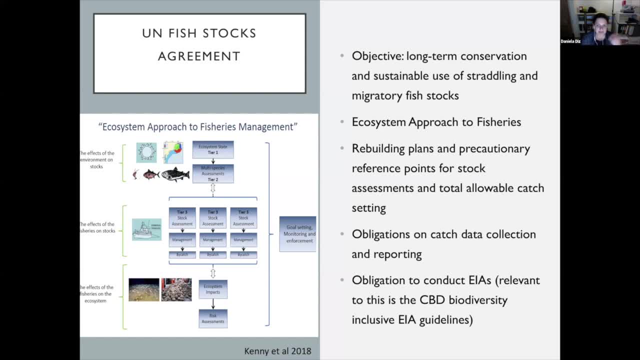 about later today, which are deep water corals, sponges. that also depend on the healthy stocks and the stocks depend on the healthy ecosystem and the ecosystem services that those areas provide Again. so article six of the convention provides for these rebuilding plans. 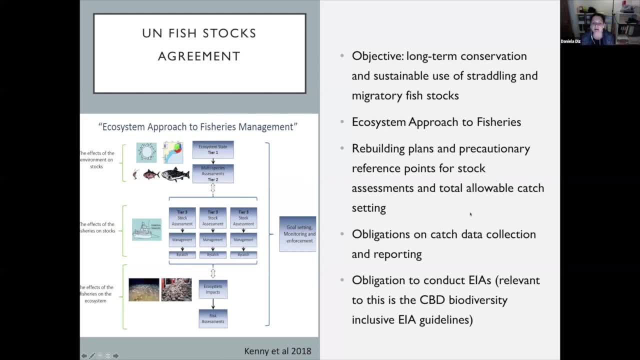 the precautionary reference points, having maximum sustainable yield, for example, as not only the water target, but something that you want to be more precautionary than that, And it's aligned with SDG 14.4,, for example, and also contains a number 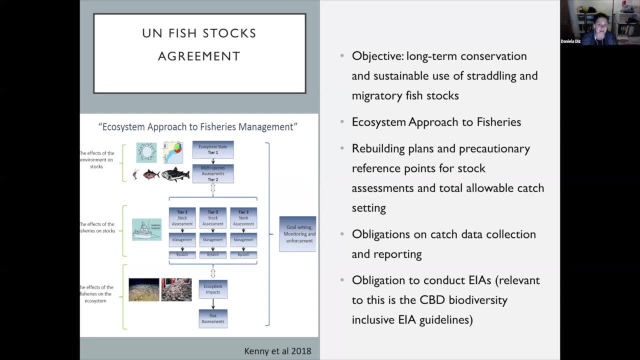 of applications related to catch data collection and reporting, which is also very important to feed into those stock assessments of the most species models that are to be put in place. And in addition to that, another one that I find very important is the obligation to conduct impact assessments. 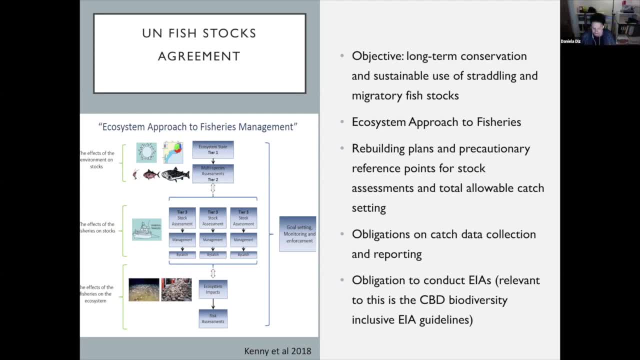 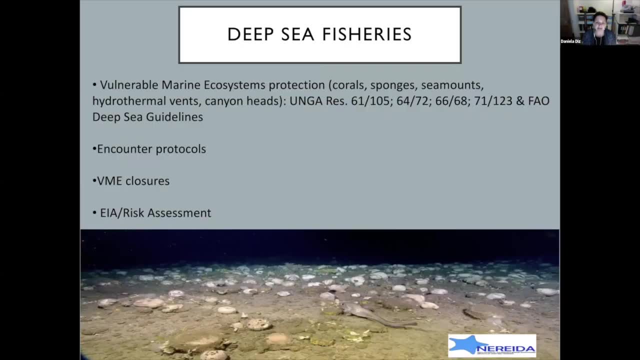 And we'll see more details of what that entails in practice in relation to fisheries, with respect to vulnerable marine ecosystems. So, in relation to deep sea fisheries, something that emerged throughout the years after the fish stocks agreement was negotiated and because of its limited scope in covering shredding- 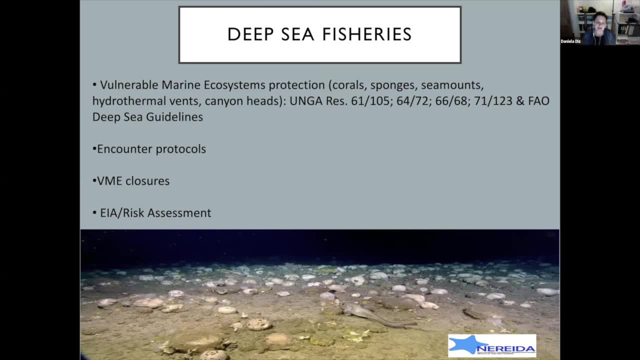 and highly migratory fish stocks. there is a concern about the discrete stocks that only occur in the high seas. There is also concern about those vulnerable marine ecosystems such as cold water, corals, sponges, sea mounts, hydrothermal vents. 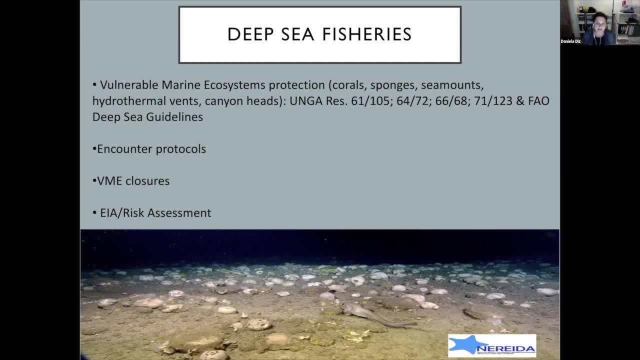 canyon heads that were left somehow not covered by the fish stocks agreement, Even though covered by the law of the sea convention. it wasn't very detailed and they required more specific provisions and guidance around that, And in 2006, the UN General Assembly. 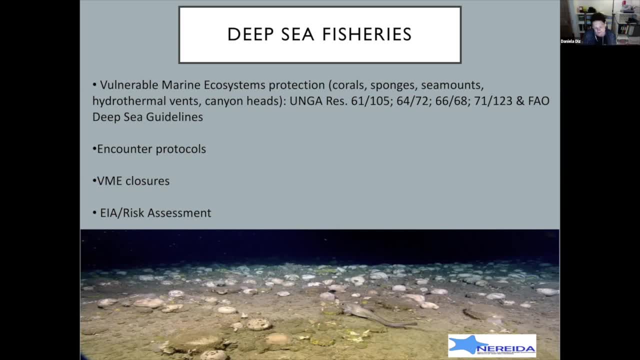 adopted a resolution on sustainable fisheries- the resolution that they adopt every year- but with a specific focus, in its paragraph 83, on vulnerable marine ecosystems, and also requested the FAO, or invited the FAO at the time, to develop guidelines to apply some of those conditions. 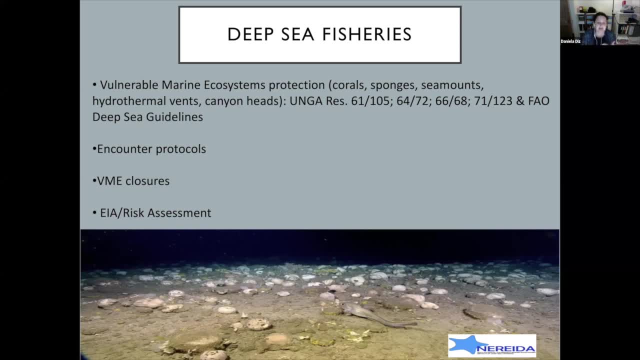 for bottom fishing activities in areas beyond national jurisdiction, But since it was adopted, a number of coastal states have also included some of these requirements into its national legislation with respect to coastal waters, So that's been a success story. I think that provides. 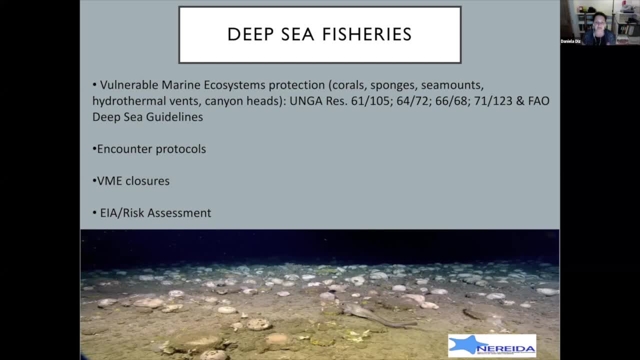 you know some sort of a roadmap for what can be done to protect those ecosystems, And a number of instruments are contained in the FAO guidelines- the deep sea guidelines, for example, encounter protocols- But the most effective so far from literature has been a closure. 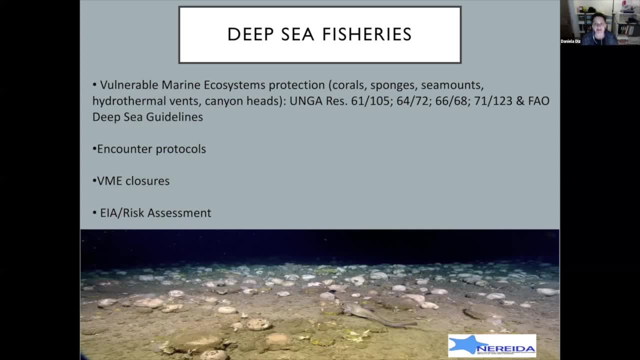 fisheries closures to protect those vulnerable marine ecosystems that, of course, need to be identified, And sometimes you need to because of the you know the location of them, you use habitat suitability models to identify those and you can ground truth eventually with research cruises. 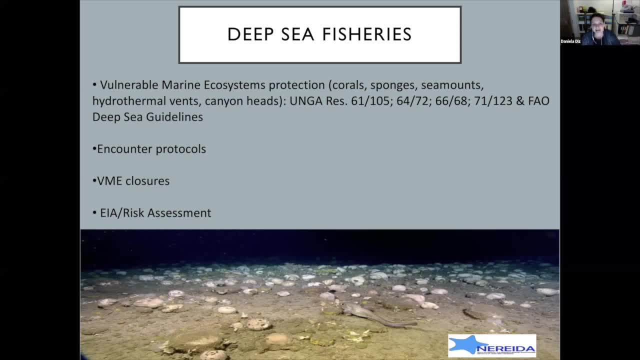 and so on And again. the impact assessment was much more explained under the FAO deep sea fisheries guidelines. It contains criteria for what the environmental impact assessment needs to contain And including risk assessment provisions as well. I'm going a little bit quick. 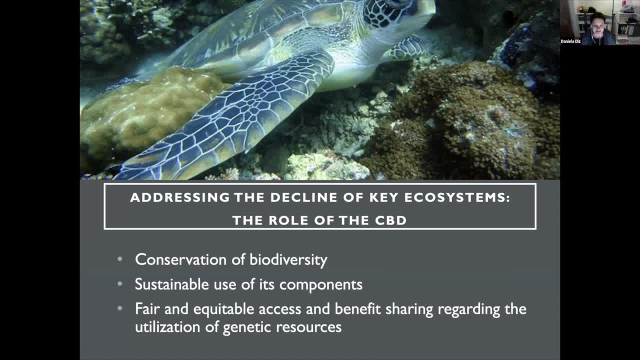 because I know I'm conscious of the time, but I'm happy to answer questions on those specific instruments that I'm alluding to. In terms of CBD, the Convention of Biological Diversity, I'd like to complement, you know what, the law of the sea. 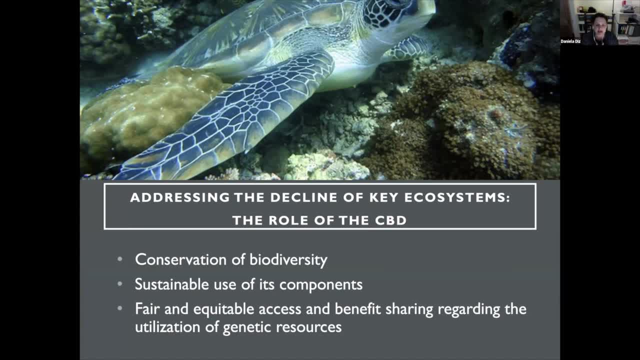 the fish stocks agreement and the deep sea fisheries guidelines, the UNJ resolution, have done with the provisions of the Convention of Biological Diversity, because to address the decline of those key ecosystems that we're talking about here today, the Convention of Biological Diversity is a key instrument. 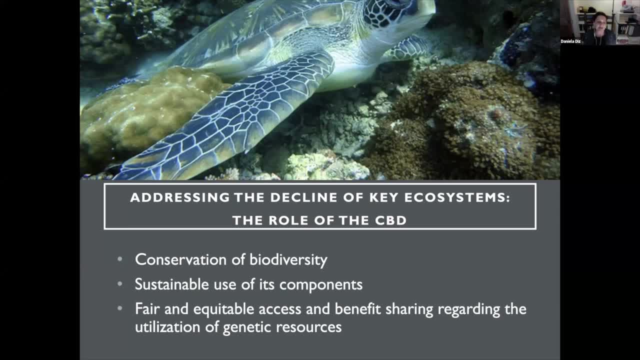 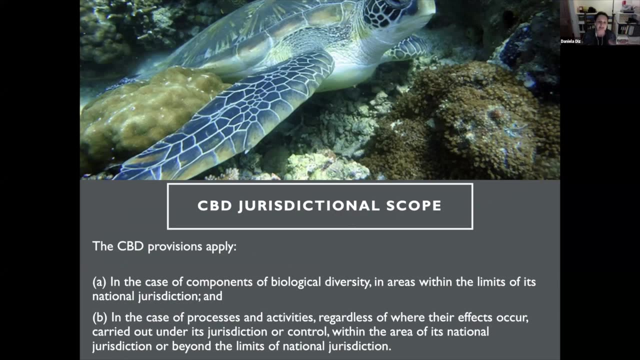 Its objectives are around conservation of biodiversity, the single use of its components, as well as the fair and equitable access and benefit sharing of its genetic resources, But within a jurisdictional scope, that is, you know, it differs from areas within national jurisdiction. 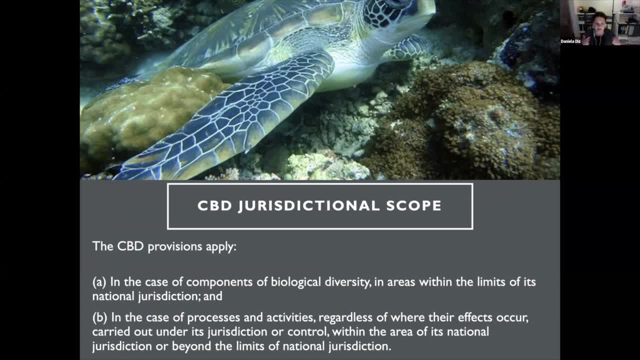 and beyond. So, in terms of with relation to the components of biodiversity itself, the Convention applies to areas within the limits of national jurisdiction, And, in case of processes and activities, the Convention applies in areas within and beyond national jurisdiction. So, for example, 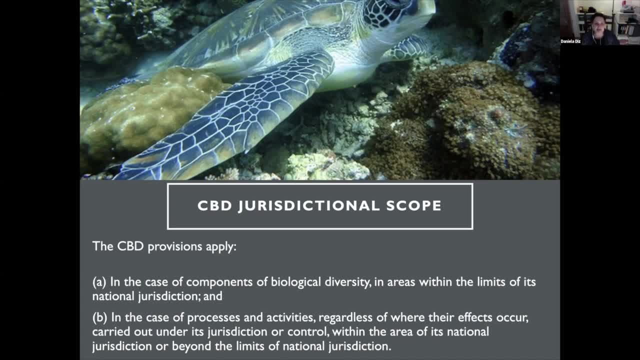 marine genetic resources, that is, marine genetic resources, can be regulated in areas outside national jurisdiction through the CBD And there is a lot of debate many years ago around the possibility of establishment of marine protected areas in areas beyond national jurisdiction, given the limited jurisdictional scope. 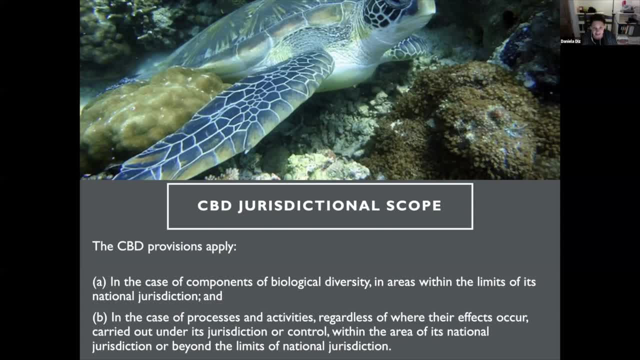 of the Conventions of the Convention, even though it applies to processes and activities that would be regulated by those MPAs. But it was decided that, under the law of the Sea Convention, marine protected areas- that's their home- for being regulated. 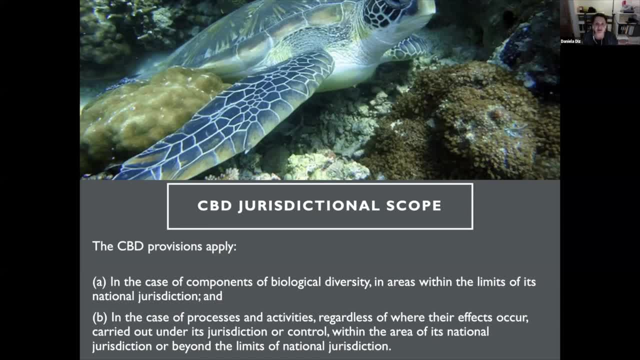 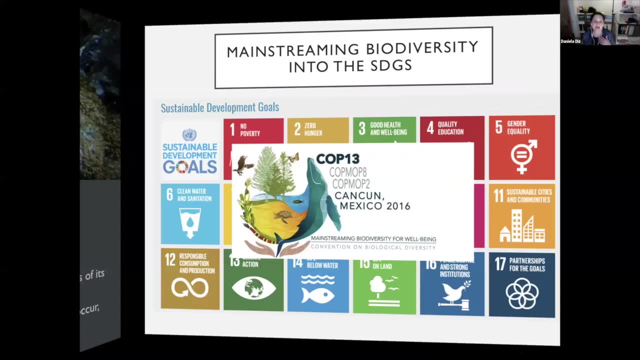 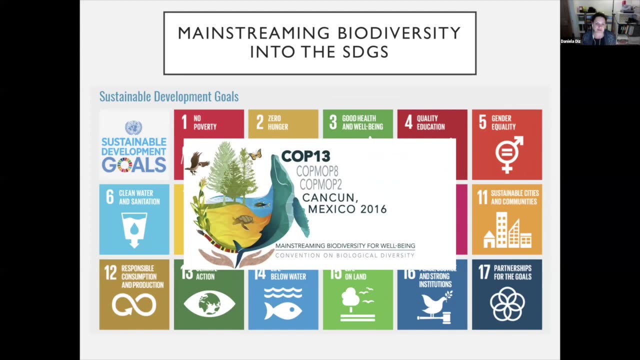 And that was one of the reasons why a new implementing agreement to the law of the Sea Convention is being negotiated at the moment. In 2016,, the CBD COP- its COP conference of the parties 13,- adopted a decision that called for its parties. 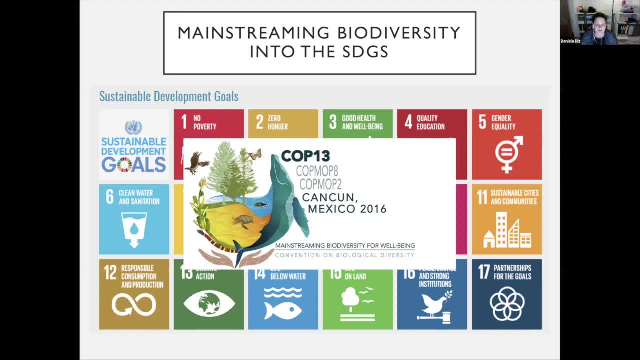 to mainstream biodiversity into the implementation of the SDGs. So it urged parties, when implementing the 2030 Agenda for Sustainable Development, to mainstream biodiversity in the implementation of all the SDGs relevant SDGs, thus promoting linkages between the efforts to implement national biodiversity strategies. 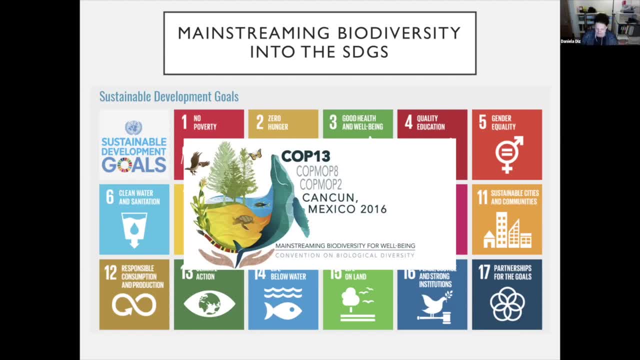 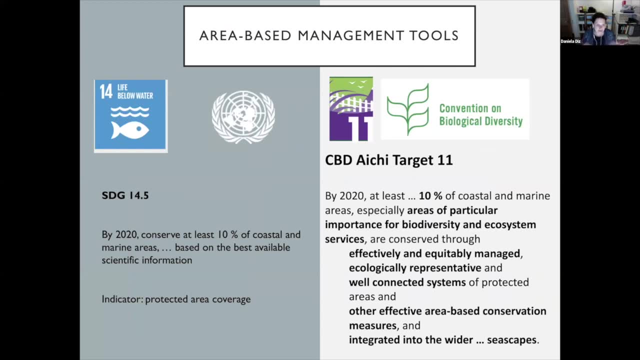 and action plans. So we're going to see some of the examples of how this could be done. So one of the examples. so if we pick SDG 14.5 on protected areas, marine protected areas and IHE Biodiversity Target 11,. 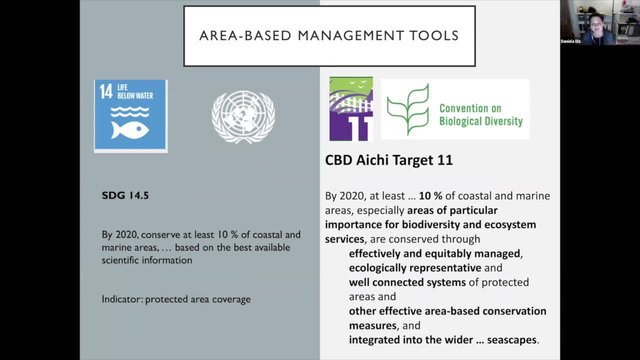 we can see that the IHE Biodiversity Target 11,, which was adopted by the CBD conference of the parties in 2010, and they're expiring the end of this year, is much more detailed. So if you compare, you can think that. 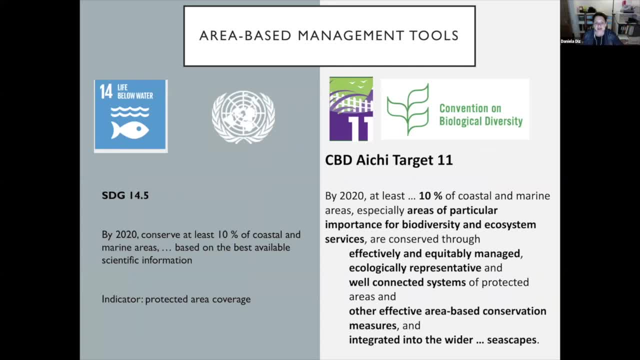 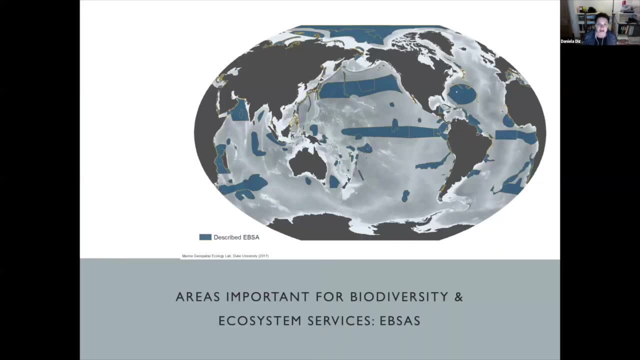 okay, implementing SDG 14 could benefit from using a number of those qualifying elements of the IHE Biodiversity Target 11.. So I'm just going to go through some of those elements. I don't have time for too much detail today. 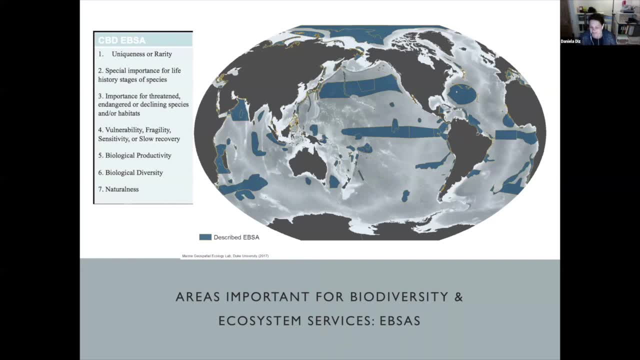 So this is a wonderful map by Pat Halpin from Duke University in the US, And this is just an example of when you look at Target 11, it talks about protecting, conserving biodiversity in areas important for biodiversity and ecosystem services. So what are those areas? 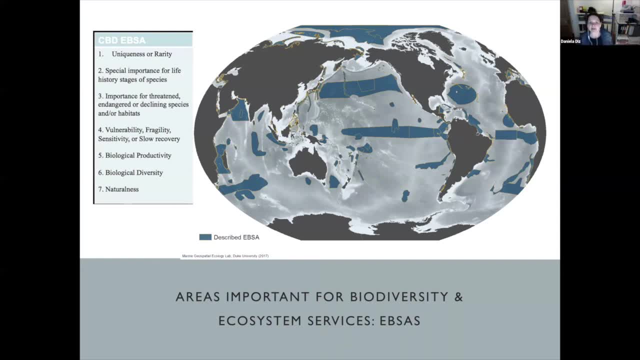 Of course, a number of those habitats that we're talking about here today comprise those areas, But the Convention of Biological Diversity created a process to describe areas that meet the ecological or biologically significant marine areas criteria, which is this one listed on your screen. 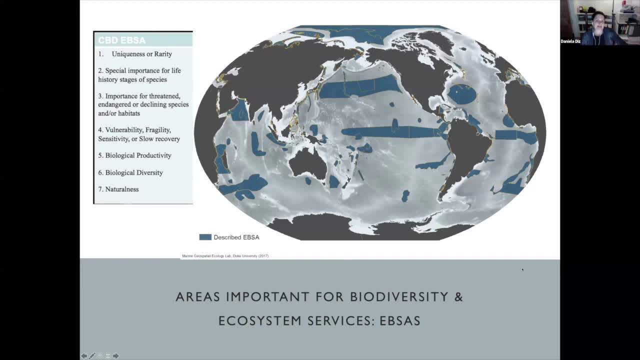 And to meet that criteria you can meet just one of the criterion, but it's very robust mechanism, scientifically and technically robust mechanism that promotes international scientific cooperation to describe those areas, And those areas comprise a number of those ecosystems that we are talking about. 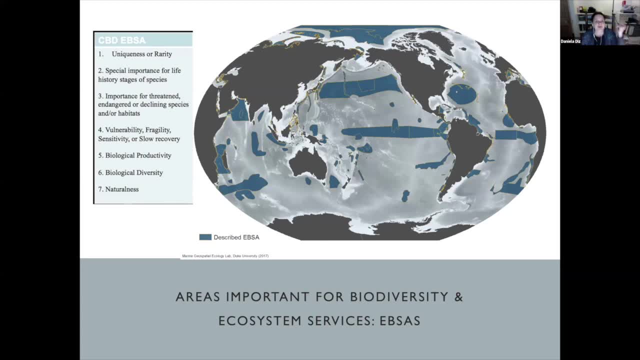 mangroves and coral reefs and deepwater corals, hydrothermal vents, seamounts- a number of them, as well as important habitats, spawning grounds and so on. So it's very the areas are there. There has been 319,. 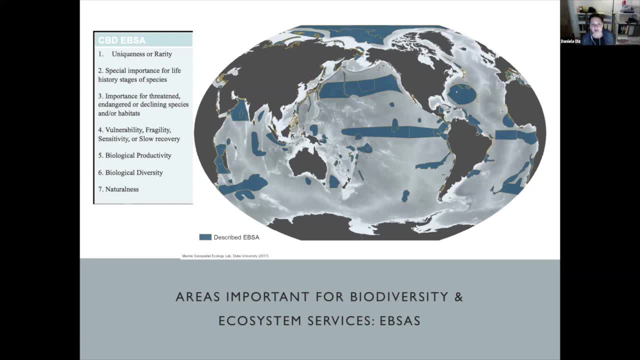 around 319 EBSAs described globally and there are 17 more waiting to be adopted by COP 15.. And when it takes place? So yeah, so the reason why I wanted to show the EBSAs is that they provide some. 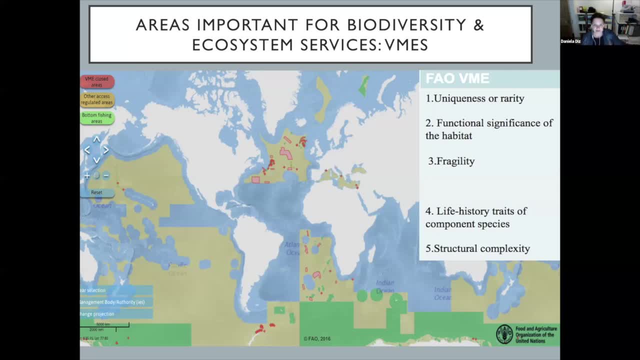 already some baseline information that will be important to monitor in the future in terms of the status of those habitats. The other important areas for biodiversity and ecosystem services are, of course, the vulnerable marine ecosystems that we talked about. FAO has a database and FAO doesn't identify them. 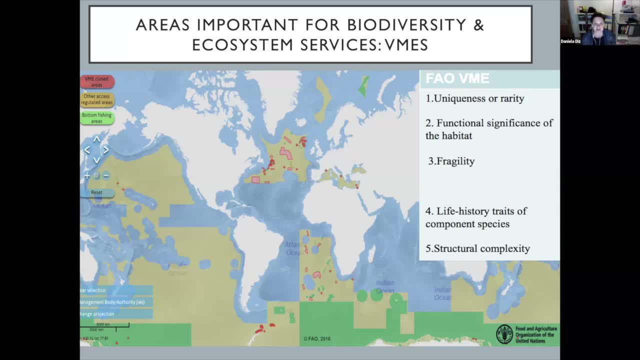 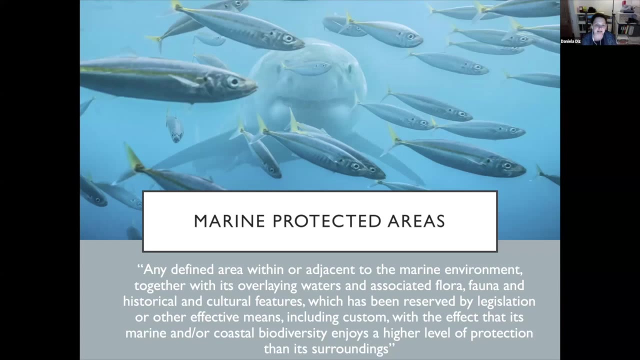 per se, but the regional fisheries management organizations are tasked with that, with that function, and they provide information to FAO to display in their database. So another element of that IH Target 11 is marine protected areas And of course we know there is a definition. 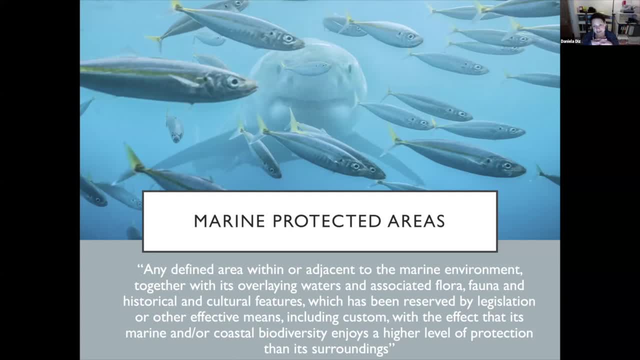 of marine protected areas contained in the by the UCN that was incorporated through a COP this year, a footnote in the COP decision of the Convention on Biological Diversity, talking about the area needs to be identified, needs to be in marine environment. 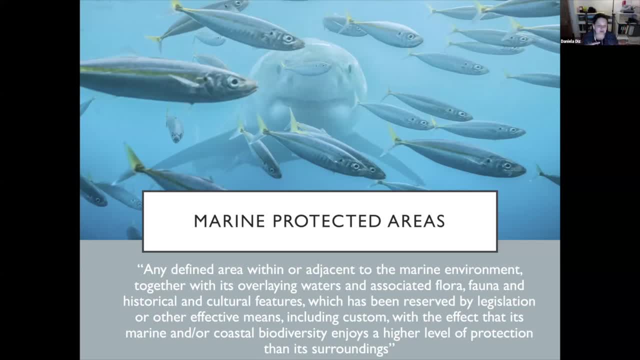 It could have flora, fauna, historical, cultural features, but it needs to be reserved by legislation or other effective means so that effective management needs to be in place through that and also management plans. Of course, there is a whole series of different series of guidance. 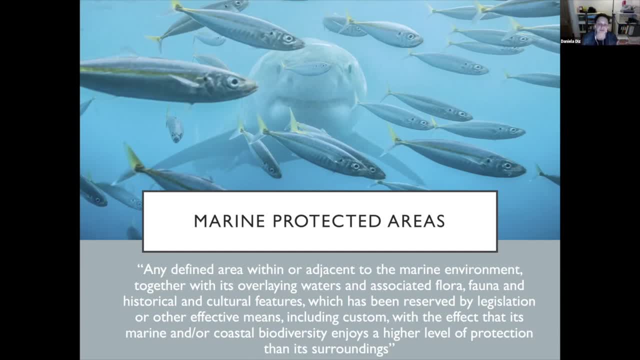 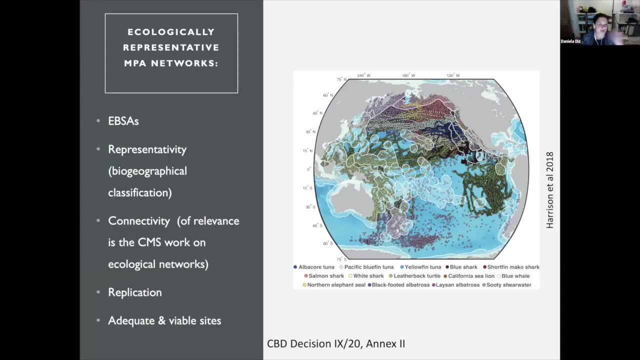 on how to create and to establish and to monitor marine protected areas effectively, And we don't, you know, and CBG also developed guidance around the other components of the IH Target, which is the need for those MPAs to be ecologically representative. 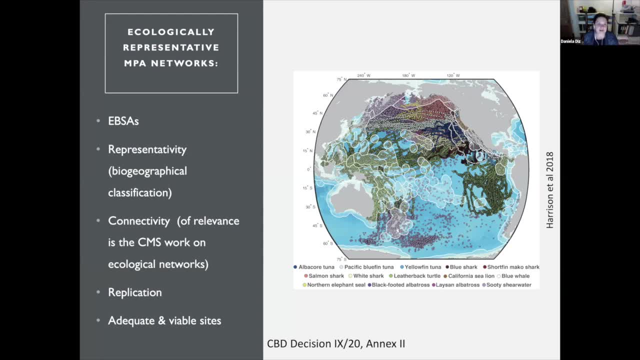 and part of this network of MPAs And ecologically representative MPA networks have been provided and guidance has been provided through COP decision back in 2009 by the CBG. So EBSAs are there, but of course, not all EBSAs need to become MPAs. 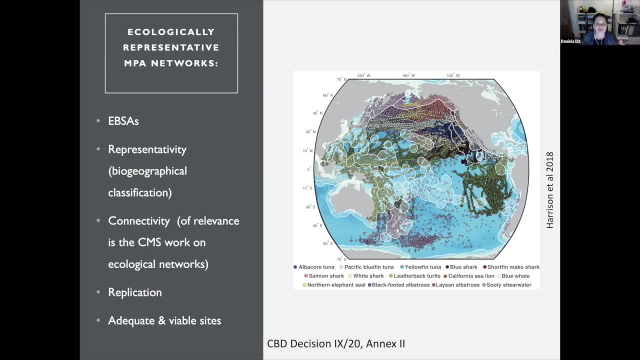 In fact EBSAs are not a management tool, Just to clarify also. there are just scientific and technical information on the importance of that area for biodiversity And of course then managers and government can utilize that information to apply to management tools. 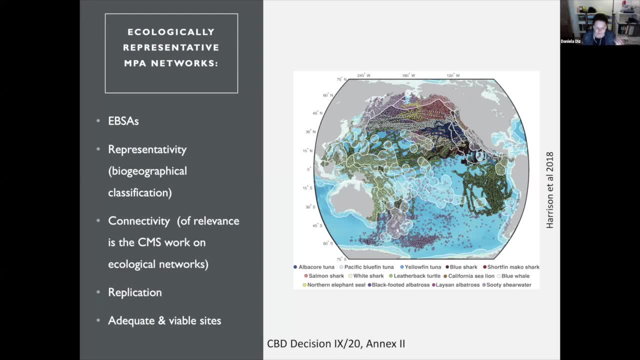 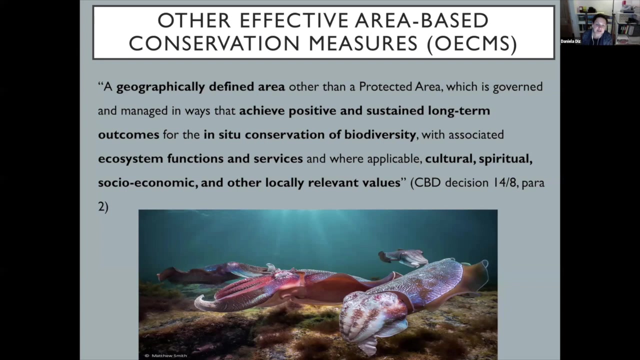 but MPAs could be one of the tools that they decide to use those EBSAs And in addition to that, for network representativity and connectivity and replication and adequate and viable sites through the size of them is very important. Other effective area-based conservation measures: 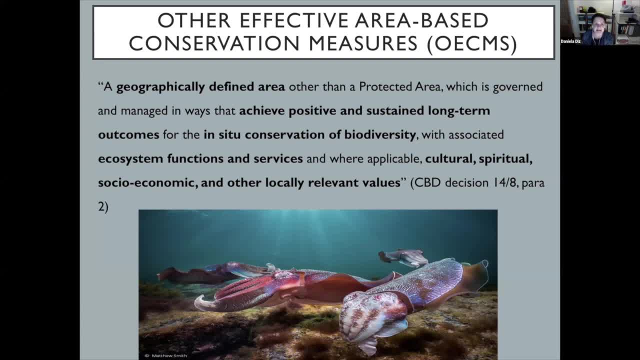 that is also part of that IH Target, which biodiversity target 11- and will probably be part also of the post 2020 biodiversity process that we're gonna talk about in a minute- has been defined more recently in the last COP as a geographically defined area. 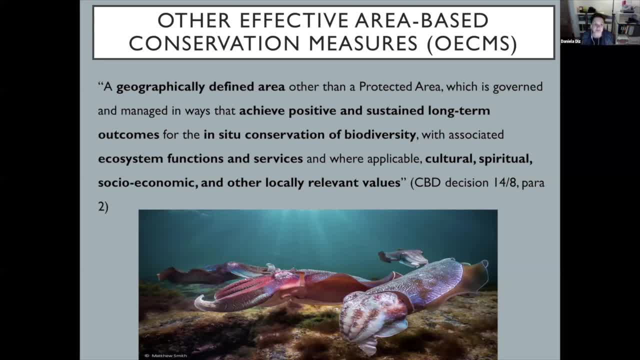 So it needs to be other than a protected area which is governed and managed in ways that achieve positive and sustained long-term outcomes for the in situ conservation of biodiversity, with associated ecosystem functions and services, and more applicable cultural, spiritual, socioeconomic and other locally relevant values. 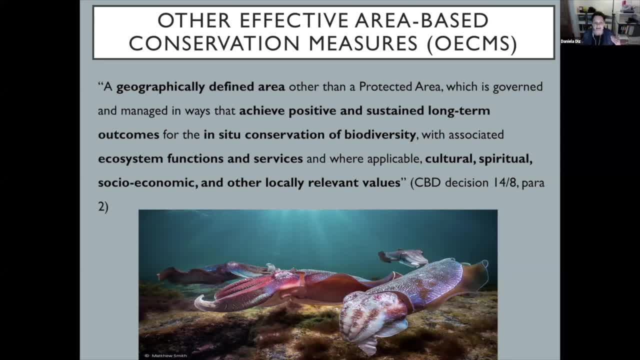 So I find it interesting because while the MPAs need to have a conservation objective, the OECMs they don't need to have a conservation objective, but they need to have a conservation, biodiversity conservation- outcome. So in the way, it's very robust. 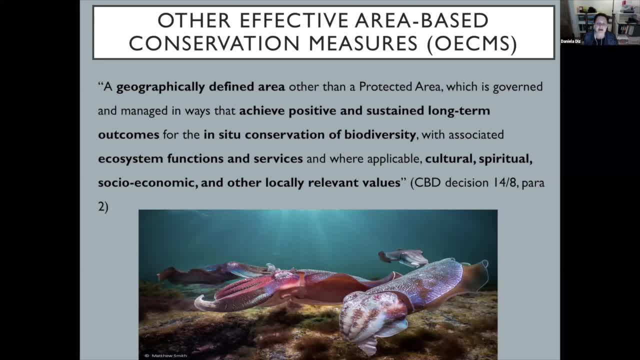 and also criteria for the application of this, of this tool has been developed and adopted by the same decision, CBD decision 14 slash eight. So it's important because some one of the elements that they also highlight in the criteria is the ability to handle multiple threats. 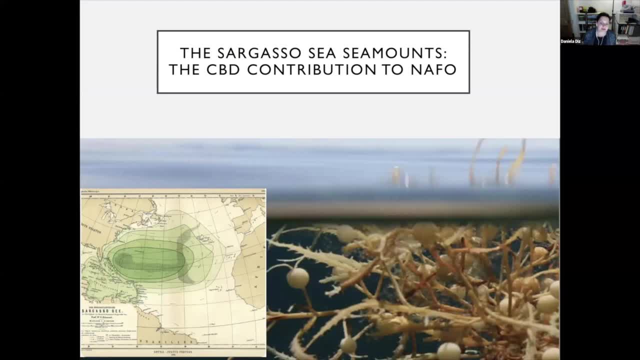 So just to illustrate a little bit what I consider that could be a candidate OECM and bringing those different tools together, just to provide a quick example of: to me a success story has been how two seamounts have been protected at seamounts. 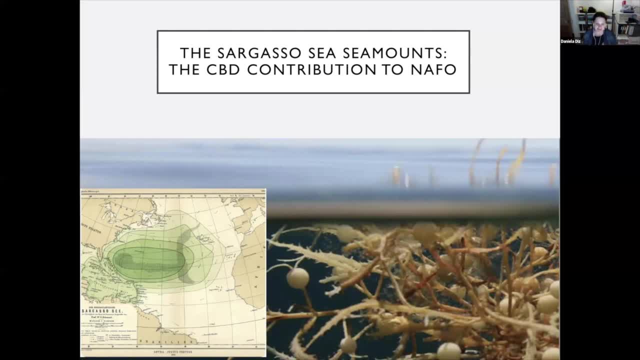 that are part of the Sargasso Sea EBSA that was described became the object of conservation and management measures through a regional fisheries management organization In well, it's been a while, but after the Sargasso Sea was described as an EBSA through the CBD, 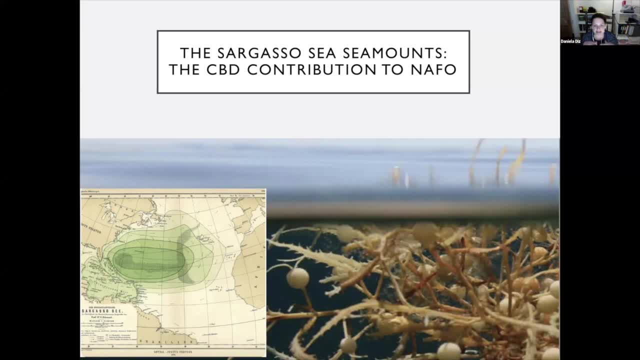 two contracting parties to the Northwest Atlantic Fisheries Organization requested its scientific commission, scientific council, to assess the impacts of their activities, of the fishing activities that they conducted on that EBSA. Initially it was, you know, thought that because the Sargasso Sea is quite pelagic. 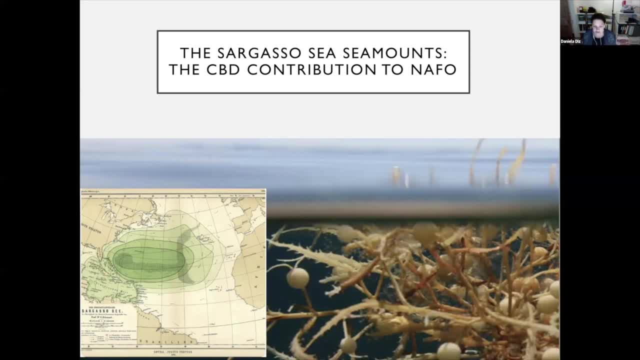 and it didn't include- well, it was thought that it didn't include- the benthic features. Initially. it was almost, you know, disregarded as well. there is no impact. But after looking further, the scientific council saw that in the description of the EBSA. 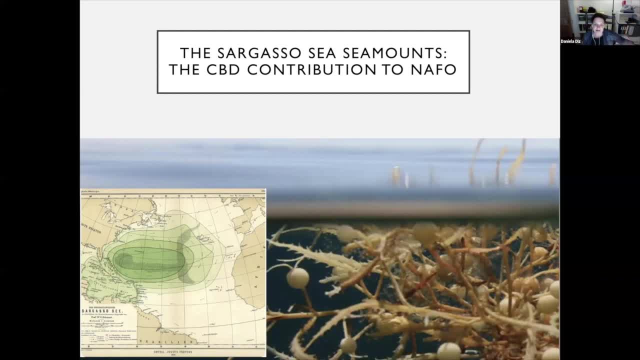 two seamounts, the cornerized seamounts and the New England seamounts, not the entire range but the areas beyond national jurisdiction of the United States. So the areas on the high seas in the ABAJ was included in the EBSA description. 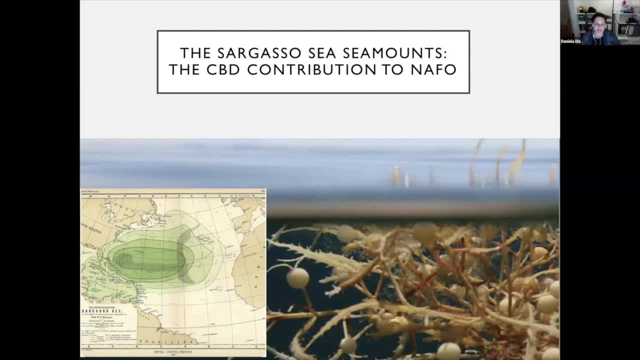 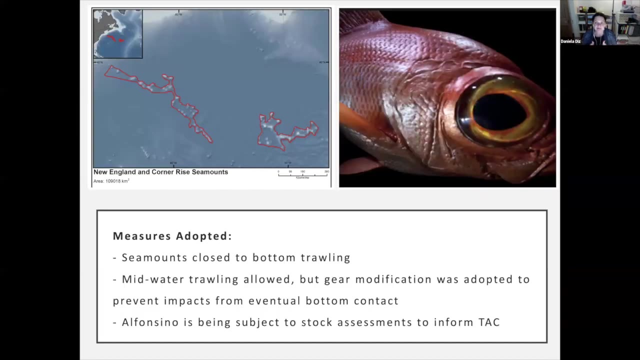 including the Alfonsino species. That's part of object of fishery that was taking place in those seamounts. So a number of efforts were put in place by the scientists who developed guidance for how to conduct that fishery more sustainably and measures were adopted eventually.